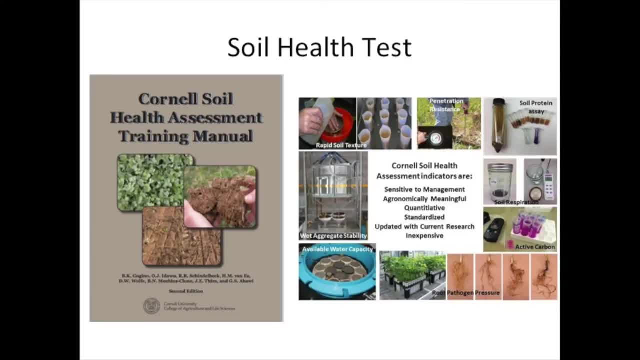 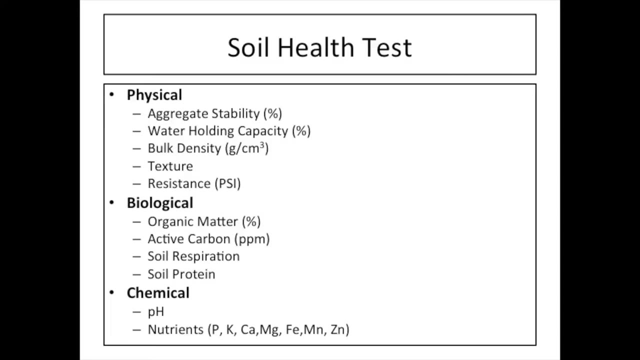 And what this test does is- it's a set of standards, like I just described, that, when integrated together, kind of gives you a holistic picture of your soils. And this test is just like any other soil test that you could send a sample into and have results sent back to you. 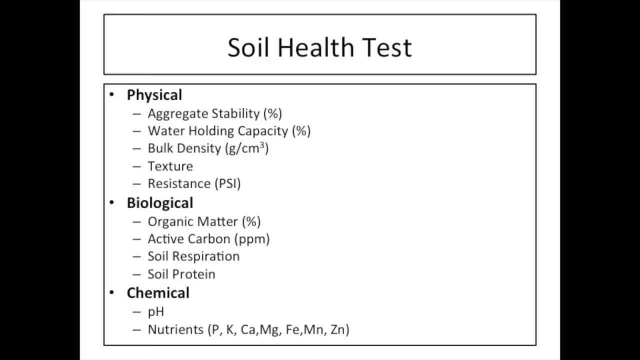 But different from maybe strictly a biological or a chemical test. we cover a bunch of different aspects. So when we talk about physical, we're mostly referring to is aggregate stability, water holding capacity, bulk density, texture and resistance, or compaction is a synonym. 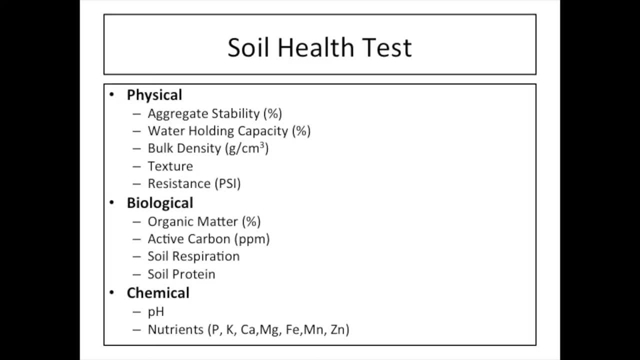 When we're talking about biological, mostly, what we're thinking about is the soil microorganisms, And this is going to cover organic matter, active carbon, which is just a fraction of total organic matter, which is just a fraction of the amount we get from soil matters. 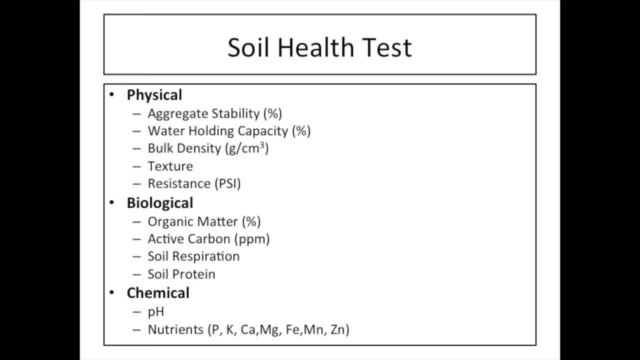 So we are actually going to cover a ton of organic matter, which is just a fraction of total organic matter, and that is hormones, as well as soil, respiration and protein. And also, when we're looking at chemicals, we're gonna be primarily looking at pH. 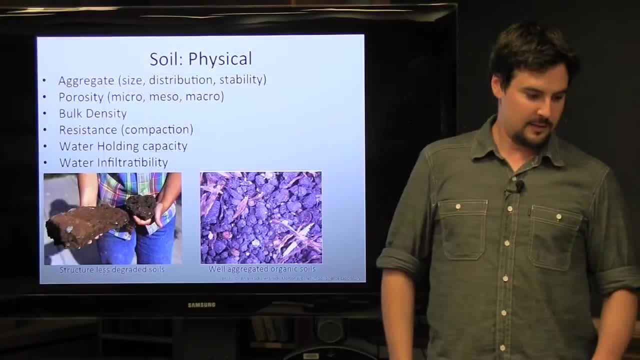 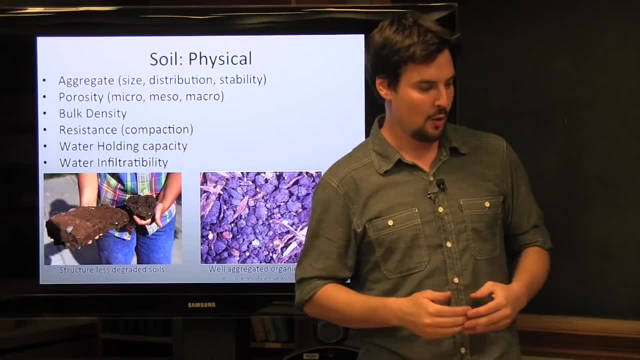 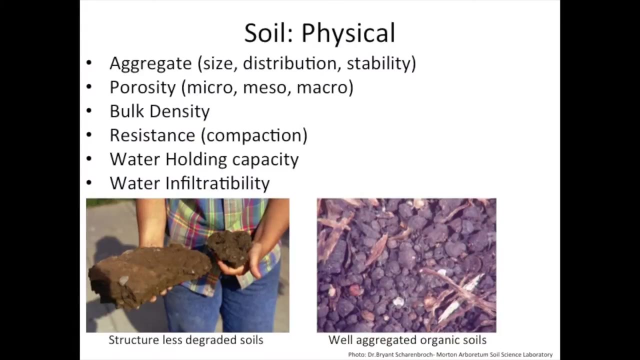 and as well as our macro and micro nutrients. So, to go through this talk, today I'm gonna introduce soil health. we're talking about looking at specific indicators within specific aspects of our soil. So when we're talking about the physical aspects, we're 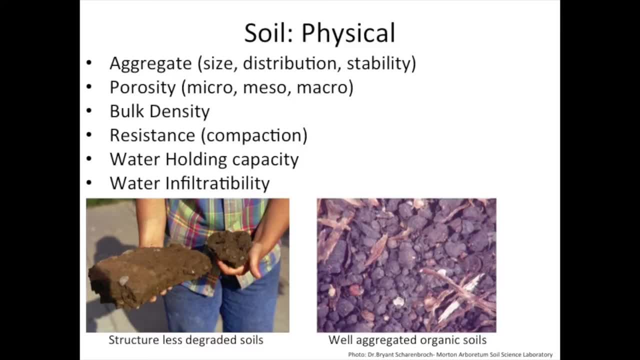 mainly talking about aggregates, so the actual particles that conglomerate together in your soils, and so size and distribution, as well as stability- how easy they break apart. We're talking about porosity- how easy, how much air is in your soil and how much space is between your aggregates and your 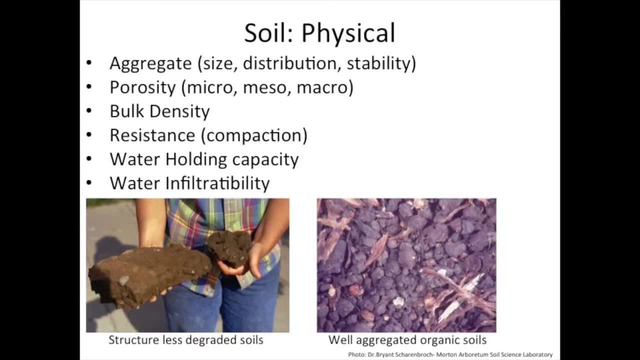 structure. We're talking about bulk density, which specifically refers to weight by volume and is a very good indicator for compaction, which can oftentimes be a large inhibiting factor in our soils or at least our abilities to be able to grow landscape plants directly in them. Resistance as well. 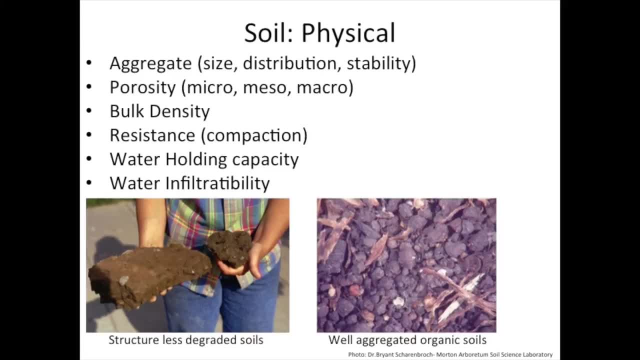 which is a measure, another measure of compaction which we can use: a penetrometer, a very easy field tool to use to get a quick sense of what our compaction looks like And as well as water holding capacity, how much water is in the soil that is. 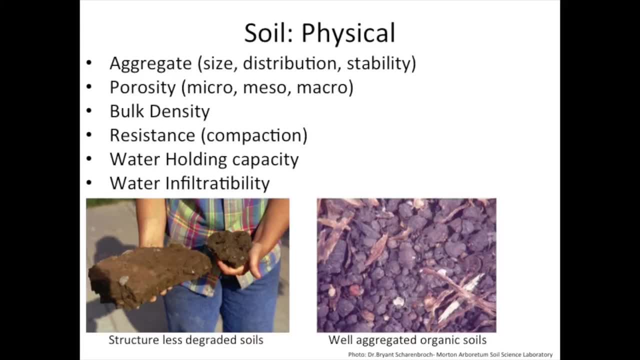 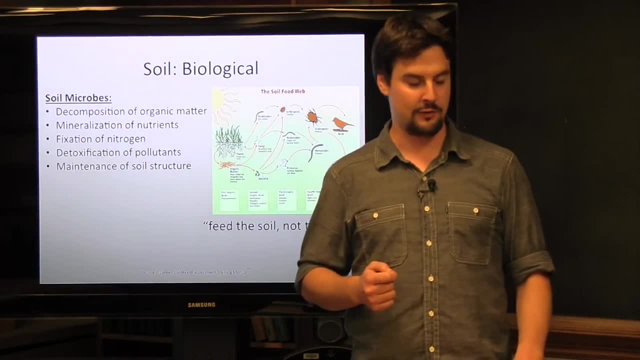 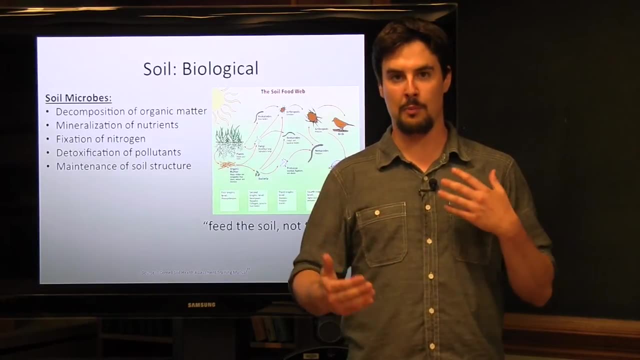 available for your plants and water infiltratability, so how quickly water can move into your soil. When we move on to the soil, biological factors mostly, what we're talking about is the microorganisms that we find in our soil, And these play a very important role and have been an area of research that has 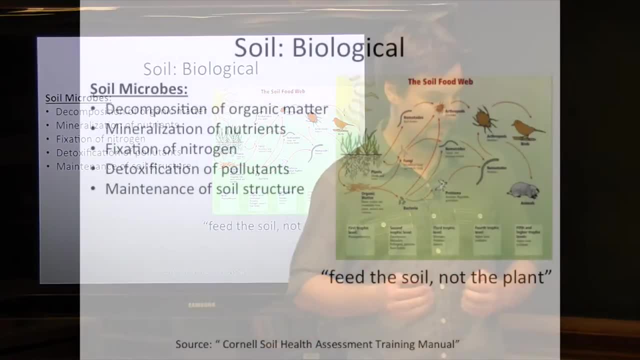 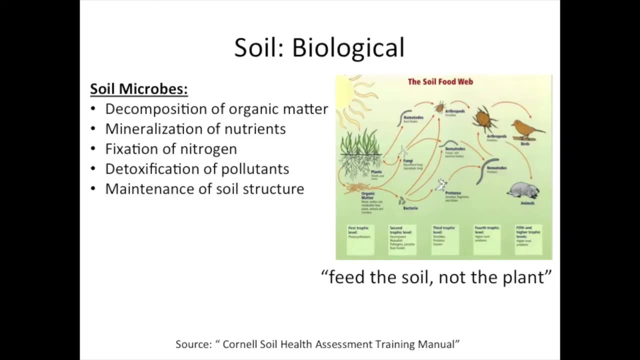 been gaining more traction and more focus in recent history. But a lot of what the biological factors tend to focus on is the ability for microorganisms to mediate soil nutrients turning over in the soil, as well as them contributing to organic matter. Also, the fixation of nitrogen is a common 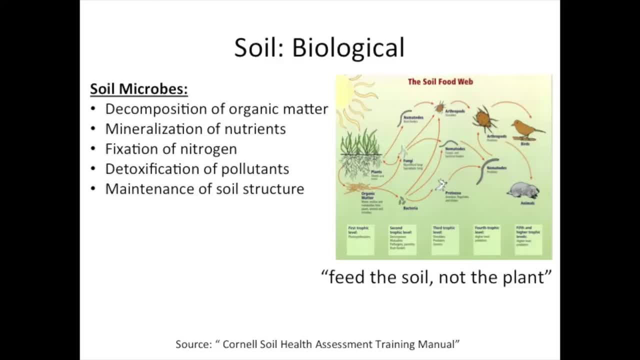 benefit we see from soil biological factors, as well as detoxification of pollutants and the maintenance of soil structure. And, as we're kind of thinking about soil biology, the kind of mantra that I like to go with or that you tend to hear frequently, is that what we're thinking? 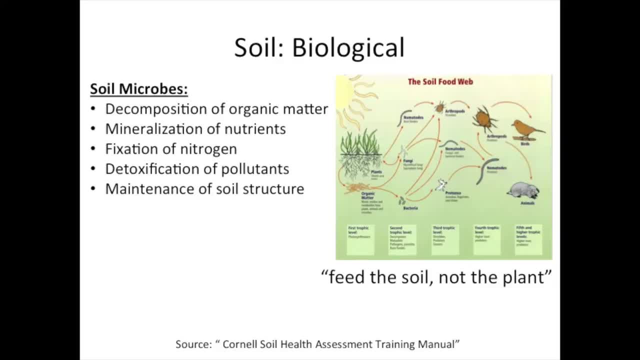 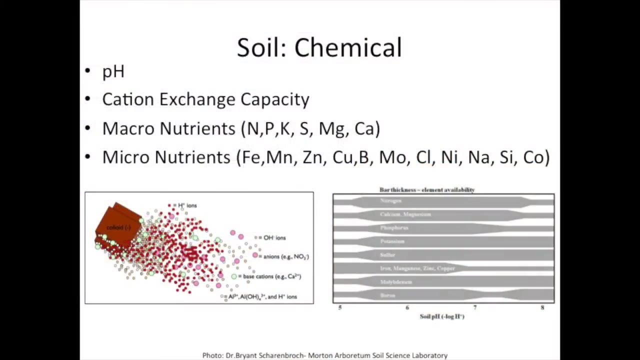 about specifically with nutrients is feeding the soil not necessarily feeding the plants specifically- And we'll get into this a little bit more as we continue our talk today- And the third major area is soil chemical, And soil chemical refers to the specific micro and macro nutrients that are required for plants to be able to grow in. 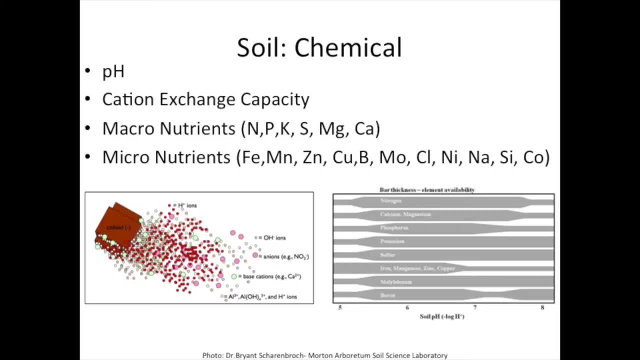 thrive in a given environment, as well as the specific pH, which is also going to be a limiting factor for what kind of plants you can use in that soil, and then cation exchange capacity, which specifically refers to the ability for soil to hold on to nutrients and then allow them to be plant available So that 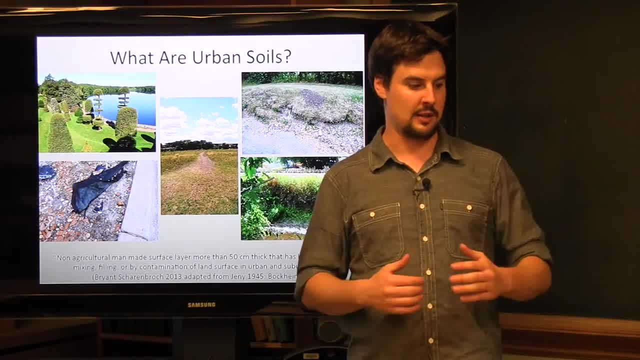 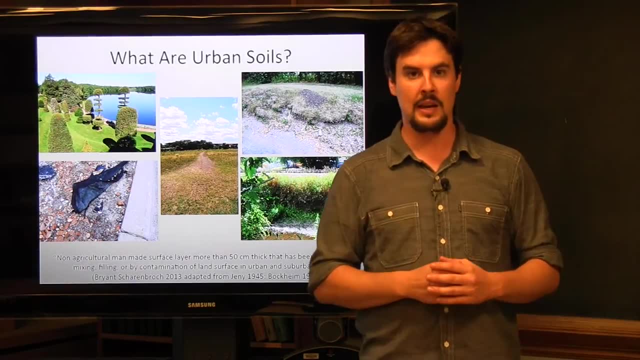 was a quick summary of what soil health is and the general concepts that go with it, and I'm going to move now into talking a little bit about urban soils and remediation. And if you're unfamiliar with the concept of urban soils, what we're talking about when we're talking about urban soils are soils that are. 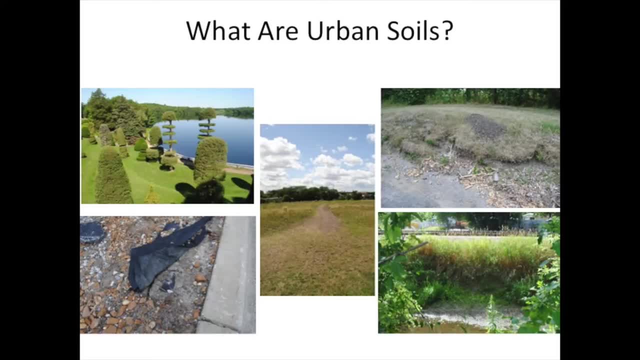 non-agricultural, not necessarily naturally forming or not naturally forming, and in one way or another, are influenced by human impacts and development. So a definition that I like to use is non-agricultural man-made surface layer more than 50 centimeters. 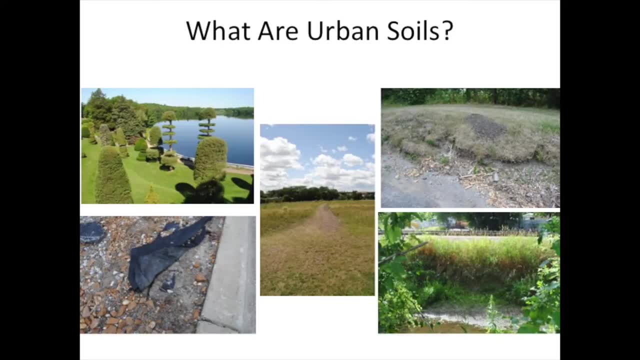 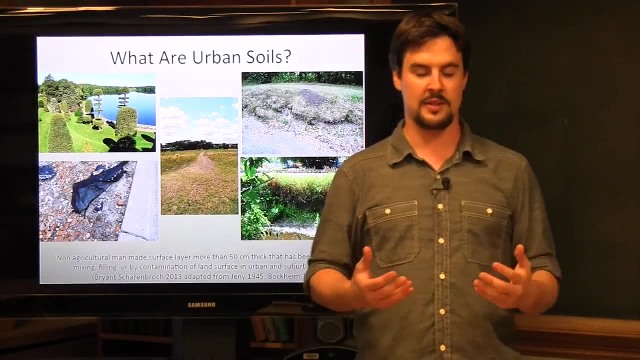 thick that has been produced by a mixing, filling or contamination of land service in urban and suburban areas. So when we talk about urban soils, what this can really refer to is it could refer to parks, it could refer to botanic gardens. 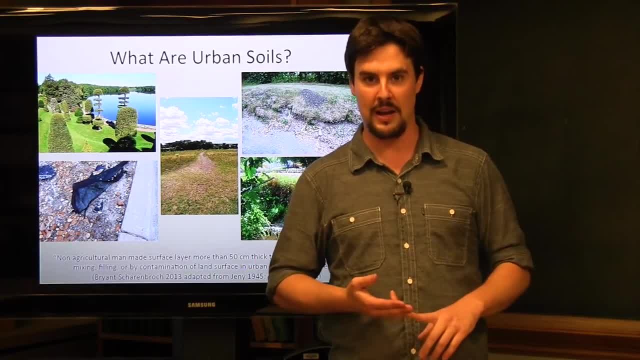 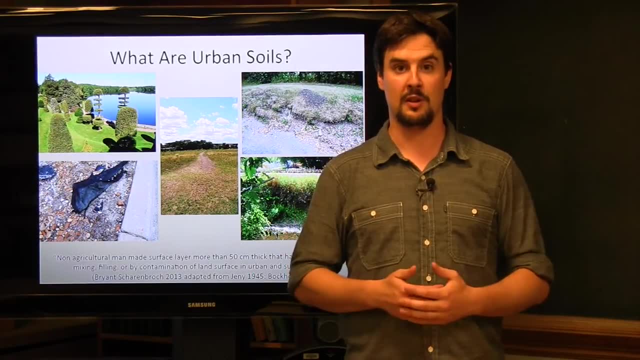 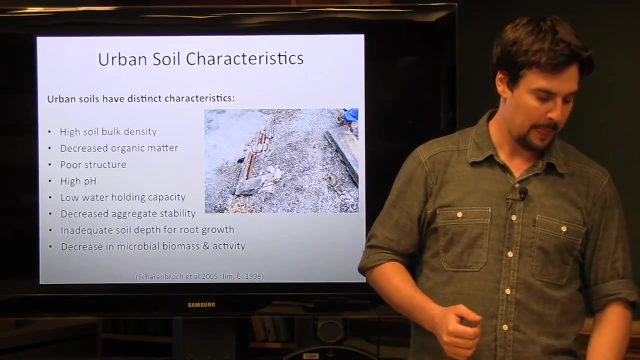 could refer to right-of-ways on highways, could be talking about urban, like city cores, or even suburban, just like people's yards. so soils that in one way or another are influenced by human activity, and the reason why we define urban soils in the 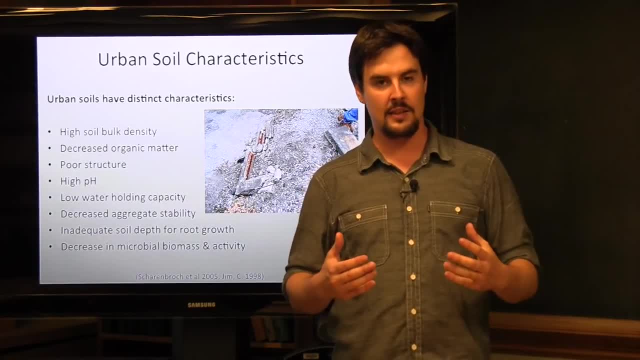 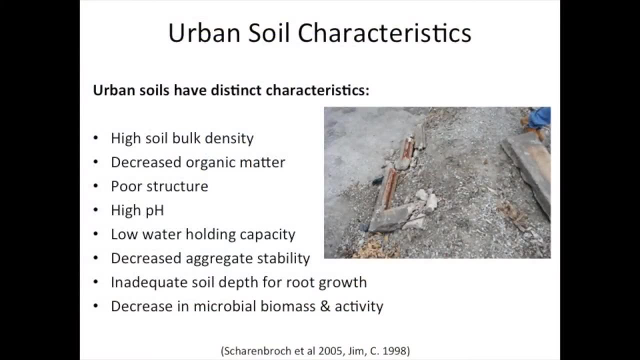 first place is because there's a number of set characteristics that we tend to find in our urban soil systems, and these characteristics typically tend to have adverse effects on the landscape plants that we wish to put in those landscapes. so what we tend to find in an urban system is high soil bulk density. 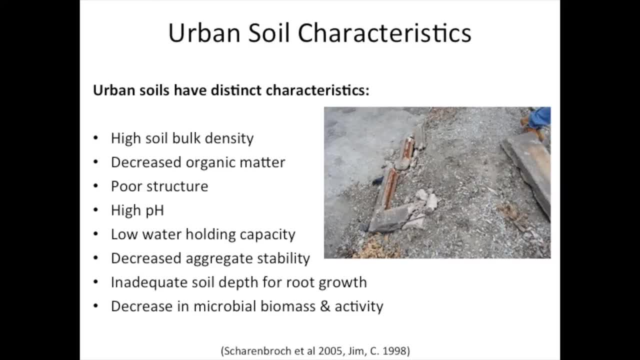 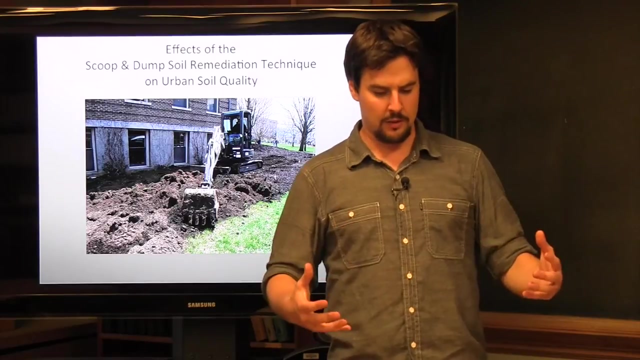 decreases in organic matter, poor structure, high pH, low water holding capacity, a decrease in aggregate stability, inadequate depth for for roots to be able to proliferate in the soil, and as well as a decrease in microbial biomass and activity. so here at Cornell we were trying to find a way to define urban soil density and we found that. 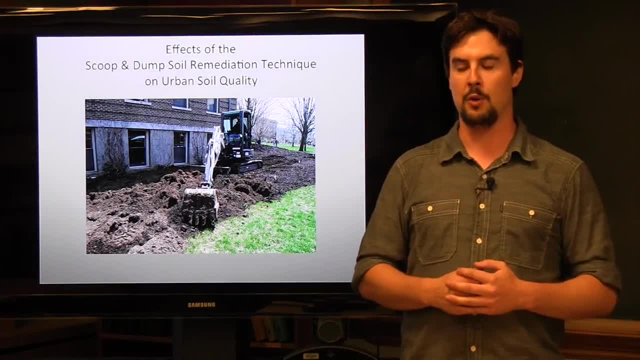 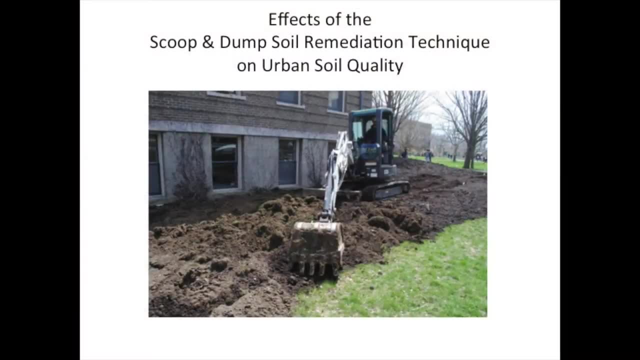 we were trying to think of ways of how to kind of proactively deal with with urban soils and some of the challenges that we tend to see with them. so in the urban horticultural Institute, in Neenah Basics lab, we focused on developing this technique, known as the scoop and dump technique, of soil remediation and the 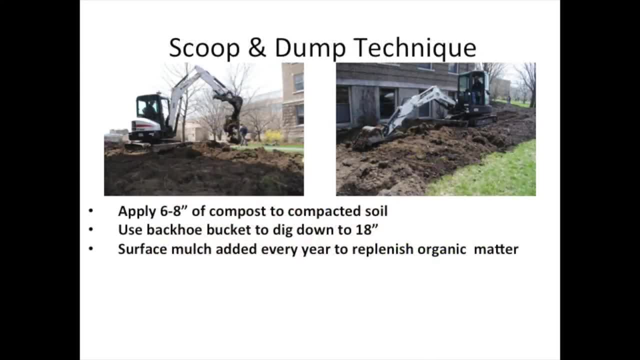 practice is is relatively straightforward. what you do is you come in with compost into compacted and disturbed urban soil site and you apply that compost at a rate of six to eight inches on the top of the soil surface, and then you come in with either a backhoe or mini excavator, or you can even do it with shovels. and what? 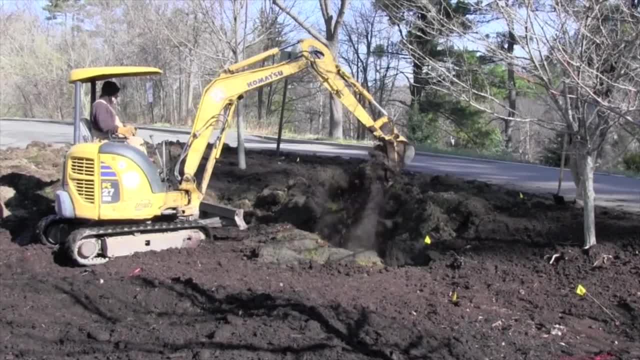 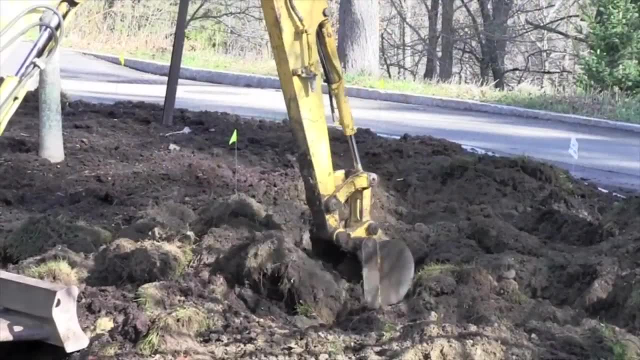 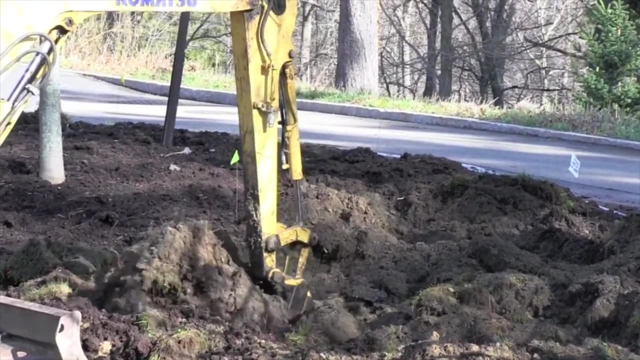 you do is you physically use your backhoe to fracture and scoop down to the soil, reaching into the subsoil. you lift it up that soil, shake it and drop it, and what this does is it creates a heterogeneous mixture of compost and soil, and after that point you can either roto till it or just iron rake it over. 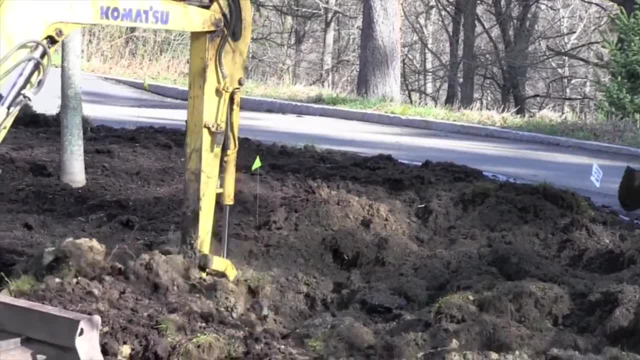 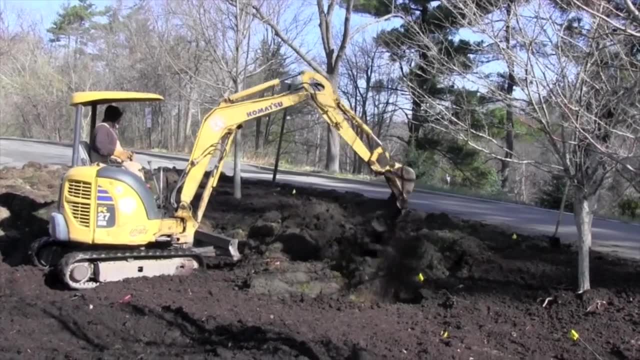 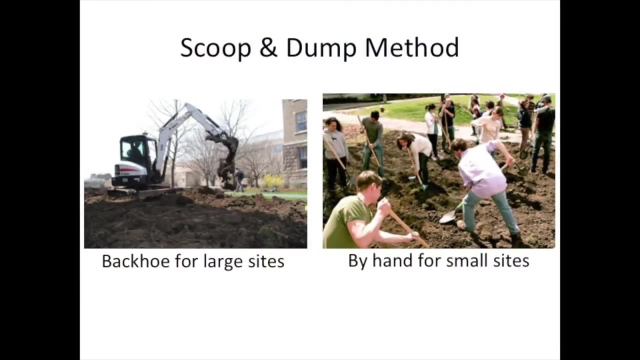 to create a smooth planting surface and then you apply mulch and what you have after this, at this point, is a planting bed that is now you can directly put plants into. mostly we've used this with shrubs and tree species, and this is just a few pictures of what it kind of looks like. you can you do this technique? 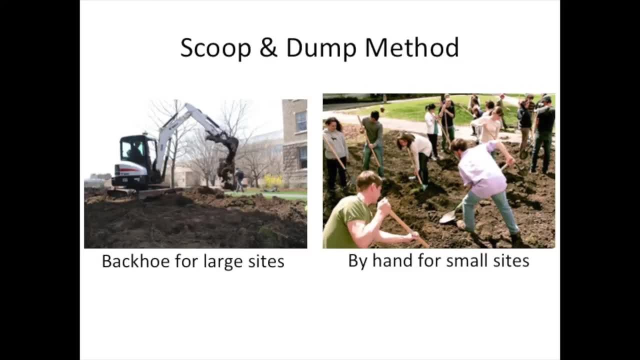 either by using a backhoe or by using- if you have a lot of help, you can do it by shovels, but it's a very simple technique that you can do with a backhoe or by using- if you have a lot of help, you can do it by shovels, but so 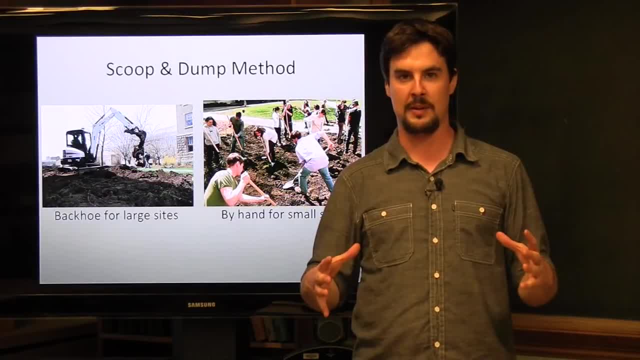 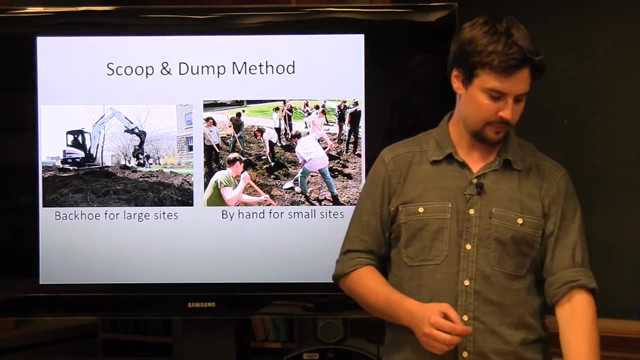 successful and you can use it to either create large planting beds or very small planting beds, if you want to just put one tree in or just a few shrubs, or if you want to renovate a large area. and on the Cornell campus we've been doing 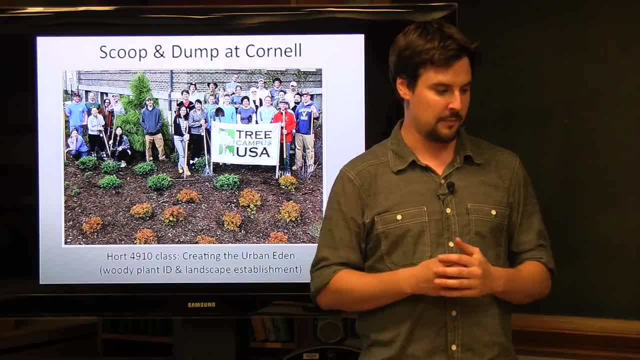 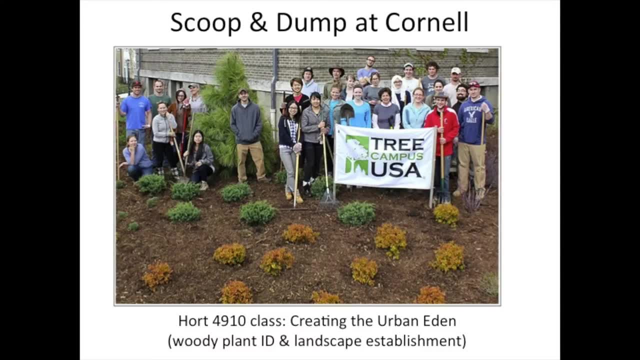 the scoop and dump practice for the last 14 years now as a part of Neenah Basics creating the urban Eden woody plant ID and landscape establishment class. every year the class will create a new garden on campus and and when they design this garden and then eventually install it, they've been 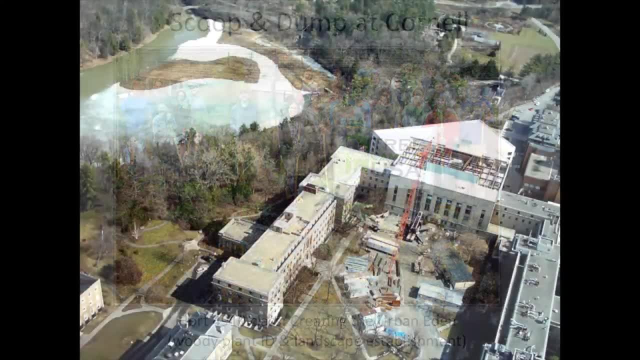 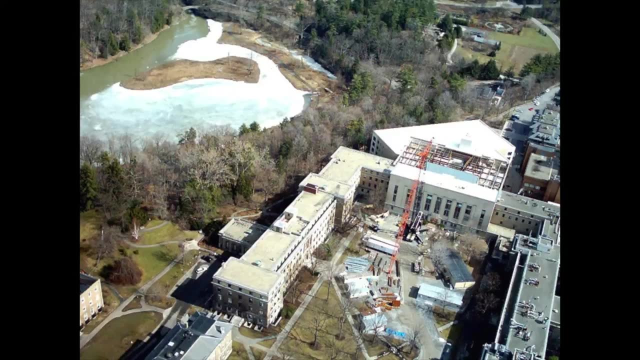 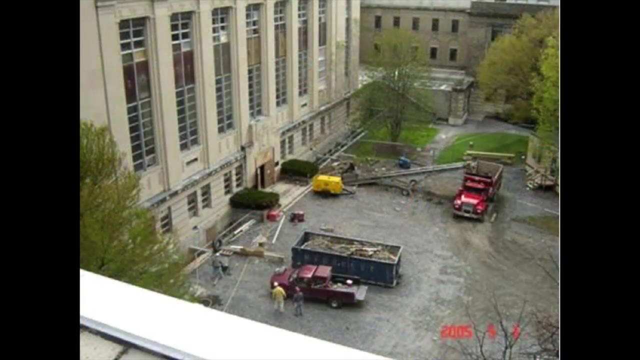 using the scoop and dump technique, and we've used this technique in in a various number of places. this is a picture of outside of man library when we were doing construction a few years ago, and you can see that the the landing area right in front of the building. here's another angle of that, of what a 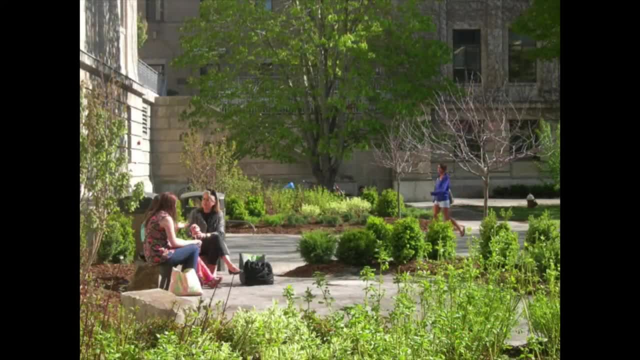 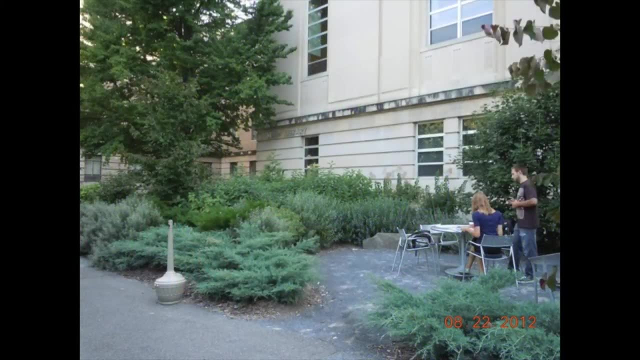 construction landscape looked like, and this is what the landscape looks like today. where we've come in. we've used the scoop and dump technique to remediate the soil and now it is a place where it went from highly compacted and impacted from construction to a place we're. 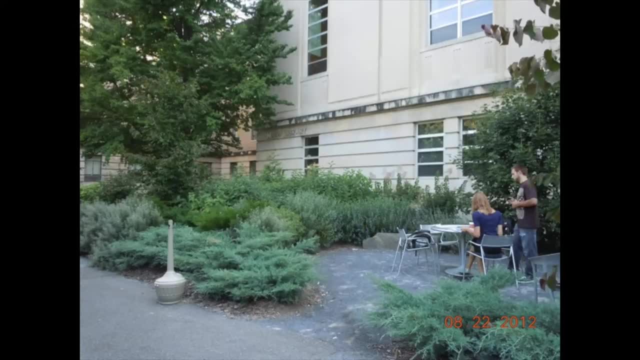 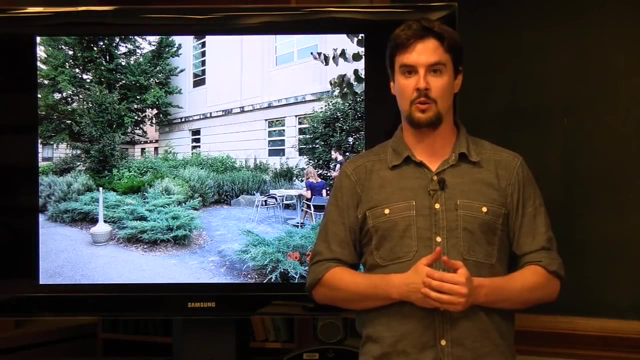 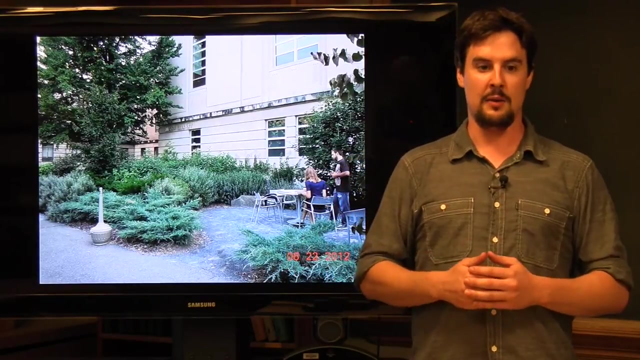 having our landscape plants thrive and survive. so we wanted to kind of look at the scoop and dump technique and learn a few things about it. we want to find how changes in soil quality, based on soil health, had changed in response to doing the scoop and dump technique. and we also wanted to look at this to see how, since 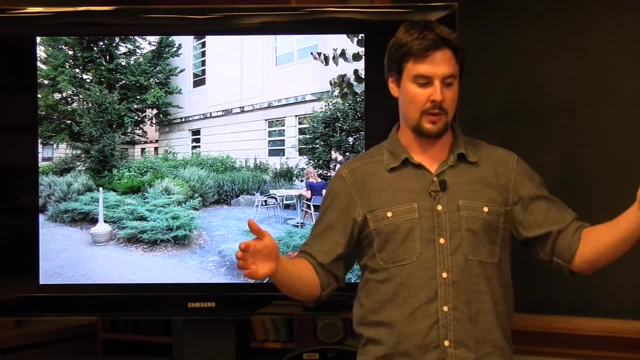 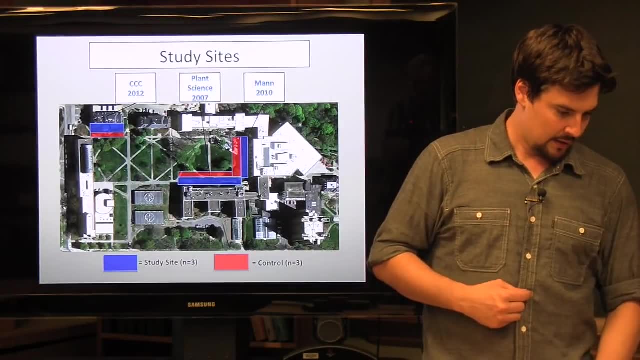 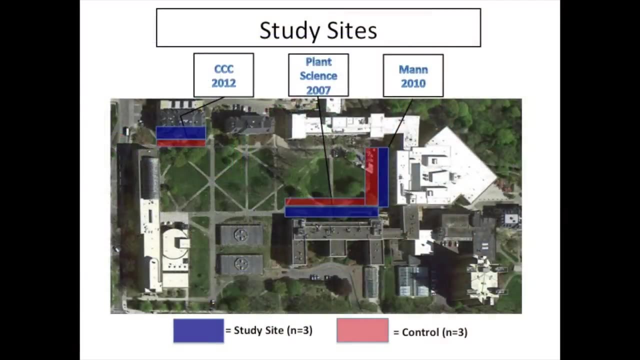 we had 12 years worth of gardens, or 14 years. at this point we were able to see over time also how changes were made. so we selected three sites where this technique had been applied and three sites directly adjacent to it. this way we could do a control type experiment where we had plants growing, or so we had. 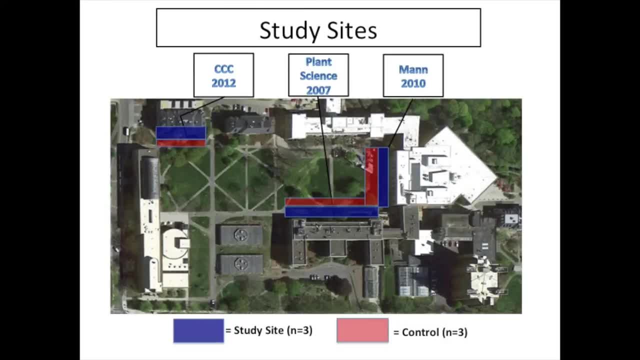 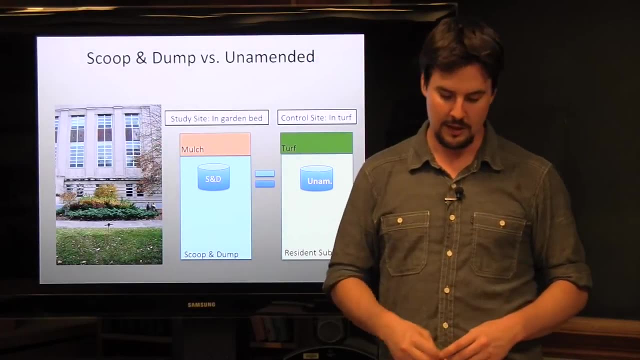 soils that had been developed by the scoop and dump technique. and then we had areas they were close by that had received similar impacts but had not gone through the same remediation. so we went to these sites and we took soil cores. we took three of them that were about this size and we took these cores. 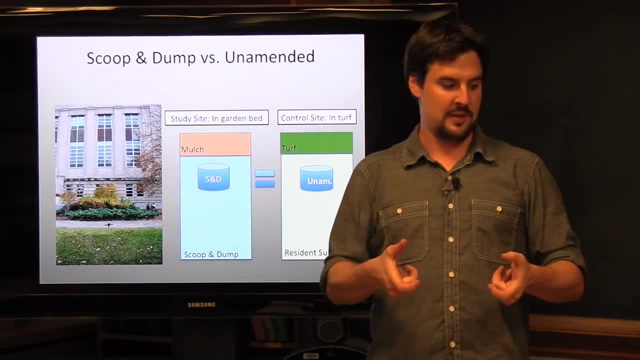 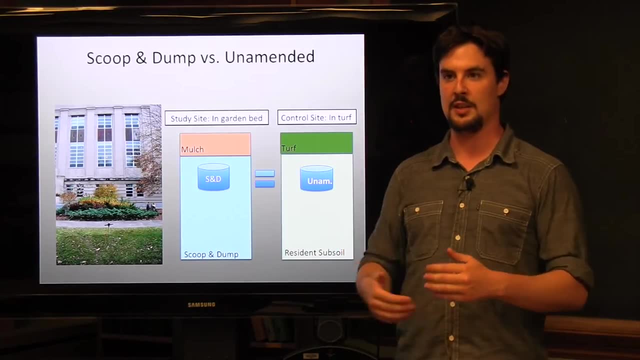 and we extracted samples directly from our scoop and dump soils and then an equal depth. we also took them in our unamended and we went just below our mulch level because, as I mentioned, when you do the scoop and dump technique, you add mulch every year and these samples you extract from the Kingdom. so you 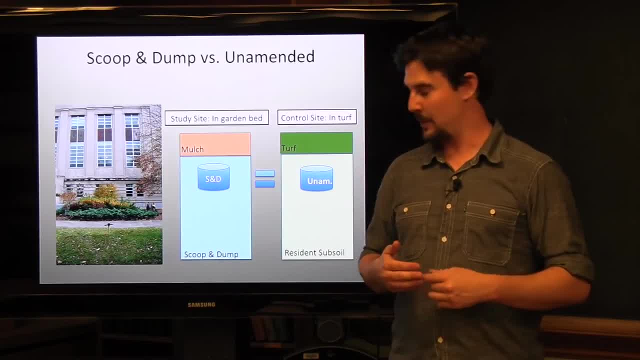 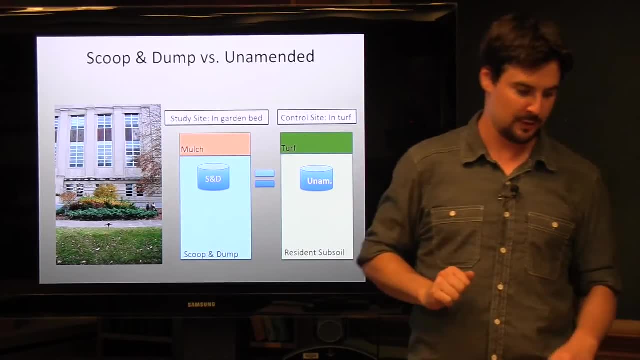 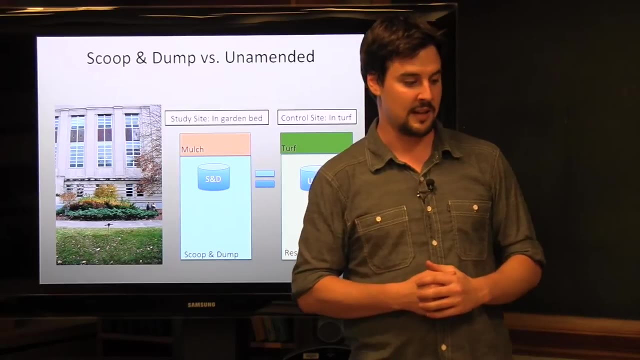 year, as you would in any kind of landscape bed establishment, and we selected our unamended or control soils at the same depth as we found our scoop and dump soils. So I'm going to go through the results that we found of our study and as I discuss these, I'm also going to discuss some of the soil. 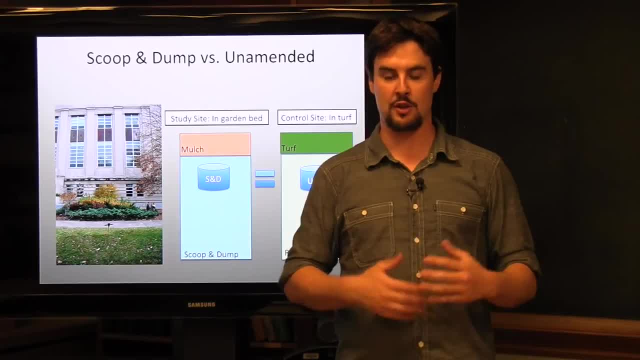 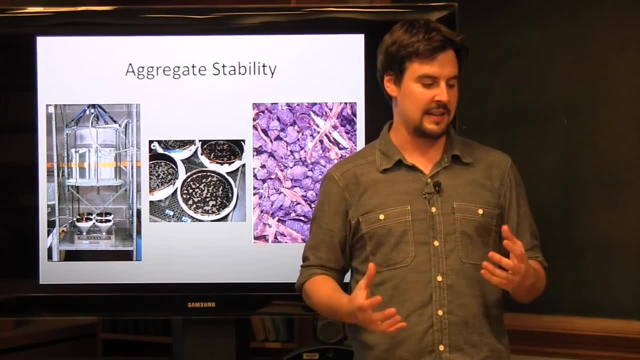 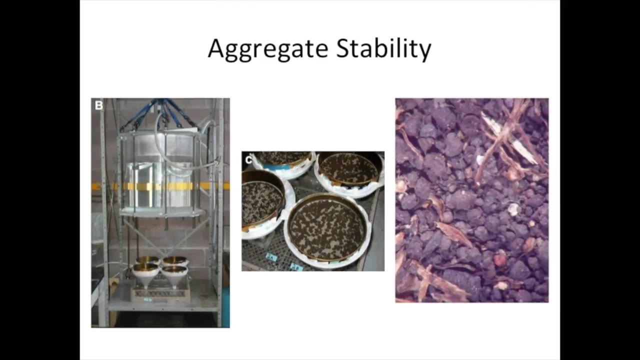 quality indicators and what they mean, so we get a sense of not just what happened, but giving a broader picture of soil health. So the first thing I'm going to talk about is aggregate stability, and what we're talking about when we're referring to aggregate stability is essentially the soil aggregates. these 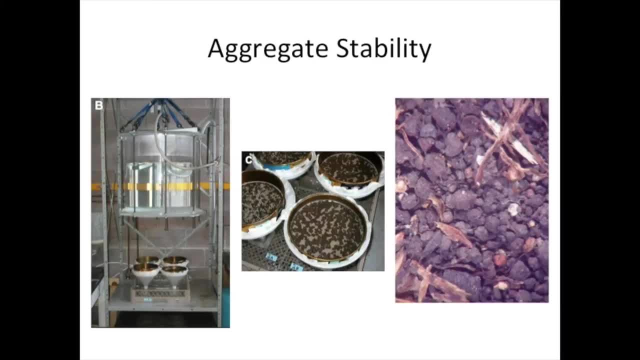 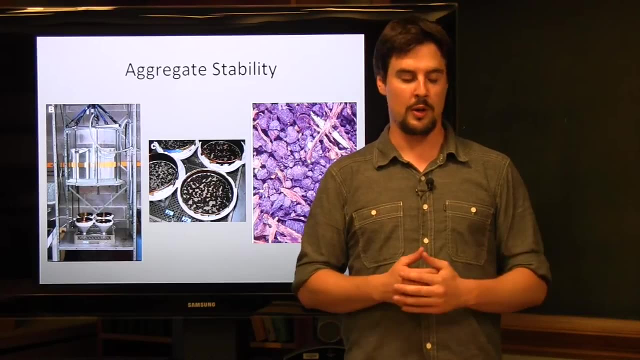 large particles that have conglomerated together and their ability to resist destruction and the destructive forces that we apply on them or water. There's two ways you can look at this. you can either look at this by flooding- how much the aggregates break apart when inundated with water- or you can look at 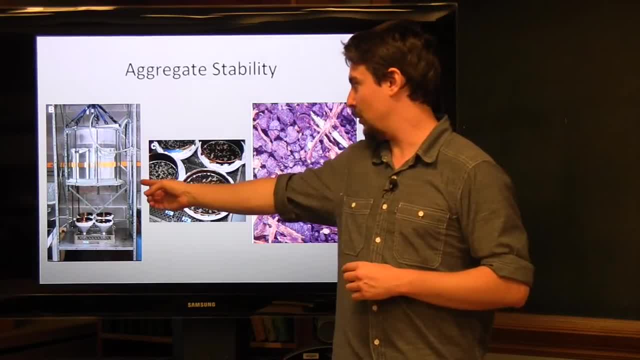 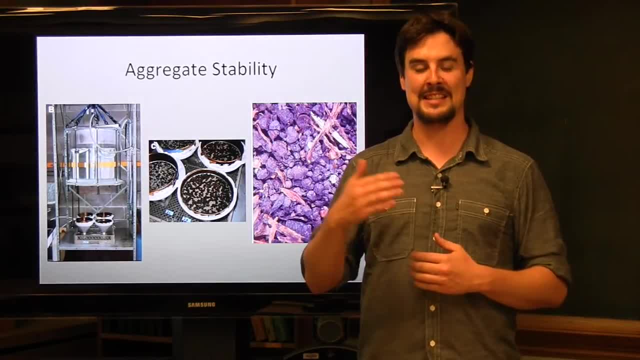 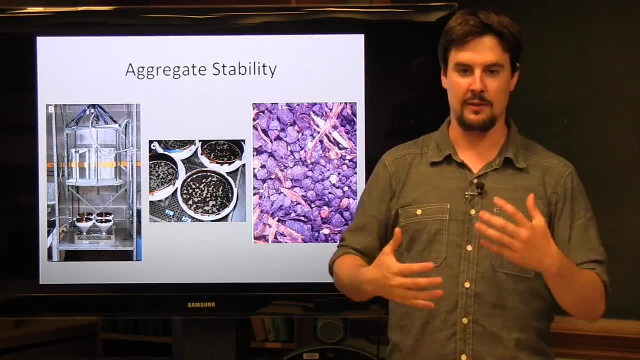 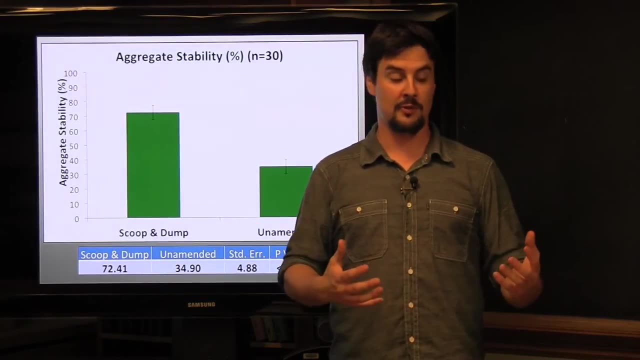 essentially the the more stable your aggregates, the less they break apart, the better that is for your soil structure and just generally creating a kind of more agreeable environments for our plant to put our plants directly into. So when we looked at the scoop and dump versus our controlled soils, what we 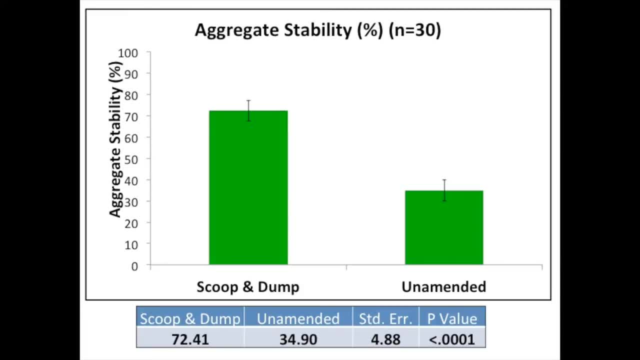 found is that our scoop and dump soils had 72 percent aggregate stability and if you compare this to our unamended, we see that are unamended is at about 34 percent. and so just by doing the scoop and dump technique, coming in and incorporating organic matter and 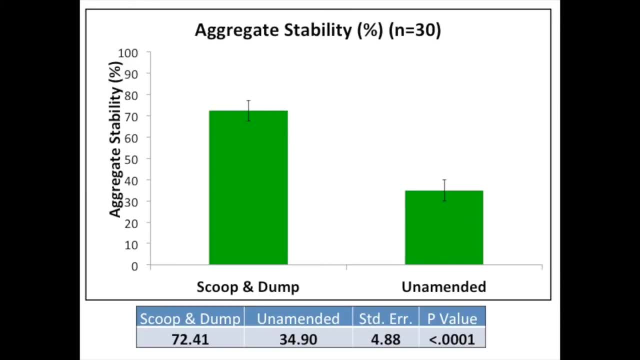 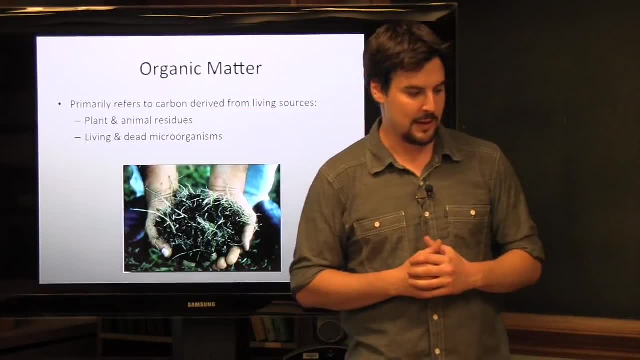 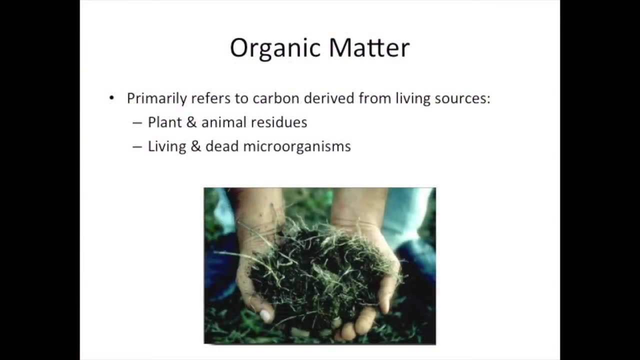 physically fracturing the soil and mulching over their site, we saw that we had almost double the amount of aggregate stability. Next we have organic matter, and what we're talking about when we're talking about organic matter is it's primarily carbon that is derived from a living source. so whether 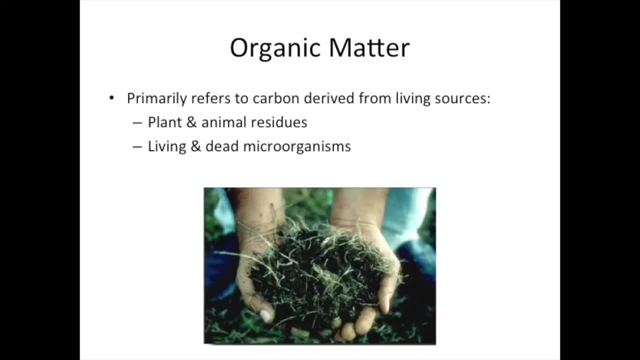 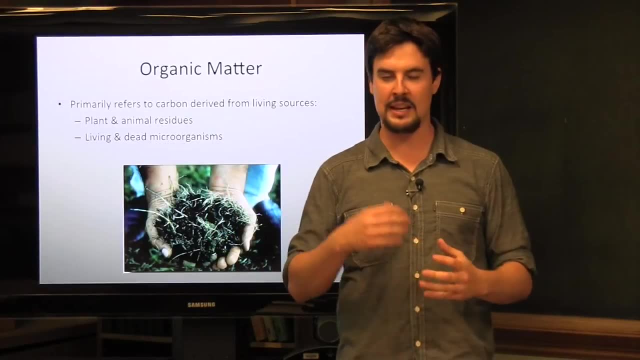 this be plant or animal residues or microorganisms that we're finding in the soil. it's a little more involved in that, but as a basic sense that's what we're referring to, and organic matter is a very important component of our soils. I think most people kind of know that the it tends to be, the more organic matter. 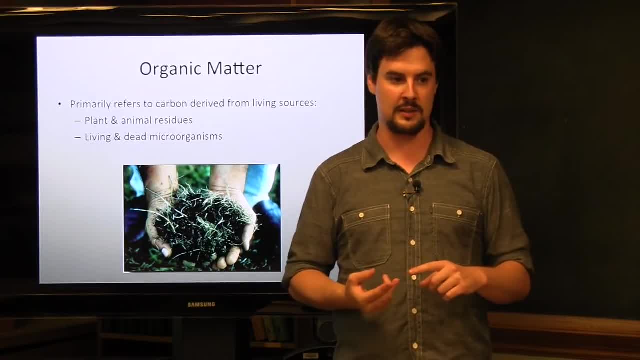 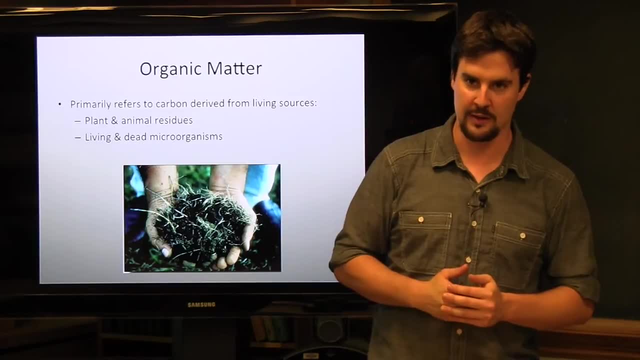 you have in the soils. it improves structure and it certainly is beneficial for cation exchange capacity, therefore, the ability for organic matter to be able to hold on to nutrients. so in a functioning ecosystem, where we want our plants to thrive and survive, organic matter is a very important indicator to 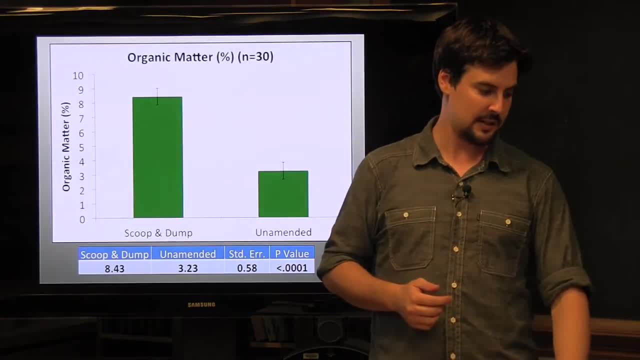 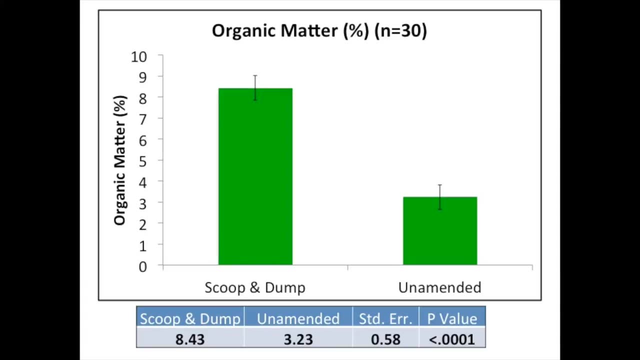 look at and on average, when we look across these sites, what we see is that our scoop and dump soils. we have eight point four, three percent organic matter, compared to our unamended. that is at three point two, three. so almost three times your organic matter after doing this incorporation, which makes sense. 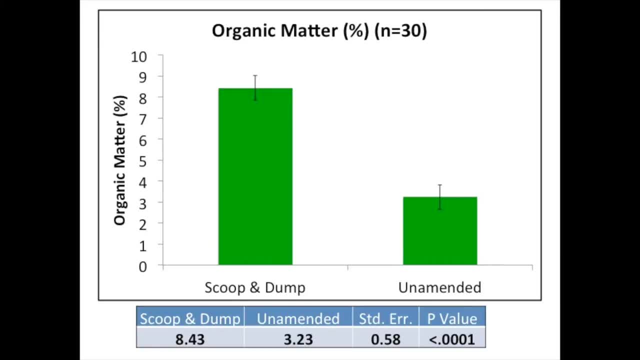 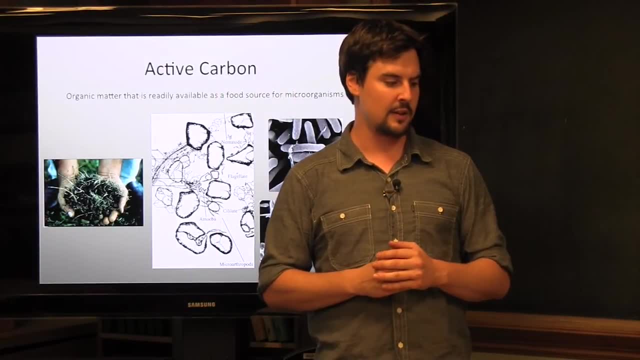 since we're adding compost, we're adding a lot of organic matter, but it's good to see this. Next there's active carbon, and this is kind of a newer test that some people may not be as familiar with. but what we're talking about when we talk about 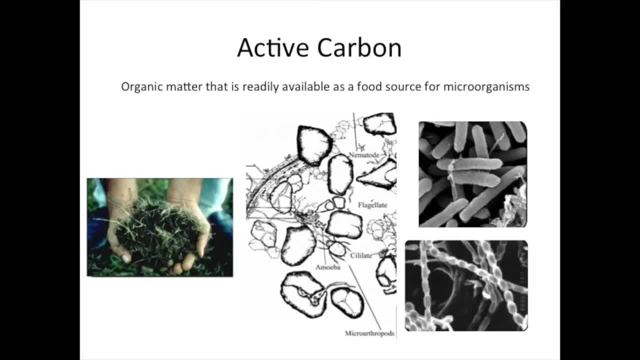 active carbon is. essentially, it's a fraction of your organic matter that is available for soil microorganisms to consume and to use as a food source. Active carbon is a biological indicator and it really is a little different than our total organic matter, because that refers to all of the, all of the. 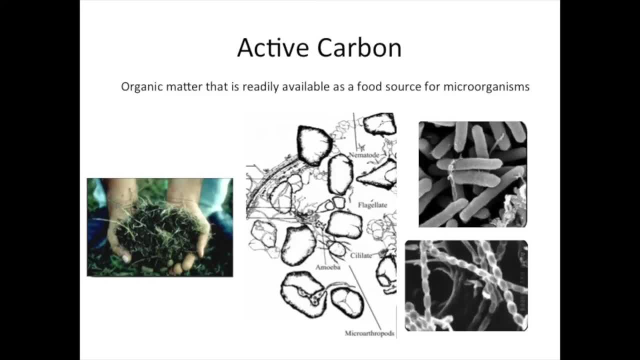 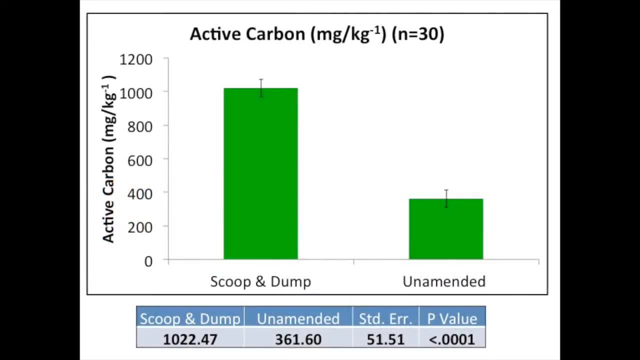 organic matter. we find active carbon is just a fraction of it and is this food source for our soil microorganisms, which play mediating roles in our nutrient turnovers. and what we see when we looked at active carbon is that- our active carbon, we are up around 1022 parts per million. compared this to our unamended. 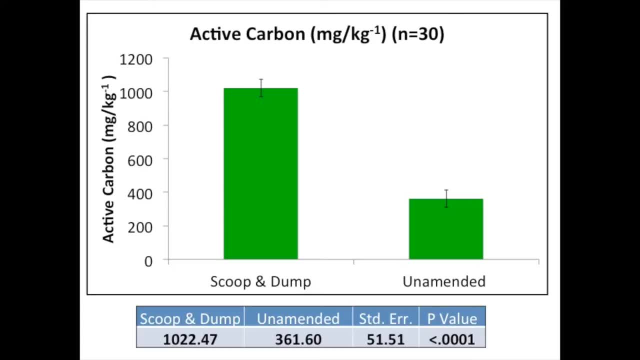 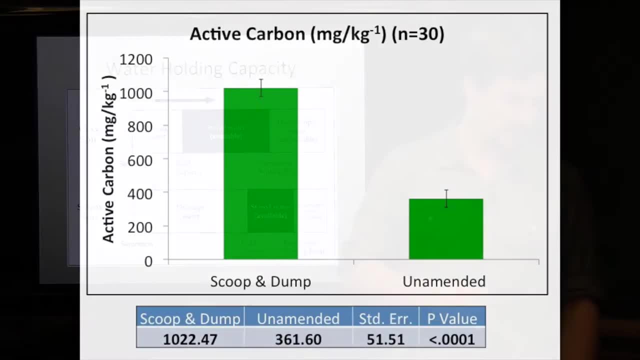 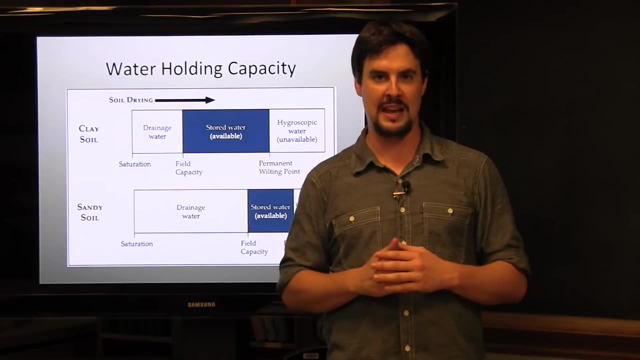 at 361.. And so almost we have more than three times the amount of active carbon in our scoop and dump soils. Moving over to water holding capacity, water holding capacity specifically refers to the amount of water that is being held in your soil that is available to plants. 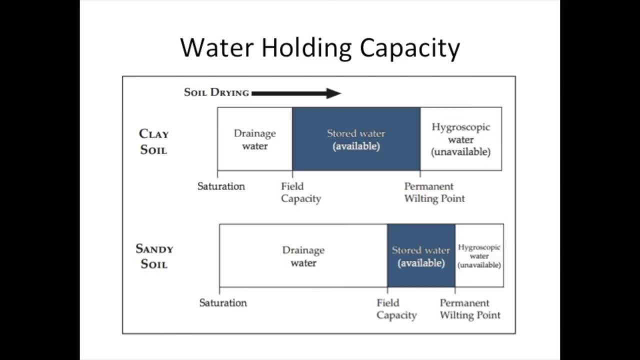 So on one end of the extreme you have field capacity, which is the amount of water that's held in the soil. when you've had a large rain event and, just due to gravity alone, the water is drained out of it. The amount of water that is held in the soil after that draining event is known as field. 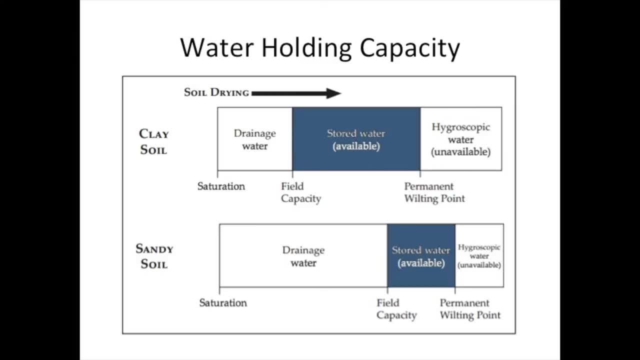 capacity, and on the other end of the spectrum you have what's known as permanent wilting point, And permanent wilting point refers to the point where the amount of water in the soil is no longer available to plants, So plants cannot pull it up from their roots and therefore the plant will start to have 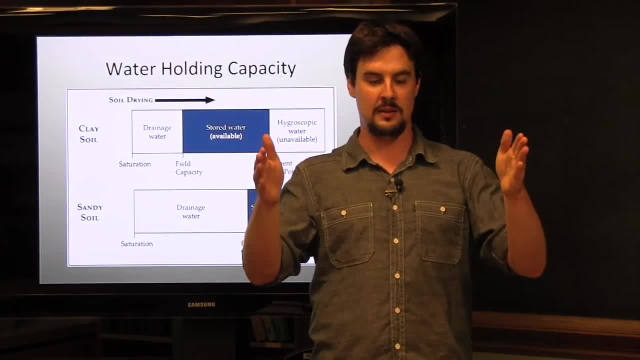 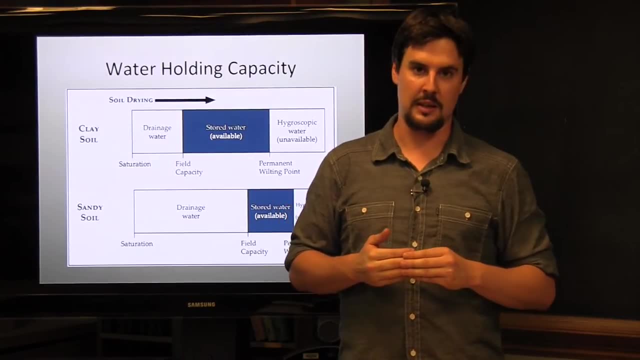 a drought response at this point. So water holding capacity is between two and three times the amount of water that is held between these two extremes. So this is very important, as you'd imagine, for thinking about irrigation and also thinking about just general maintenance of plants in the landscape. 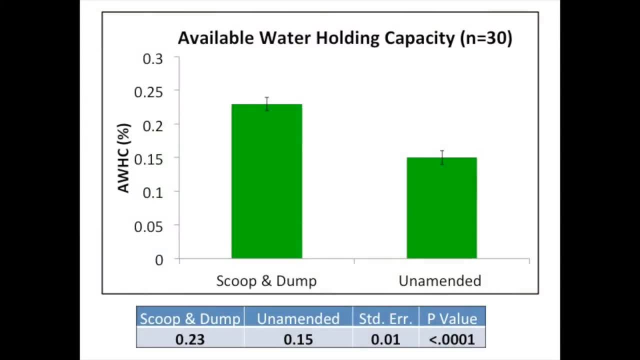 And what we see with available water holding capacity is that in our scoop and dump we ended up with 0.23, while you compare this to our unamended, which is 0.15.. And these differences may not look as large as some of our other indicators, but statistically, 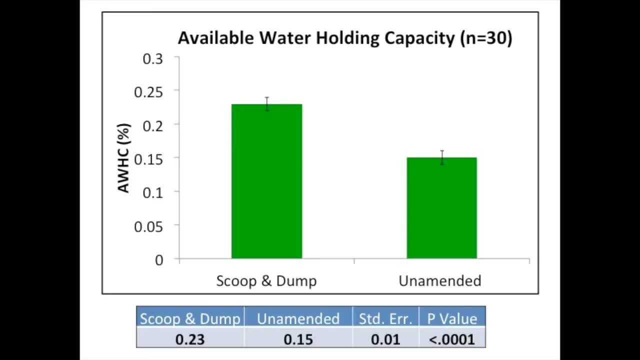 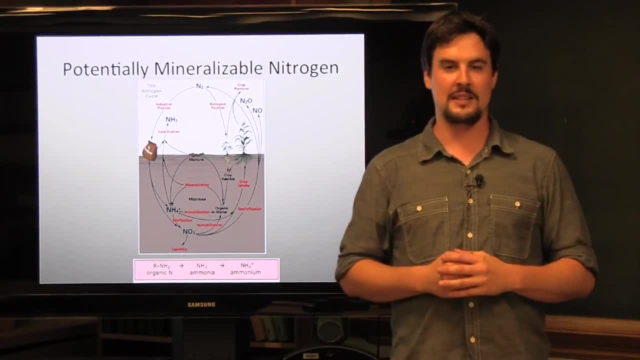 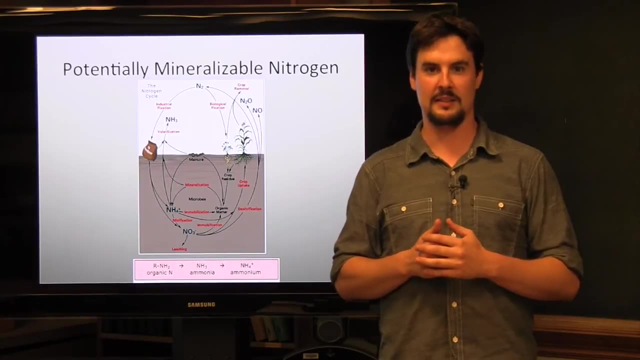 this is what we see. This is quite significant, and we see that our scoop and dump soils do hold significantly more water. So the next indicator I'm going to talk about is potentially mineralizable nitrogen, And what this indicator refers to specifically is the conversion of nitrogen from an organic 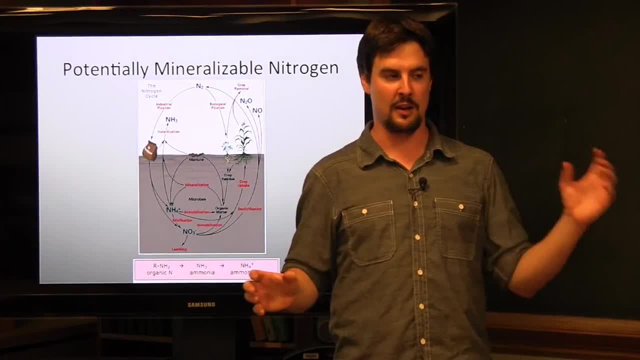 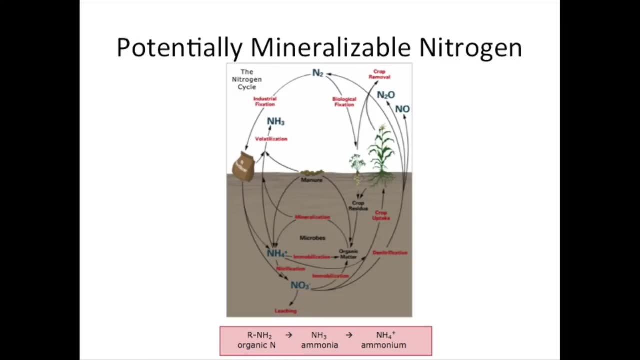 form into an inorganic form, So going from plant unavailable to plant available. And what I have up here on the picture of this slide Is the full nitrogen cycle, and I'm not going to go into full detail about this, but this is just kind of one component of it. 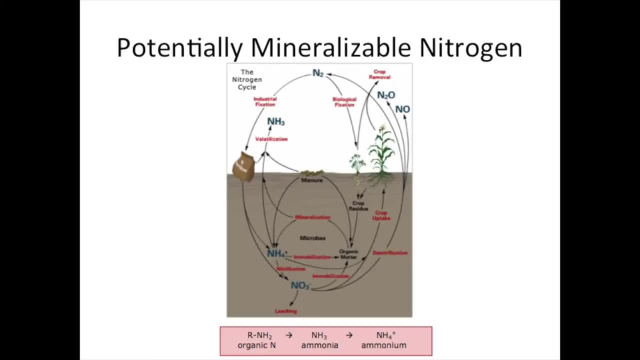 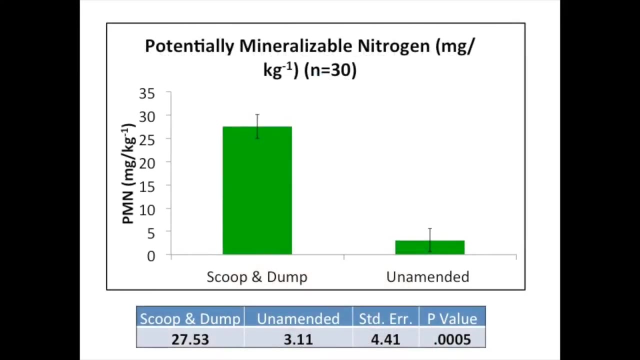 Potentially mineralizable nitrogen is another biological indicator, since this is mediated by soil microorganisms, And also since nitrogen is such an important element for, or nutrient for, plants to use, an important one to look at, And when we looked at potentially mineralizable nitrogen in our scoop and dump, compared to 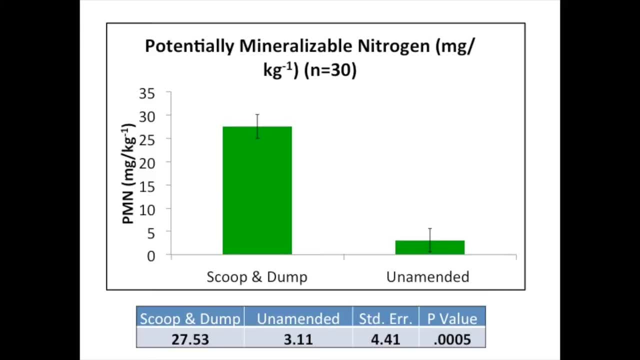 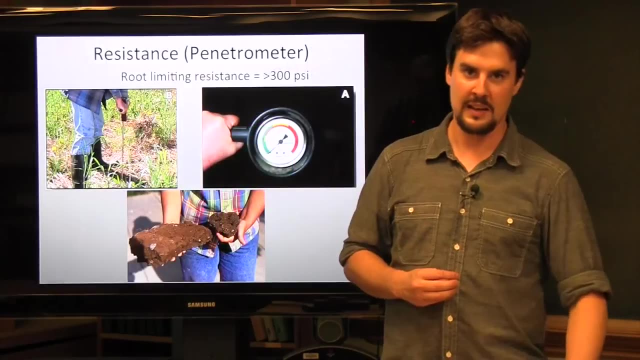 our unamended soils. What we found Is that It's almost ten times the amount of potentially mineralizable nitrogen compared to our unamended, So 27.53 parts per million compared to 3.11 in our unamended. 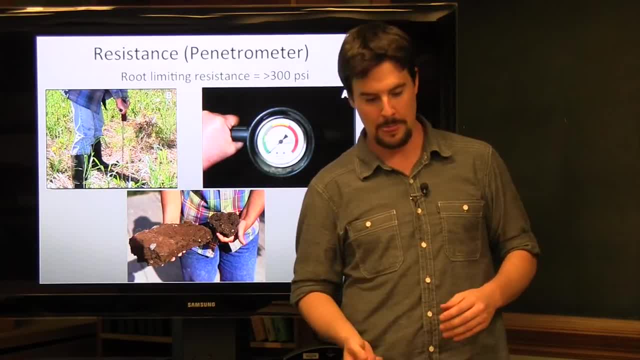 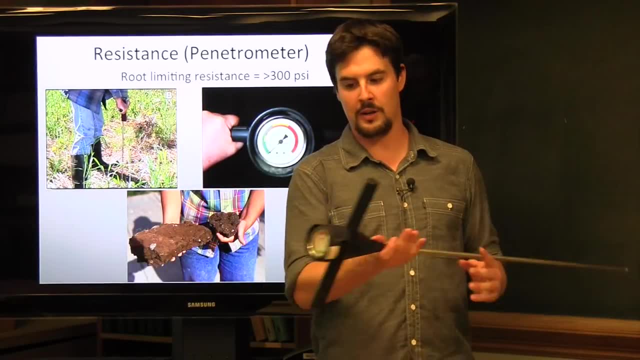 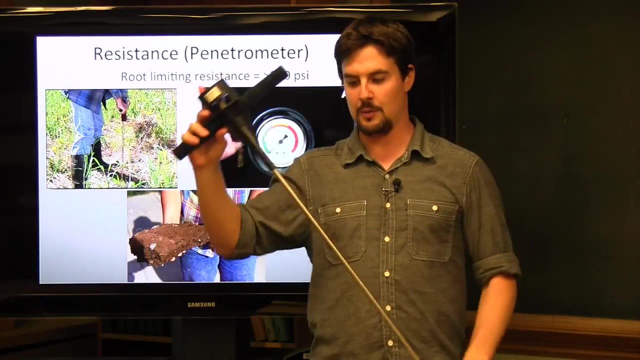 Next, we looked at resistance using a pentrometer. A pentrometer- for people who aren't familiar with it, is this instrument right here. It's pretty straight forward. It has a pressure gauge on one side and a measuring bar in the middle, And what you do is you take this and you can push it into your soil at a consistent. 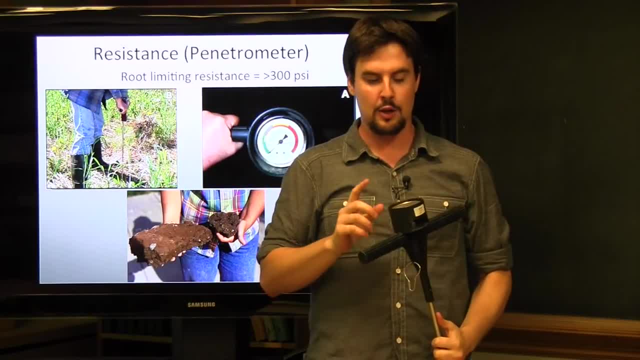 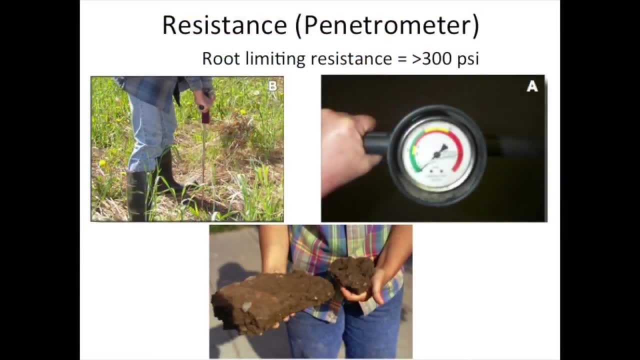 rate and measure at what point your soils reach a pressure of 300 psi or higher. And the significance of 300 psi is that that is the kind of point in your soils where roots can no longer proliferate in a compacted soil. So you know if you're below that threshold that your roots are going to grow fine if 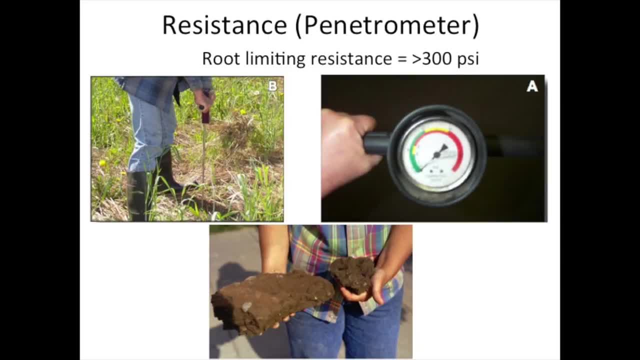 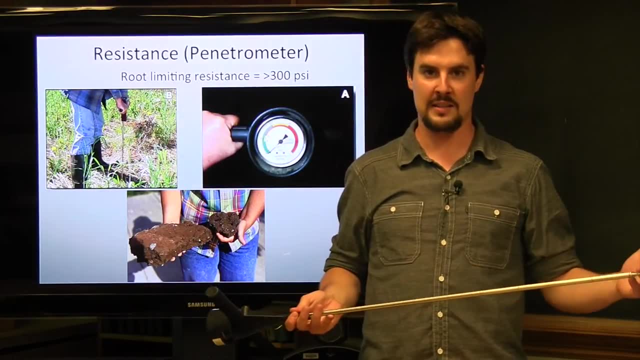 you're above it, then you're going to. you have a compaction issue and you need to address it one way or another. There are some limitations to using this instrument. It's best to use it directly a short time after it rains, especially if you're going. 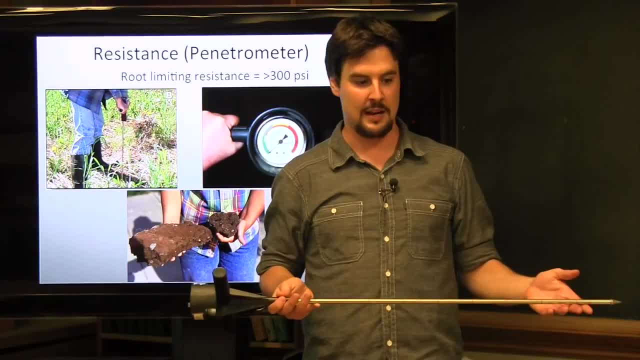 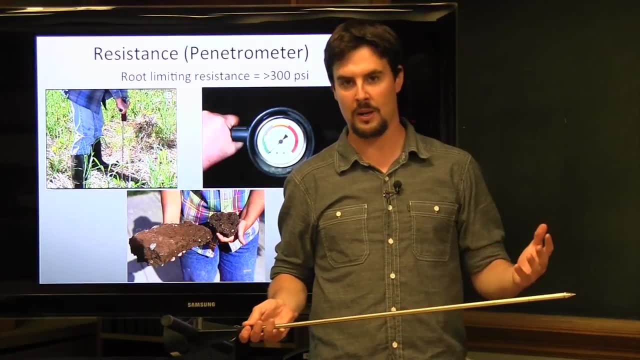 to be doing a lot of different sites because soil moisture can make a difference in how you read it, But it's a great way to just get a quick estimate of what the compaction looks like in your soil and why we talk about it in terms of soil health. 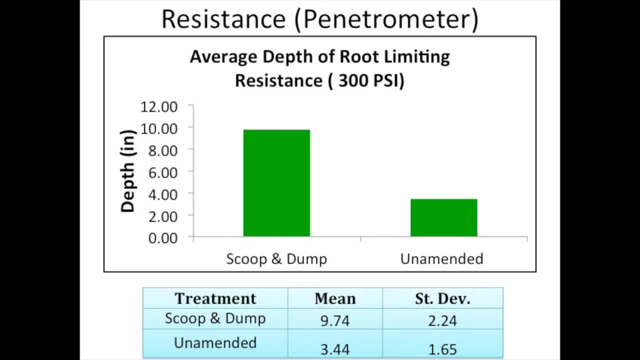 And so, when we looked at our scoop and dump compared to our unamended, What we found Is that in our scoop and dump we could go down to 9.74 inches before reaching our root limiting psi, compared to our unamended, which was at 3.44 inches. 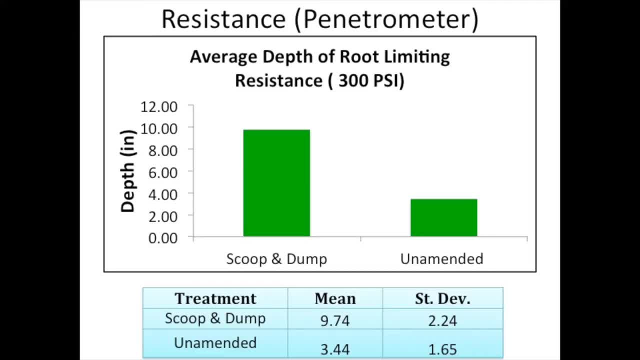 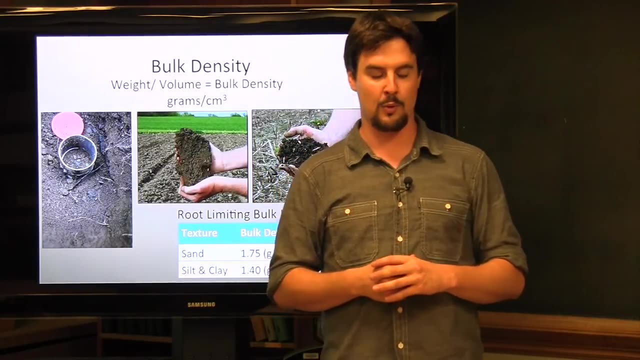 So we had three times the rooting volume or depth available to us that plants could therefore grow, explore and use. Next, we looked at bulk density And, as I I mentioned before, what bulk density is is a measure of weight by volume. 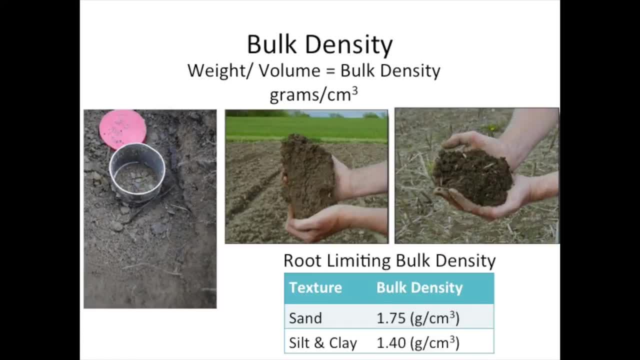 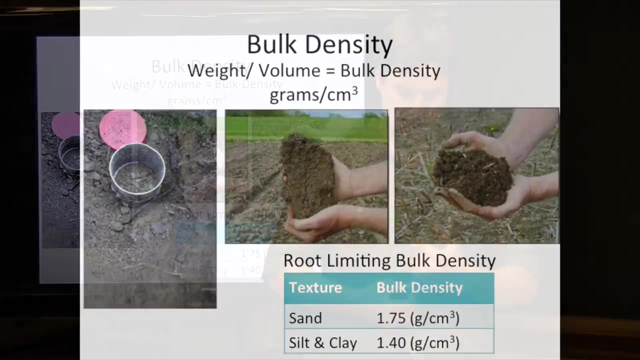 And this is another indicator that's important to consider when looking specifically at compaction. It is a little bit more telling than using the resistance measure or the pentrometer measure and pretty straightforward to take, But we use these rings typically to measure bulk density, and we'll hammer these into the 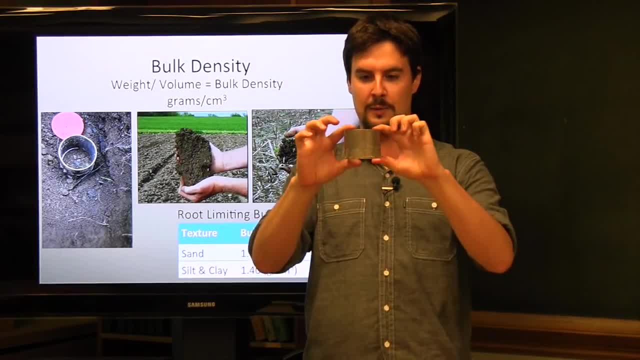 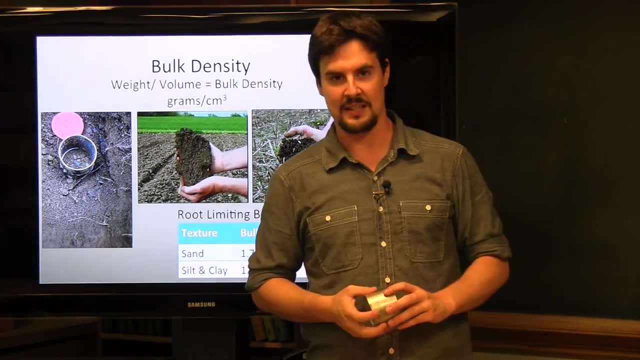 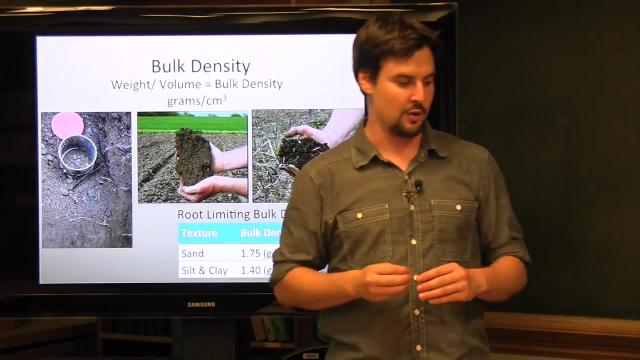 soil, get them kind of flush, so we know how much volume is in here specifically, dry them out and then weigh that. And what we can tell with bulk density, just like we can tell with resistance, is that we know, depending on texture, that once you get above a specific bulk density you start to 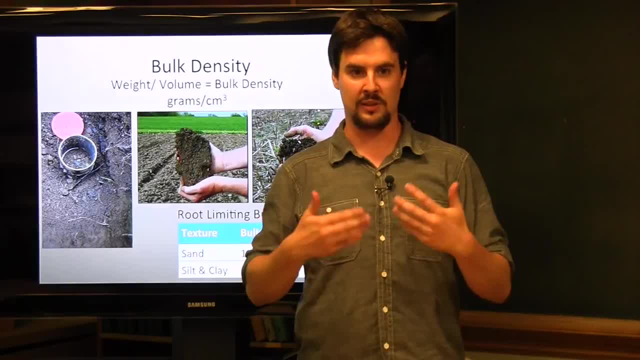 have trouble having roots grow and proliferate in your soil. So in sands it's 1.75 grams per centimeter cubed compared to 1.75 grams per centimeter cubed compared to 1.75 grams per centimeter cubed compared to. 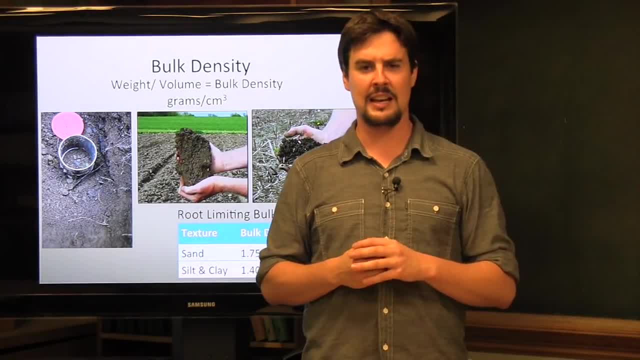 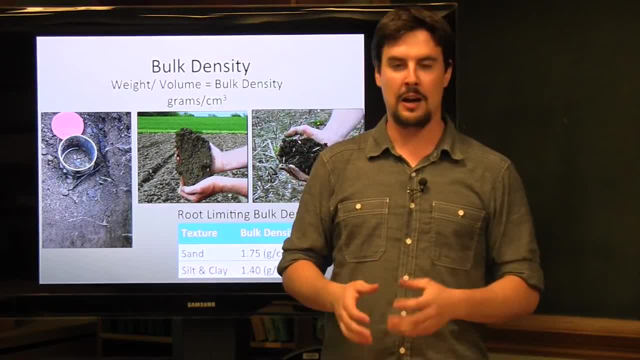 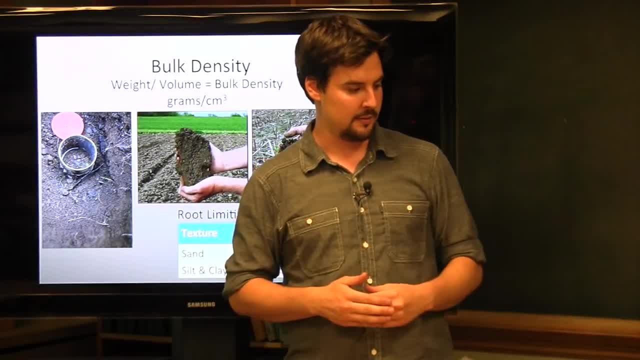 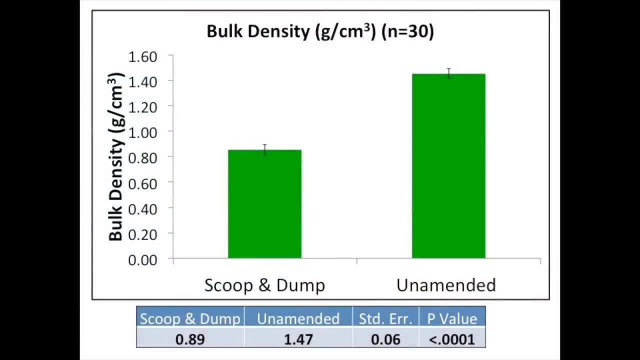 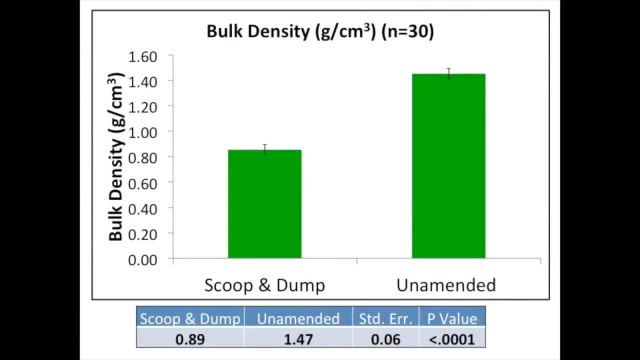 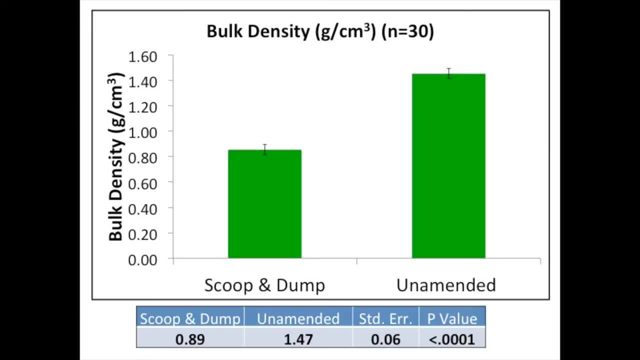 9 grams per centimeter cubed, which is well below that 1.4 threshold. So, regardless of texture, we saw that by doing this process that we were able to reduce our bulk density and create a medium where roots are going to have a much easier time growing. 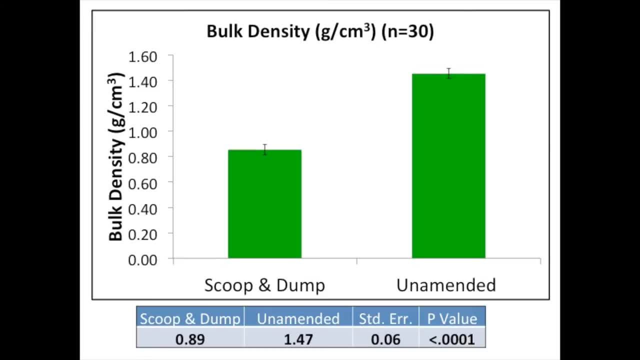 Compare this to our unamended, which is up at 1.47, and, depending on texture, you're kind of just getting to that root limiting range. So after we did our first kind of study where we looked at scuba dump soils in a compare. 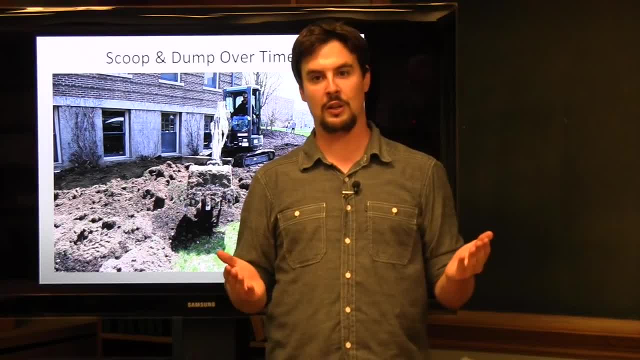 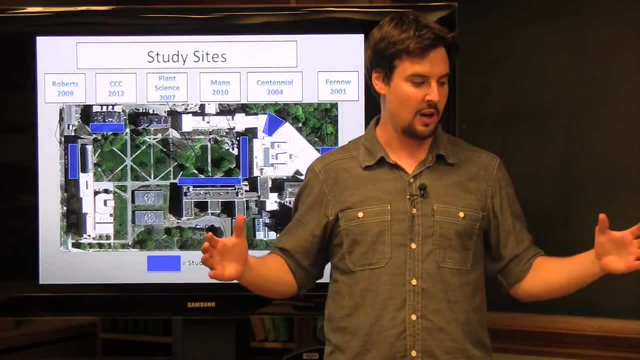 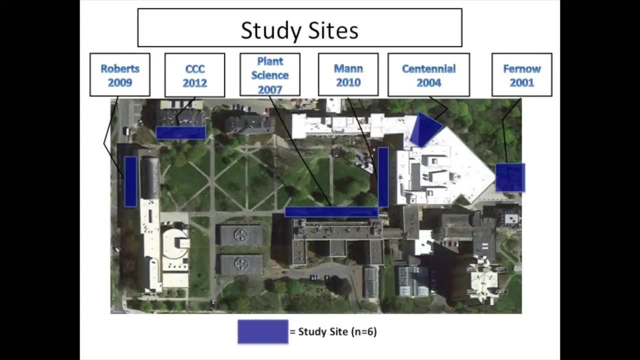 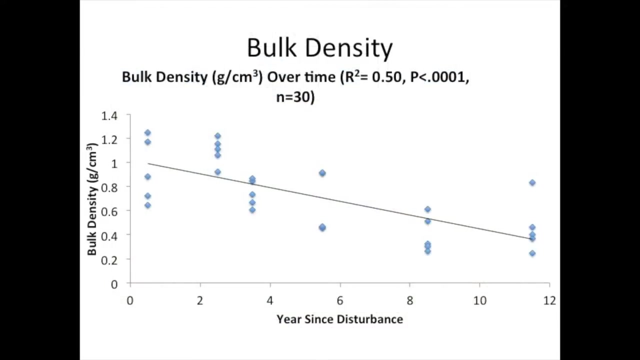 and contrast setting. we also wanted to look at how did these soils change over time. So we selected a cross-section of 12 years and we selected six sites out of those that represented that time frame, And when we looked at this in chronosequence, what we found out is that, over time, our bulk 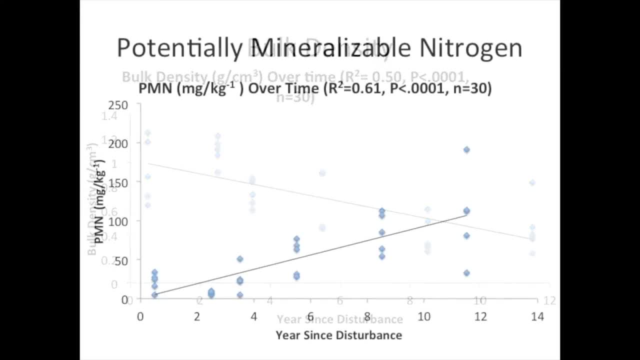 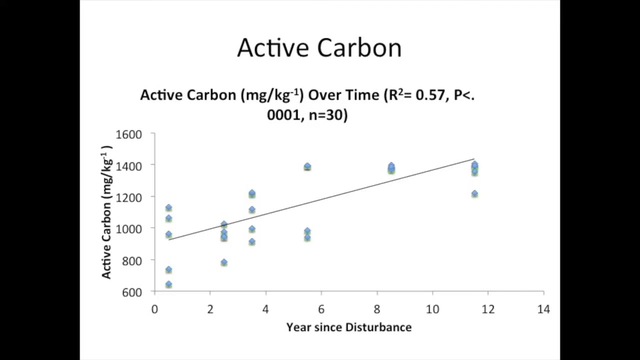 density decreased, We found that our potentially mineralizable nitrogen- our nitrogen that is being converted from an organic to an inorganic form- also significantly increased over time, as well as our active carbon, the portion of our total organic matter that is available for microorganisms. 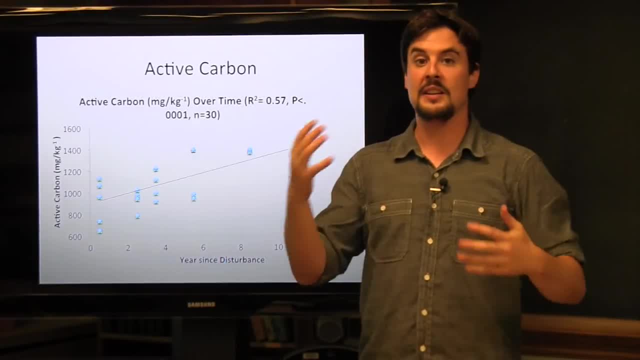 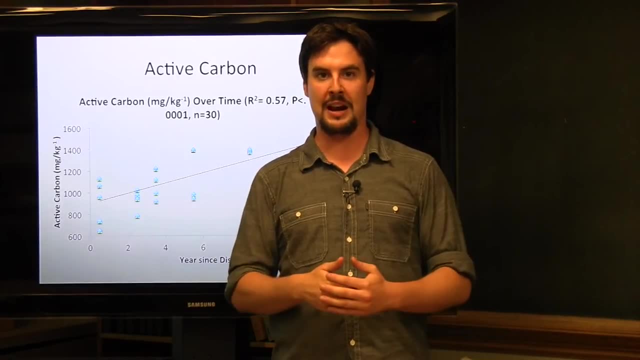 to use as a food source. And it was really exciting to see, Because when we did our first study, what we could see is that, yes, by going in and doing the scuba dump practice, we improved soil quality almost immediately. And that was the first piece of data. 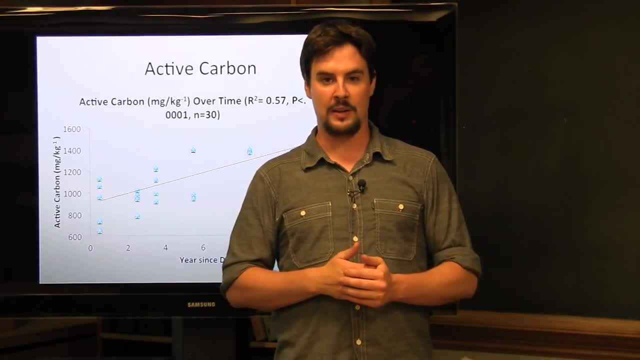 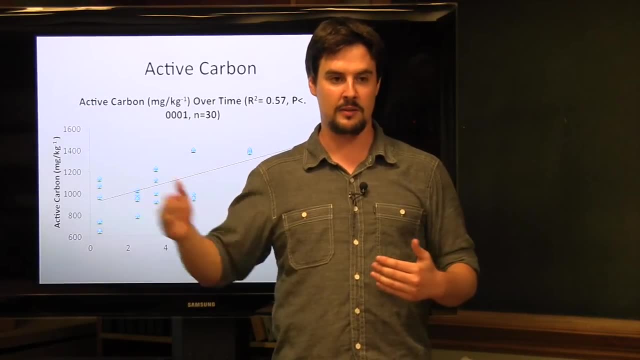 What we saw when we looked at this over time is that by going in and doing this once and then mulching every year, that there is an increased benefit that keeps on going after we've used this technique. Active carbon as well as potentially mineralizable nitrogen. 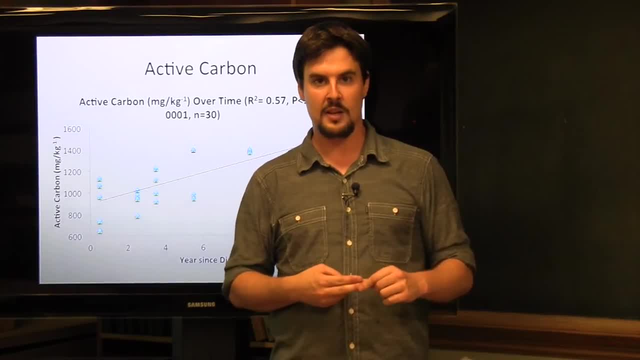 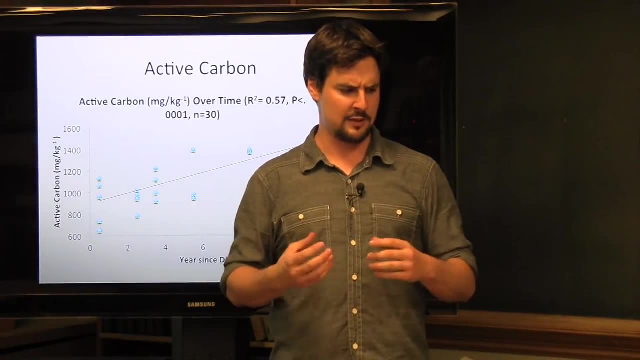 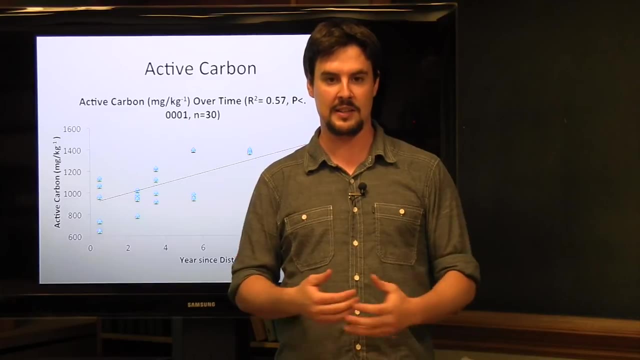 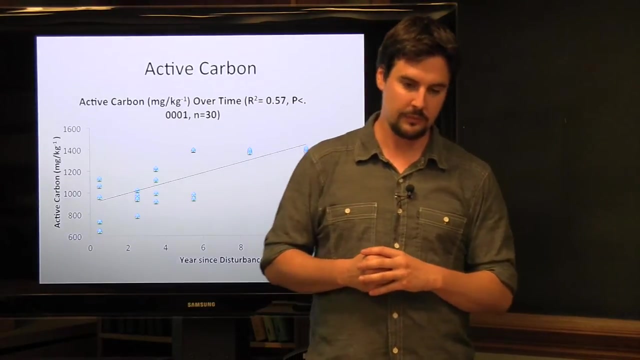 So that's the first piece of data. We also wanted to look at what we're seeing. We have this, So this is all very exciting to see. And what we wanted to do next was say, all right, we've seen that we've improved our. 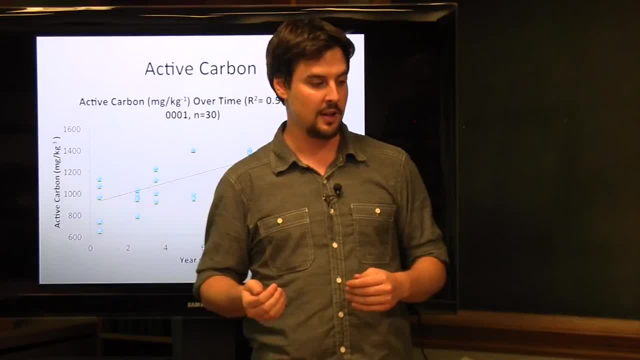 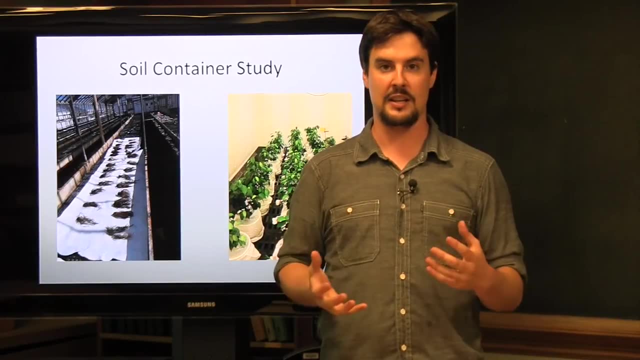 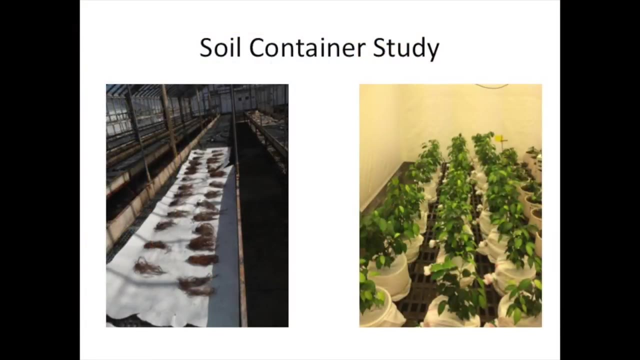 soil quality- great thing. but we also want to see how plants respond to these changes in soil quality. So we set up a soil container study where we went out again to our scoop and dump sites and our unamended sites and we took large cores, PVC cores, that we hammered into the ground. 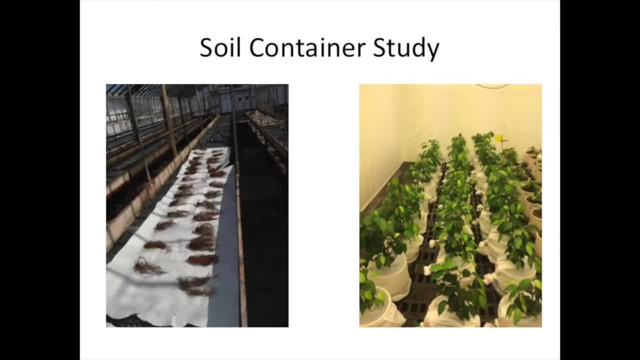 and pulled out, and we were then able to take these soils, bring them into a growth chamber and grow plants in them, specifically to see how the plants responded to this improved environment, And we were able to look at a number of different factors. but first what we did when we took these. 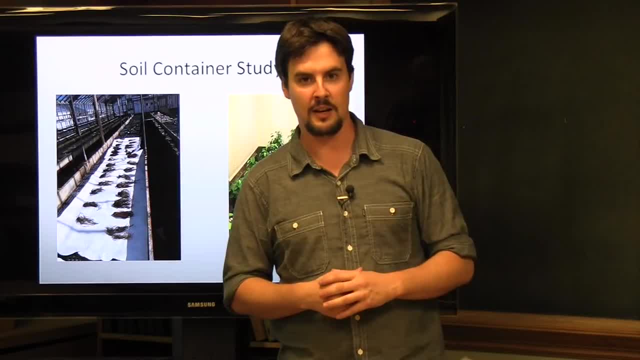 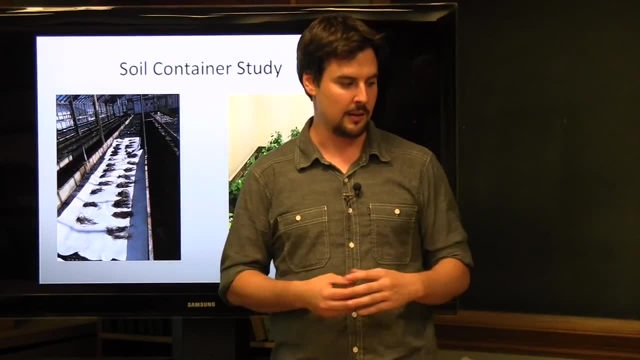 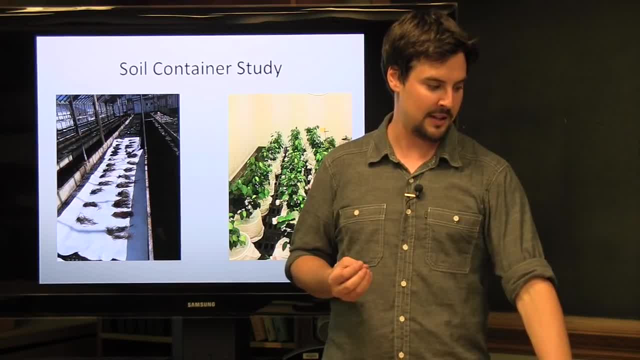 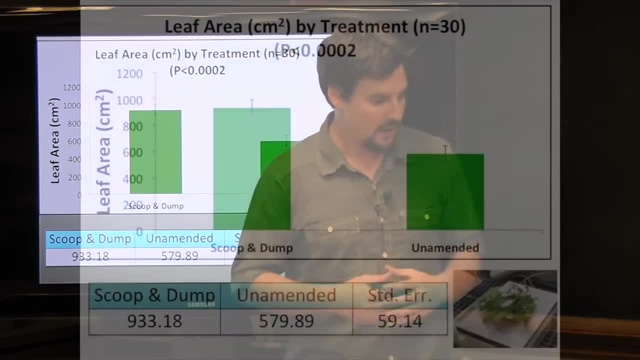 and we took a little bit of soil. and we took a little bit of soil and we looked at after growing and establishing these ficus benjamina was how, just what were the growths? plant growth response. So we see here that in our scoop and dump soils, compared to our unamended 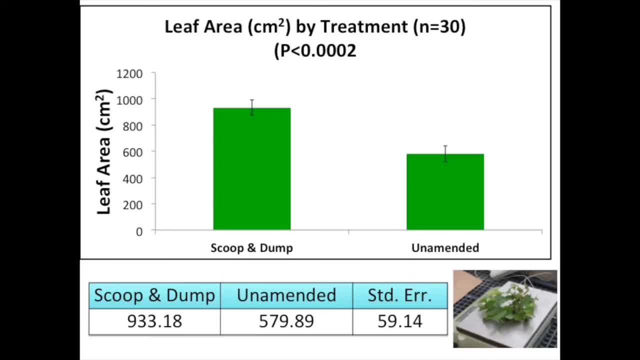 ficus that were grown in there had significantly more leaf area. Leaf area was the first indicator that we looked at, up at 933 centimeters squared, compared to our unamended, which was at 420 centimeters squared. 578 centimeters squared. 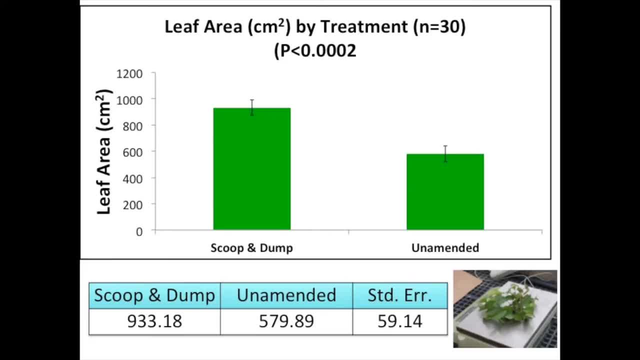 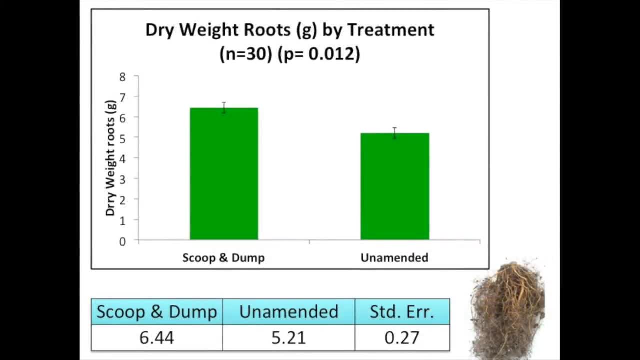 So significantly more leaf area was put on by the plants growing just in the scoop and dump soil. When we destructively harvested and extracted the roots and the shoots from the plants, what we found is that we had significantly more dry weight of roots for plants growing in our scoop and dump soil. 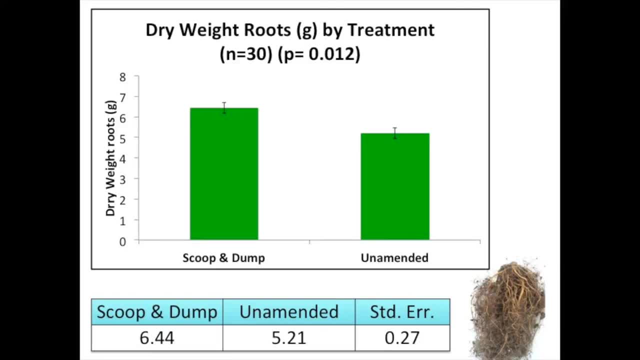 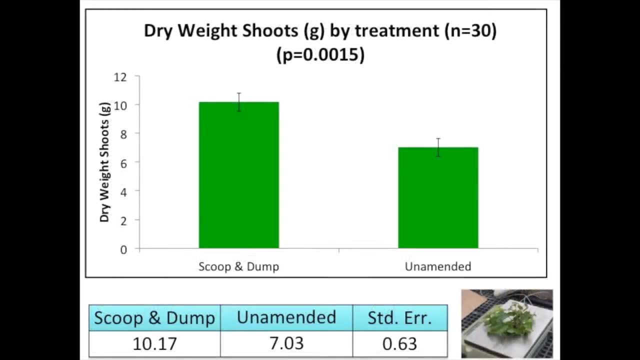 compared to our unamended. And again, these differences do not look giant, but statistically they are significantly different. As well as the dry weight of shoots, We also had significantly more shoot growth compared in our scoop and dump soils compared to our unamended. 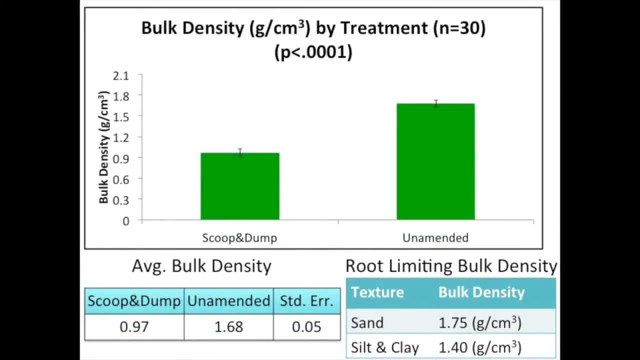 So again, like in our last study, we also looked at bulk density, this measure of weight by volume, And what we found again is that our scoop and dump soils were at this 0.97 range, which is again well below that 1.4 threshold. 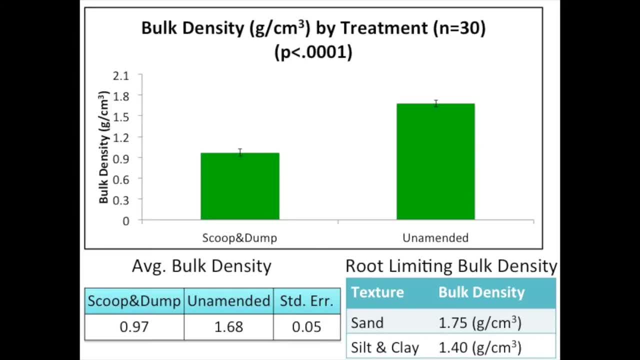 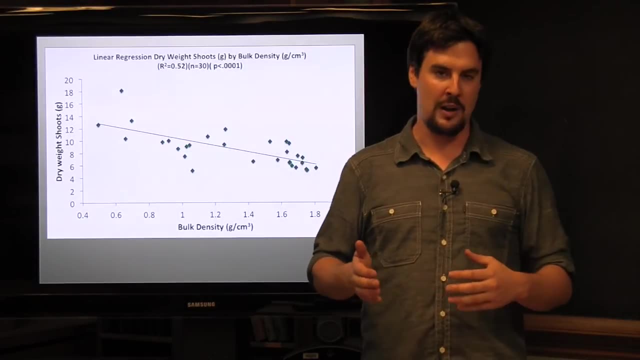 compared to our unamended soils, which are up in the 1.68 on average range, And we're starting to see limitations in the soil based on that. So what we did is we did a linear regression where we looked at bulk density by our dry weight of shoots. 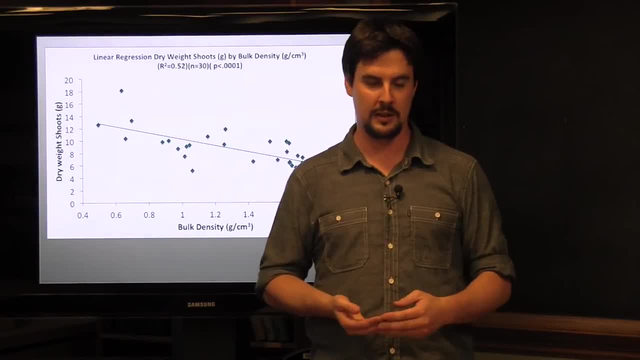 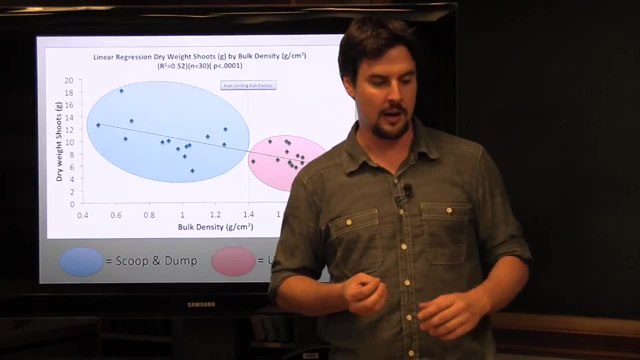 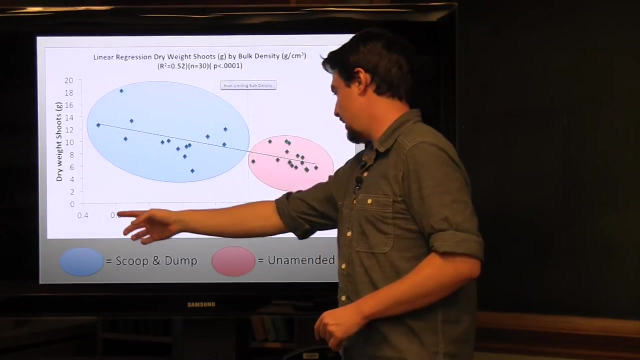 So shoots, referring to everything from the soil line up, So leaves and any woody biomass that was developed, And what we see is a very strong relationship here. In the blue we have our scoop and dump. We have more shoots on the axis here. 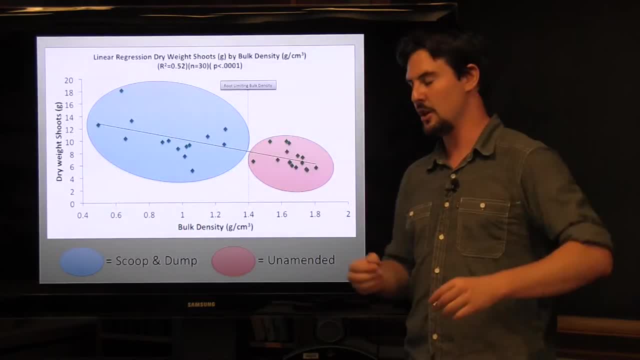 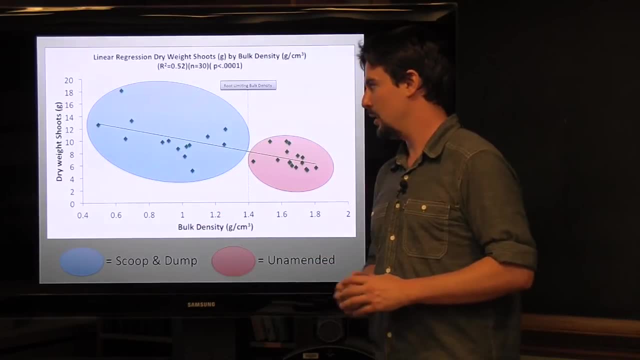 as well as higher bulk densities. So what we see is a very clear relationship where we're actually looking at the lower. all bulk density is correlating very strongly with more dry weights of shoots, And we can see in our unamended soil that you know. this line. right here is our 1.4 threshold, where you start seeing root limiting bulk densities. They're all kind of clustered down, And when we look at the dry weight of roots as well, we see a very similar pattern of our reduced bulk density. 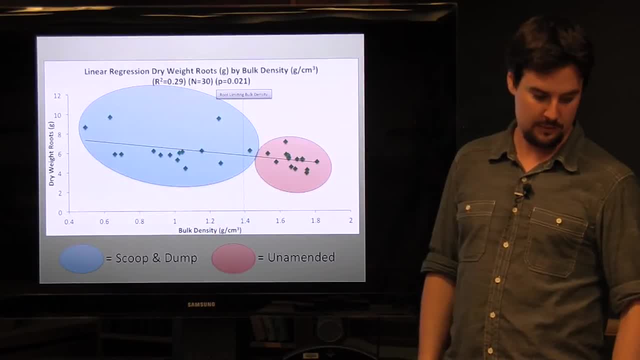 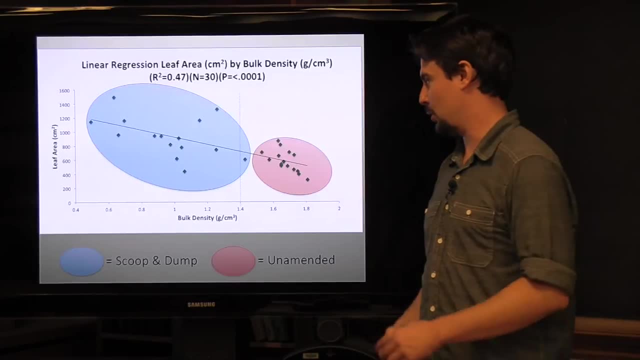 correlating with more root growth as well as our leaf area. We see the same pattern yet again, where we have strong correlations with reductions in bulk density and increases in root density, And we see the same pattern again, where we have strong correlations. 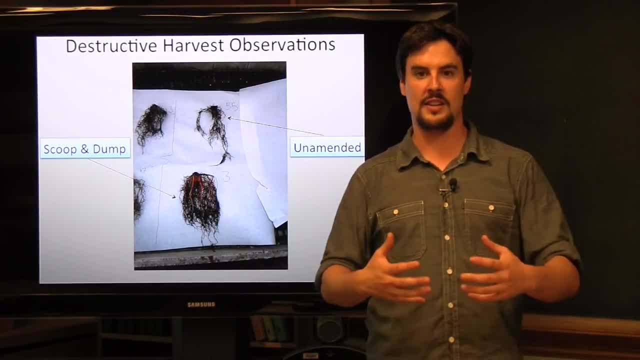 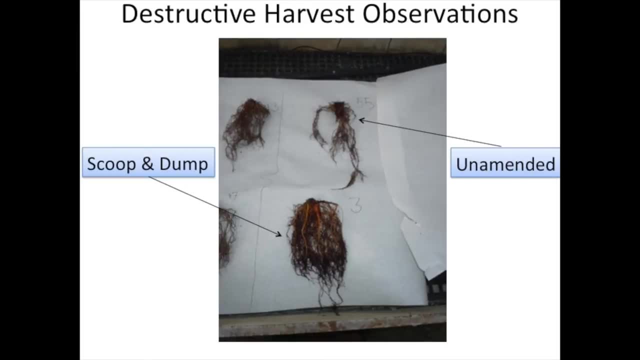 with reductions in bulk density and increases in leaf area. So when we did this destructive harvest, after we had pulled the plants out of the soils containers that they had been growing in, there was a few observations that were made that weren't so easy to necessarily quantify. 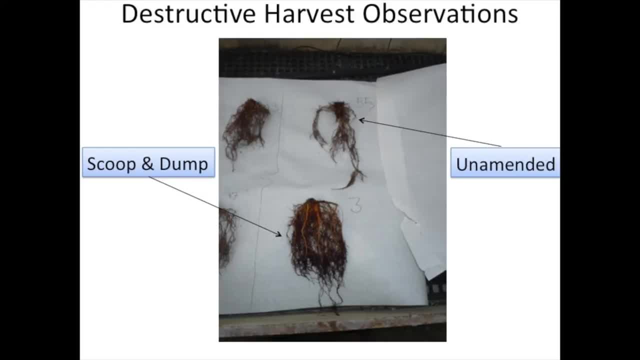 And one of the big things that we saw was just where the roots were exploring in these containers and how much more you know biomass are putting on. So this is a pretty clear picture of our scoop and dump roots. You can see a lot more. 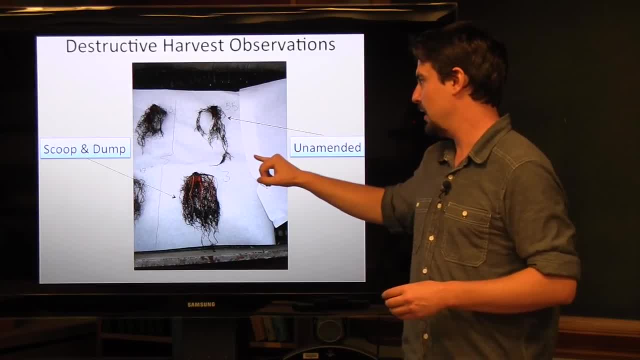 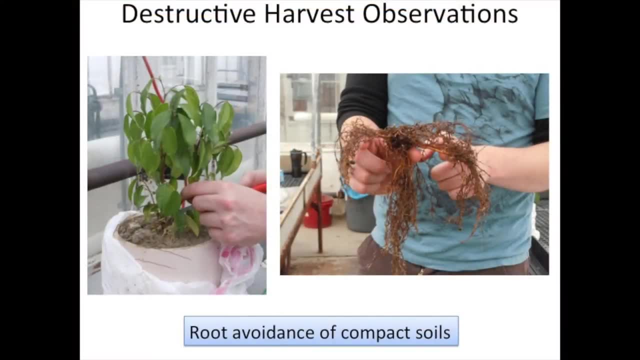 a much larger root system developing here compared to our unamended, which is just not nearly as dense. And what was interesting when we looked specifically at where the roots were in the container is that in our unamended soils, plants that were growing in our soils. 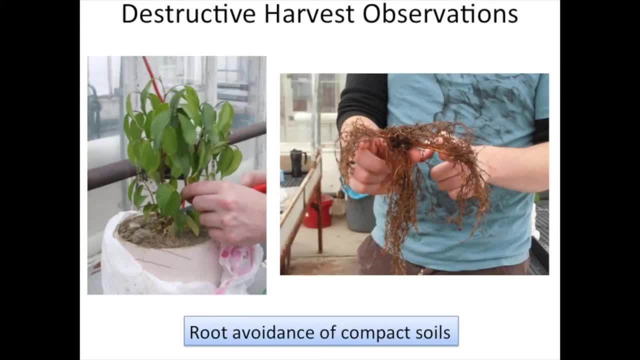 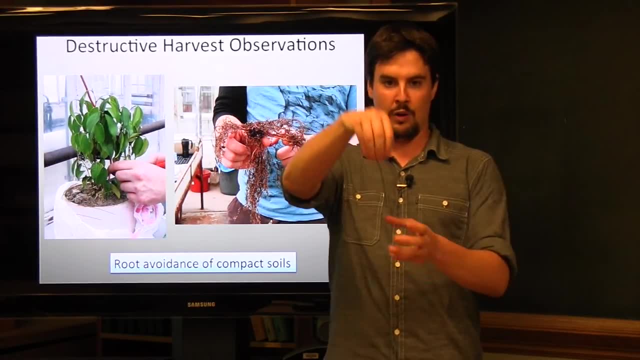 that had not been remediated, that had this higher bulk density. what we would typically see is that where we planted the, the ficus in the container, there would be roots that were growing right where we stuck the plug in, And then oftentimes what the roots would do. 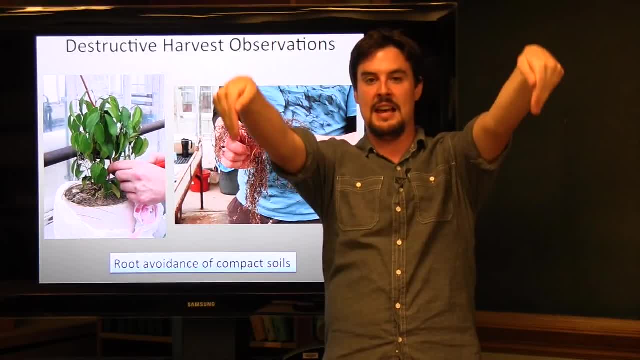 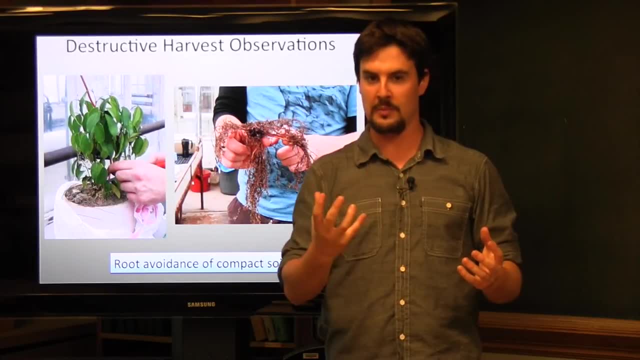 is they'd grow up from that plug across the top of the container and then down the sides, And so what the roots were actually doing in this scenario was they were not exploring the majority of the soil volume in these unamended soils, but finding a way to kind of follow the path. 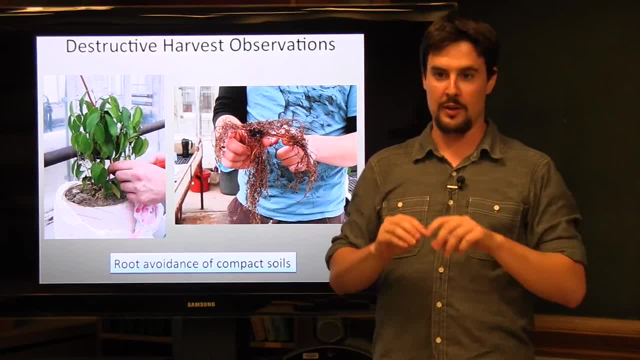 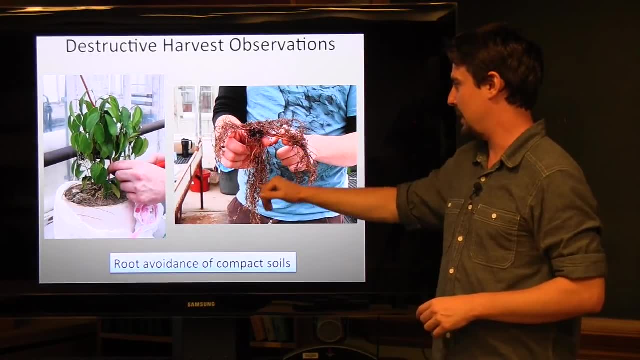 of least resistance and looking for an area where they could grow and escape. So it's a very similar pattern that you see here, where you kind of it came down. you kind of came down the middle where you planted the plug and then they'd escape off to the side. 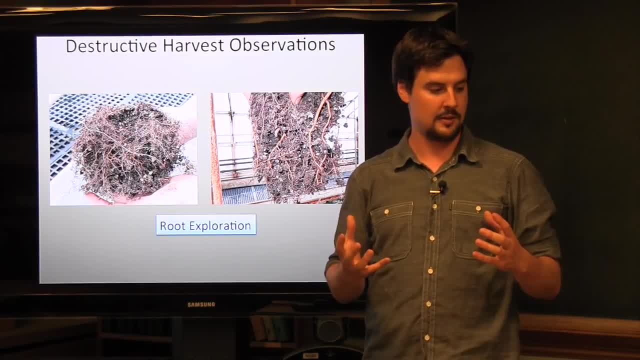 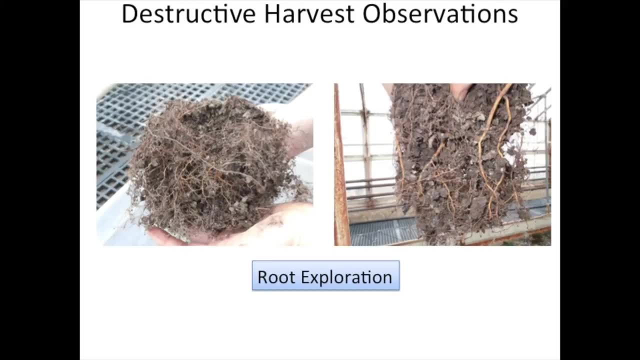 If you compare this to what we see in our scoop and dump soils, the roots growing in our scoop and dump soils had the ability to really grow throughout the full amount of the soil volume. They'd explore between those aggregates and those different air space. 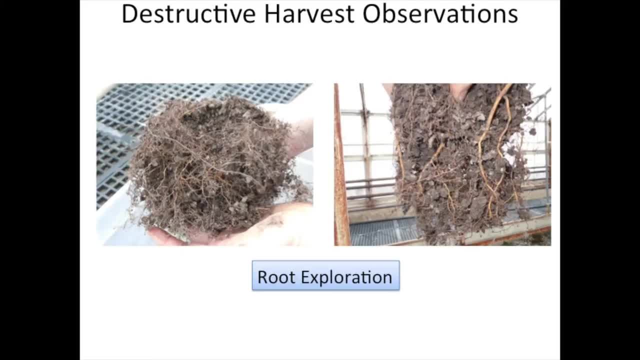 And they the volume. they wouldn't do the same escaping pattern, They would just grow throughout the whole container. And even when you tried to break the soils apart in your unamended soils, when you'd start to break the roots and the soil apart, 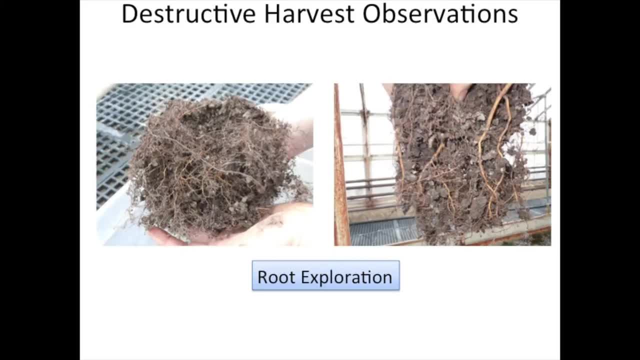 the soil would just kind of fall away In our scoop and dump soils. you'd be- you'd really have to work really hard to actually free the soil from the roots to be able to get this. So this was all exciting to see. 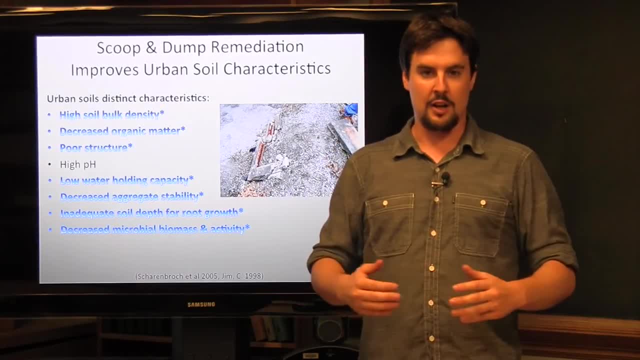 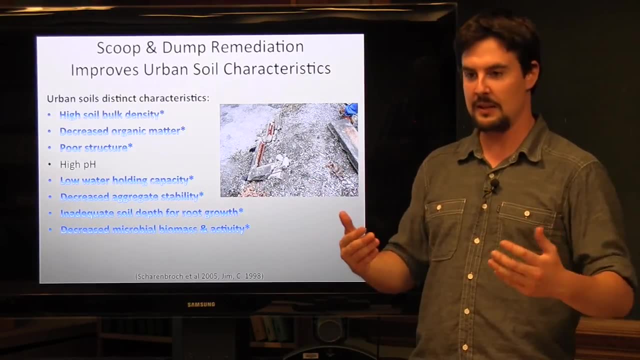 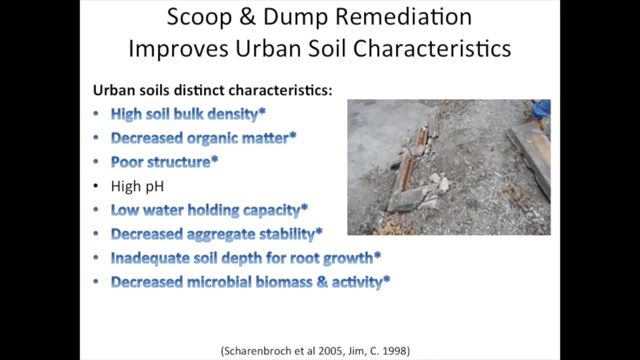 And kind of in summary. I talked about early on that- some of the issues that we see in urban soils and characterization, And by coming in and doing the scoop and dump process we've been able to improve the majority of them, pretty much everything except for the high pH. 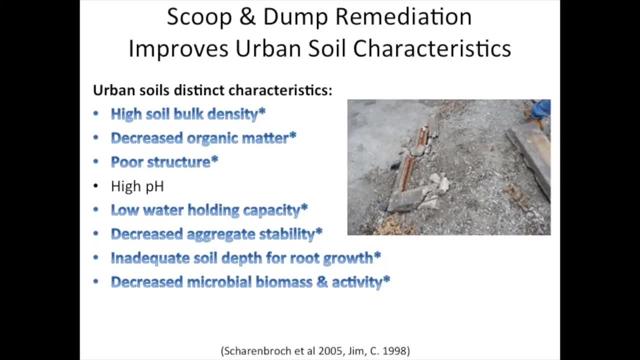 So by doing the scoop and dump process, we are able to decrease our bulk densities, increase our organic matter, improve our soil structure, increase our water holding capacity, increase our aggregate stability, improve our soil microorganism community and as well as. 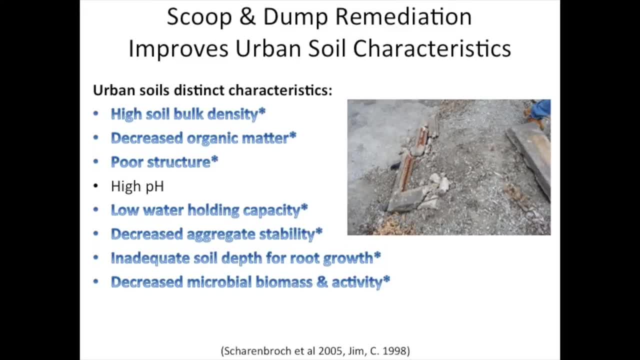 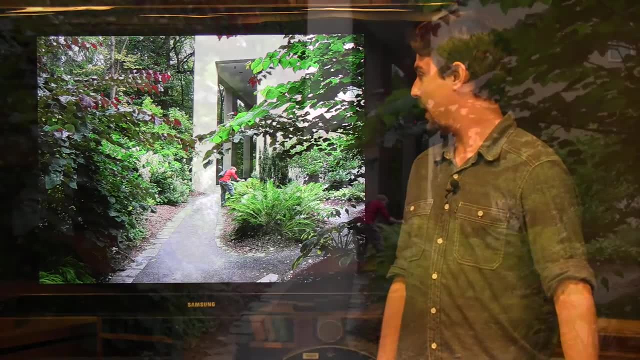 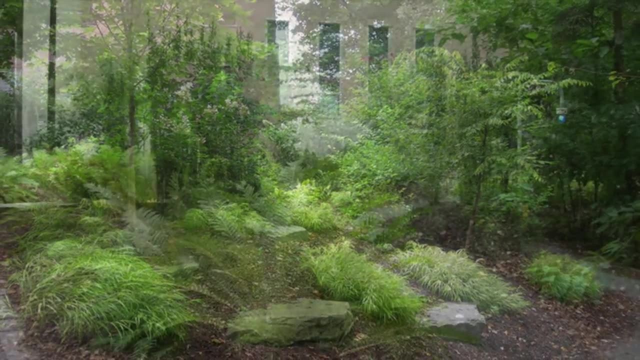 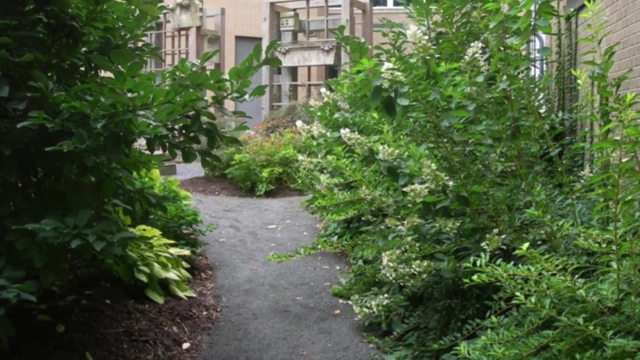 create more soil volume for plants to be able to explore. So here are a few shots of locations where we've used this technique and what some of the gardens look like today. Okay, so I'm gonna take the last little bit of time in this talk to 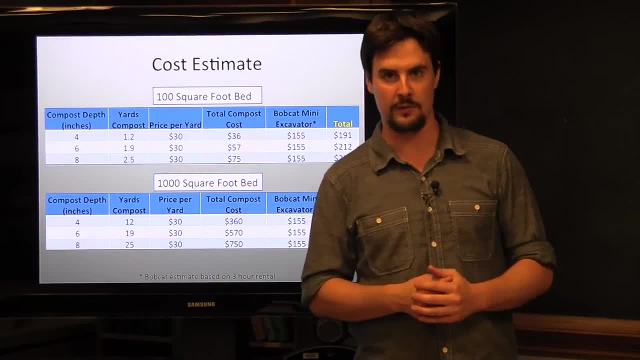 I'm gonna take the last little bit of time in this talk to Okay. so I'm gonna take the last little bit of time in this talk to talk about some of the practicalities of implementing this technique And the first thing I wanna show. 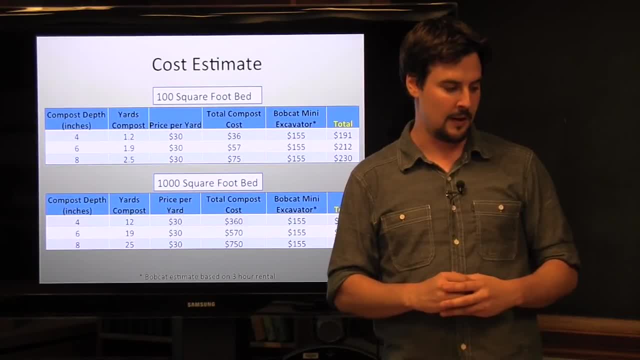 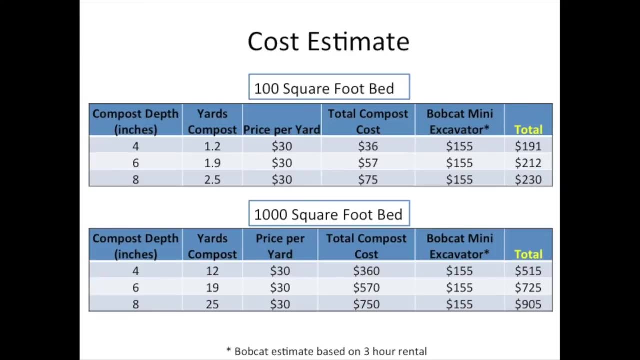 is just a cost estimate of some of the parameters that we're looking at if we wanna actually implement this. The main costs associated with the scoop and dump technique are your compost as well as getting a backhoe machine in to use. So, depending on where you work, 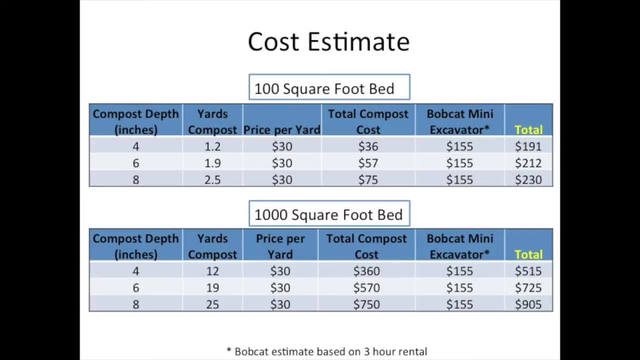 if you work in a place that already has access, if you make your own compost, this cost can be eliminated or decreased, as well as if you work in a place where you have access to a machine, then the rental costs that I've projected here 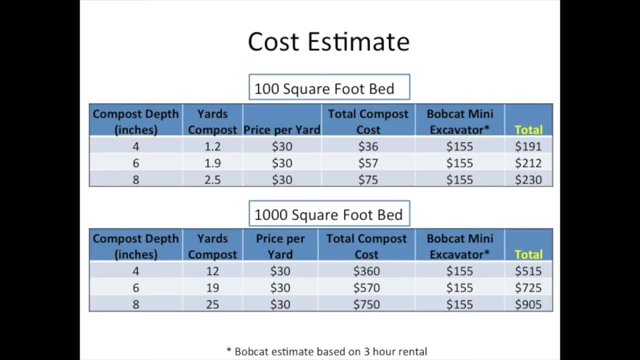 are not gonna be an issue. As I mentioned before, it is possible to do this technique also just with shovels and by hand. But a very important aspect of the scoop and dump technique is doing the physical fracturing of the soil. It's not simply. 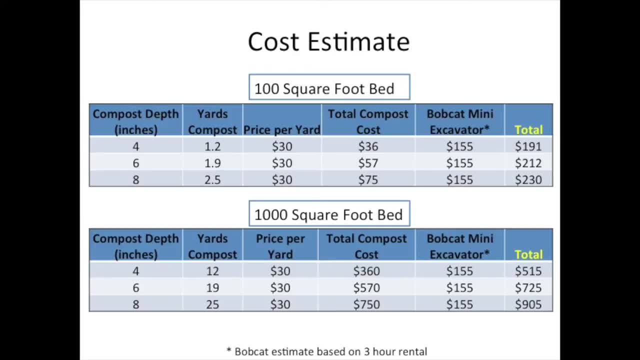 adding compost. The compost with the mixing is what creates this soil mixture and that's where we find the benefits here. So I just wanna make that point kind of clear. So estimates on an 100 square foot bed, depending if you wanna go. 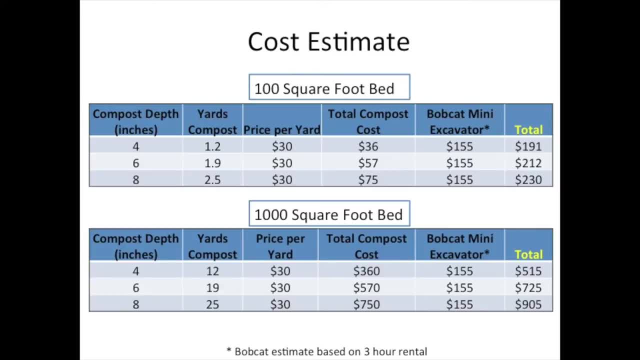 depending on your depth of compost you wanna apply. if we're talking about the six inch range, which would be fairly typical, that would take about just under two yards of compost. depending on your depth of compost you wanna apply. if we're talking about about the six inch range, which would be fairly typical, that would take about just under two yards of compost. 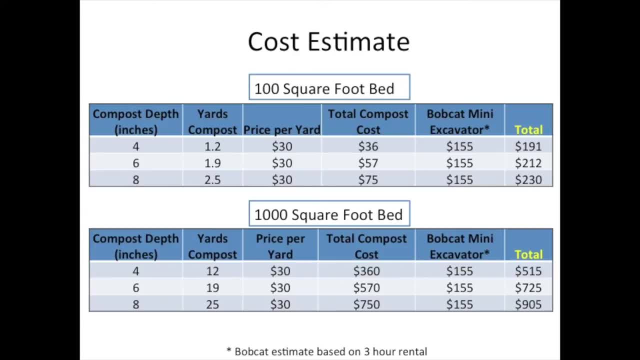 depending on your depth of compost you wanna apply, if we're talking about about the six inch range, and I estimated in this measurement for the Bobcat mini excavator to be rented for three hour period, So what we're talking about for a 100 square foot bed. 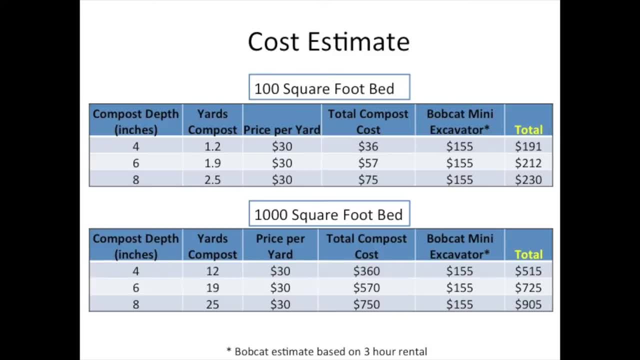 is about $212.. Scale that up to a 1000 square foot bed, which would be a fairly large size bed, but certainly something if you're planning a large installation, is for the six inch depth you're looking somewhere around $725.. 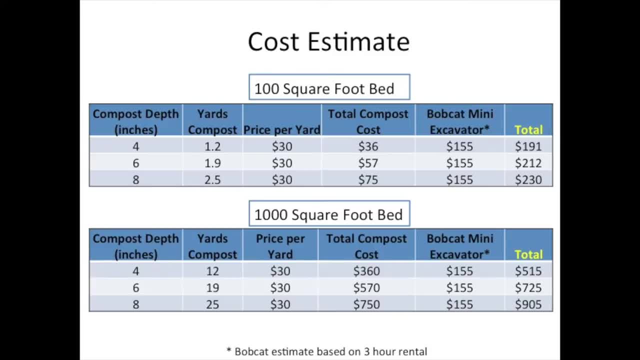 you're looking somewhere around $725.. Again, it's important to think about where your compost is coming from, what kind of source and how expensive you think that is going to be, as well as the machine use. But the one kind of point when we do think about costs that I want to bring up is just 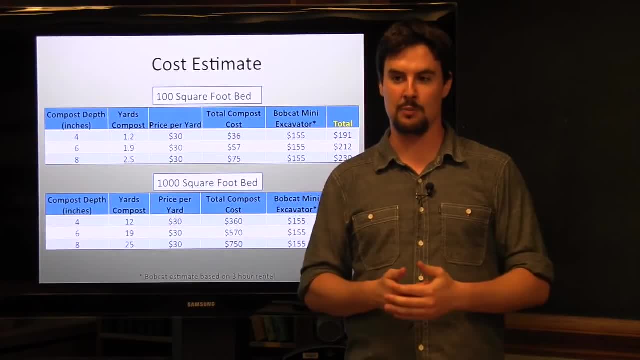 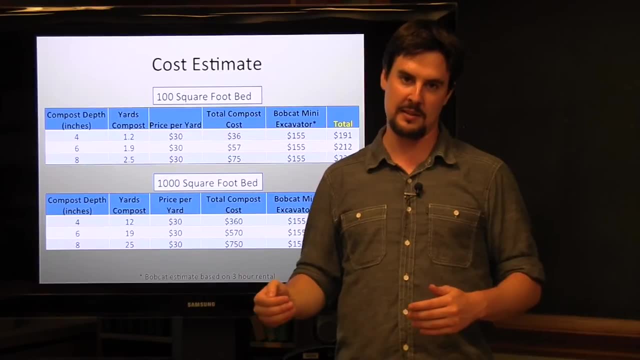 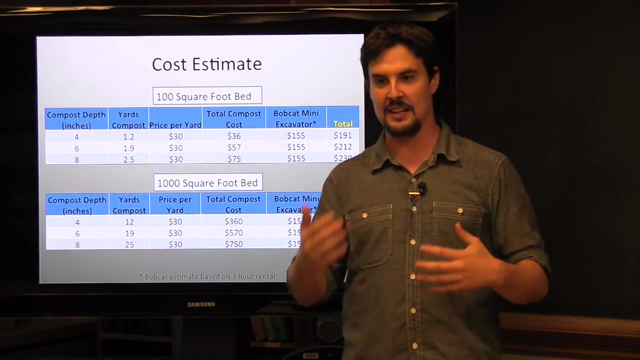 the idea that we know that this technique improves your soils over the long term. So you have to think about it more in terms of making an initial investment and then, over time, it's going to continue to pay off, And this is going to be particularly pronounced if you're working at a site that has had plant. 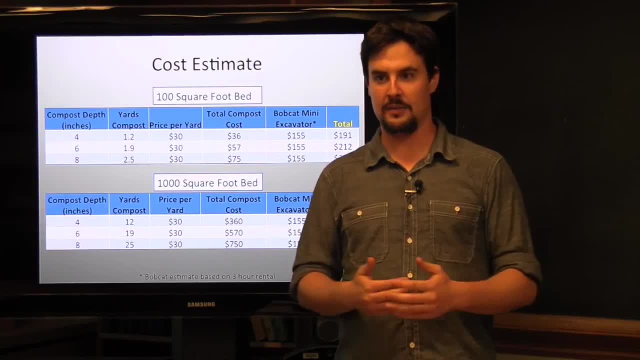 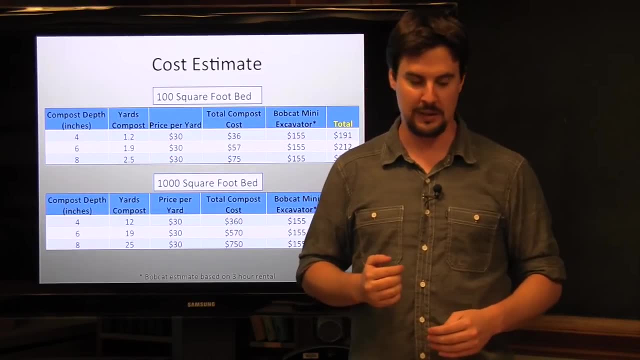 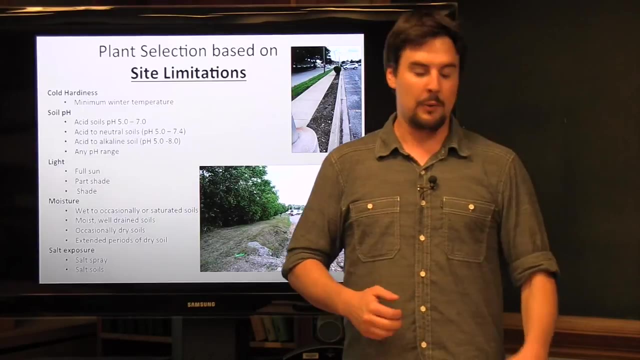 failure in the past. By using this technique, you're going to hopefully be able to decrease on plant failure and therefore be saving money by not having to replace those plants nearly so often- Or hopefully not at all- And when it does come to selecting plants to be putting in this bed, what we talk about. 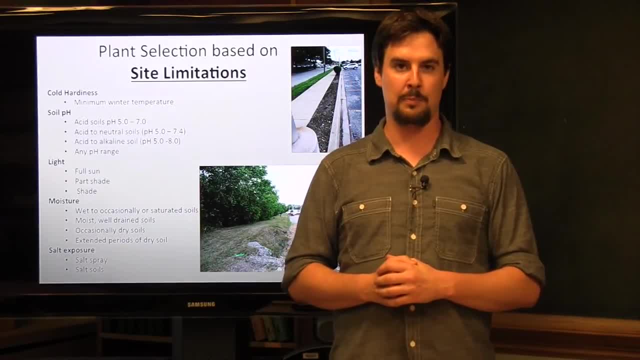 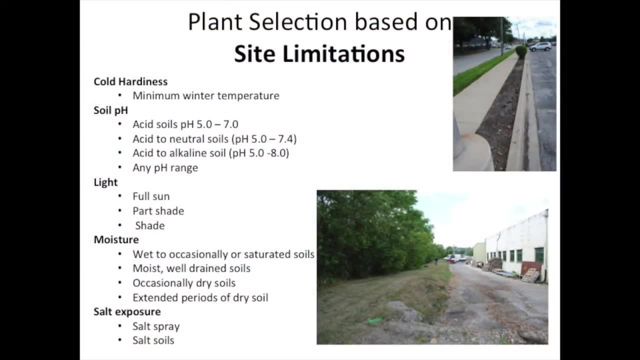 in the Urban Horticultural Institute is always selection. It's selecting your plants based on your site's limitation, And the Urban Horticultural Institute has a number of different resources available to help you figure out what your site limitations are, and I'm just going to talk about them. 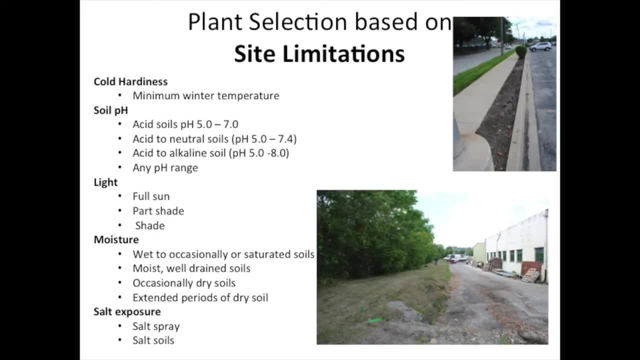 kind of briefly here. So the first one we oftentimes consider is to be cold hardiness, And most people are familiar with this. There's very good maps by the USDA which will tell you what zone you're in, and you always want to select your plant first. 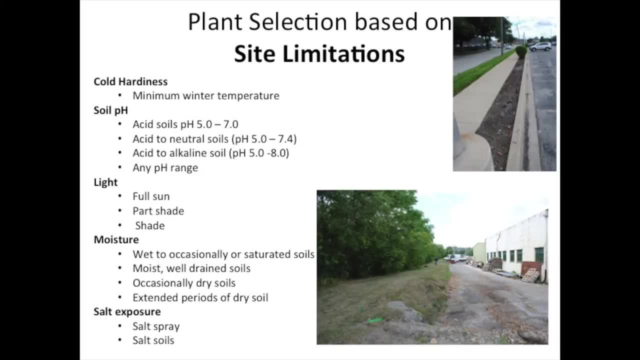 And based on zone, so you know that it can thrive on the minimum temperature that you find in your area. The next thing you consider is soil pH And you're either going to have- you could have- very acidic soils or very basic soils. 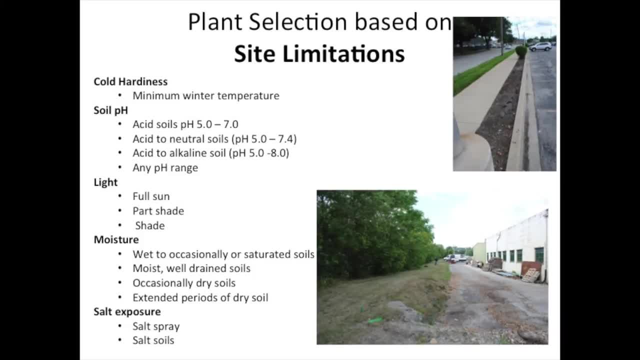 And based on this again, there's not much we can do except for select the right plants that are going to like that environment. You can make changes to soils, Soil pH, that is a possibility, But oftentimes when we think about in the urban setting, a cost that we do not tend, 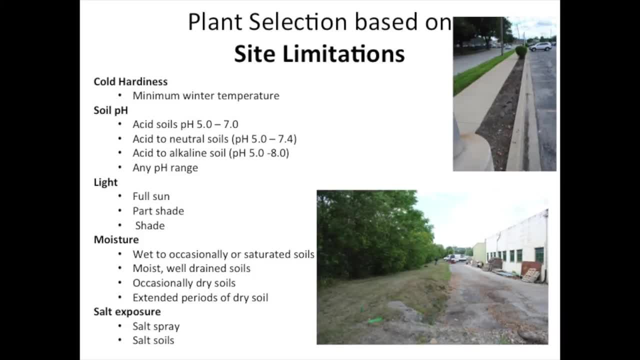 to incur because we don't actually tend to change the soils pH. It's easier to select a plant that can deal with the kind of pH range you're in, instead of going out and buying a lot of amendments. Light is the next indicator. You're either going to have full sun, which is six hours or more in a given day. 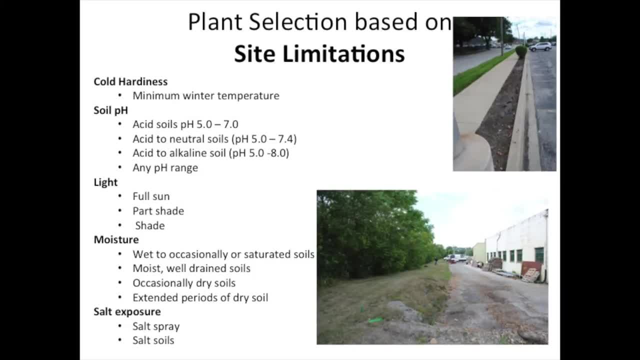 Dark shade, which is going to be less than that, or full shade, which is maybe at most an hour of light in the day. The next area that we consider is to be moisture, which is how much water is going to be at your site. 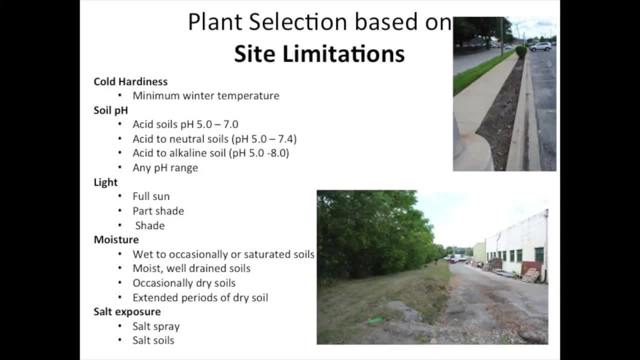 So whether you have a site that frequently floods or frequently drains very fast and actually stays very kind of dry, or if you're lucky enough to have something that can kind of do both, It will infiltrate water quickly but also hold onto it. 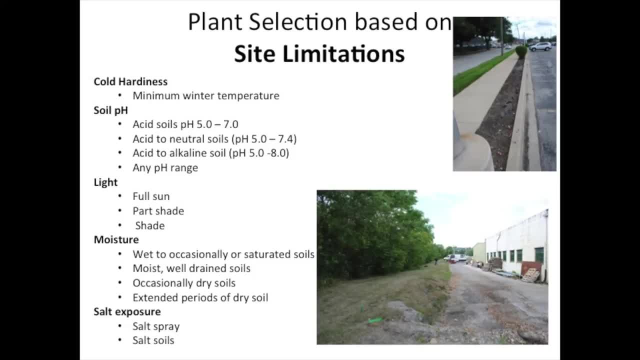 And as well as salt exposure, And this is something that we see particularly in a lot of institutional type settings or as well as in transportation type areas. We're either getting salt exposure from de-icing salts or salt soils if you're in a part of. 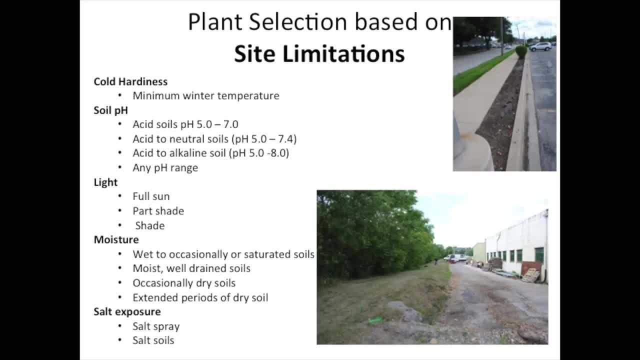 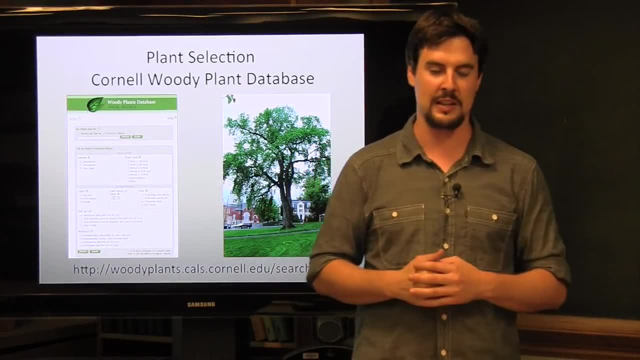 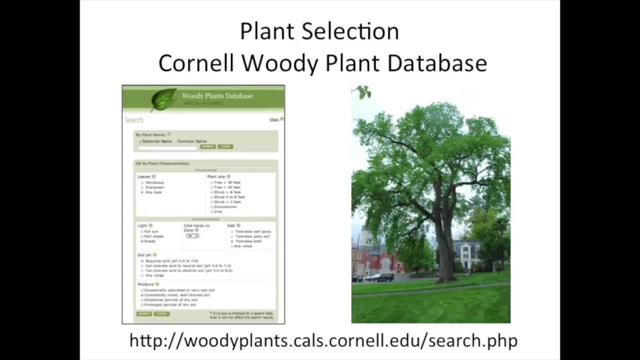 the country where salinity is an issue in your soils. So we have a great resource available to us. here at Cornell We've got the woody plant database. Okay, And what's great about the woody plant database is you can go onto it and figure out your 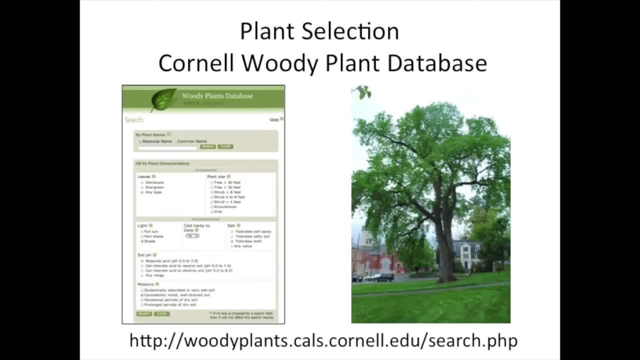 site's limitations, plug those into our database and what will happen is it will generate a list of plants that are appropriate for your environment. So I'm going to talk a little bit about some of these assessments. most of these assessments of site limitation you can do on your own in a pretty straightforward kind of a way. 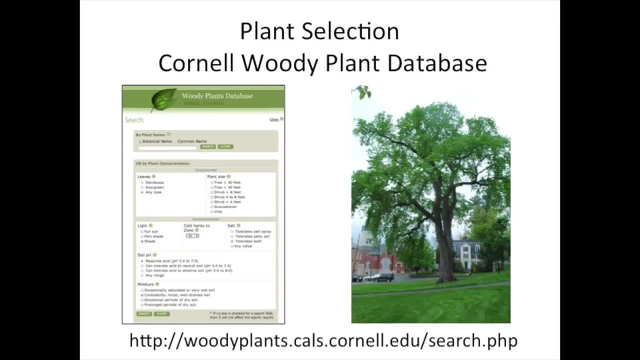 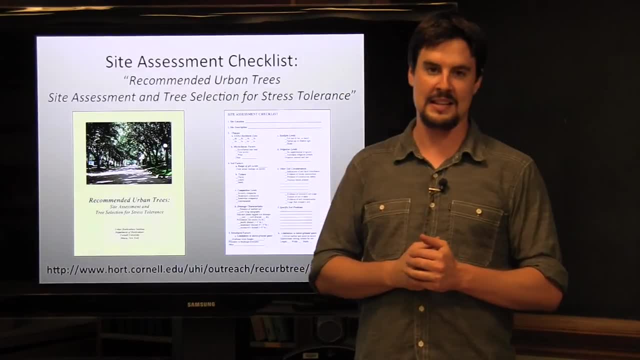 and then you can use the woody plant database to do that. Okay, So the woody plant database is a great resource that we use to find plants that are going to be, that are going to work for your landscape. Another resource available to people is the site assessment checklist. 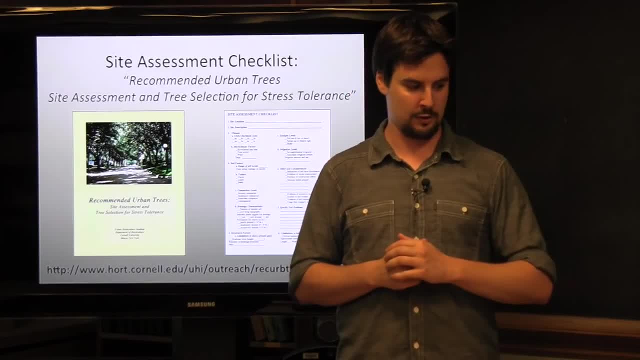 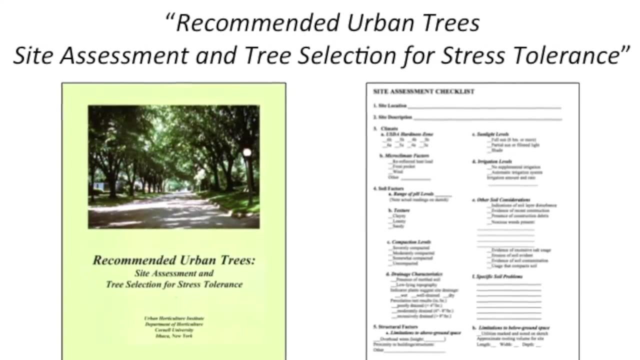 And this comes from a book written by the Urban Horticultural Institute which is recommended urban trees: site assessment and tree selection for stress tolerance. So similar to the database I was referring to a moment ago, and in this book it's free. 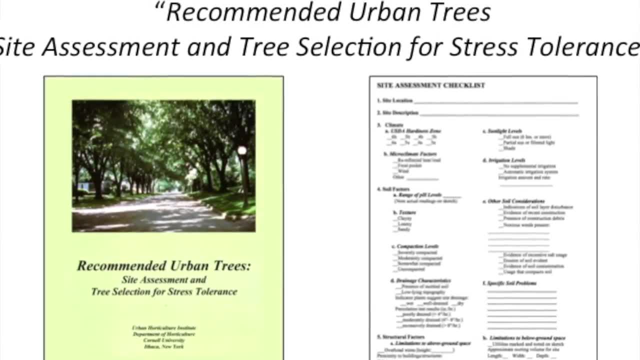 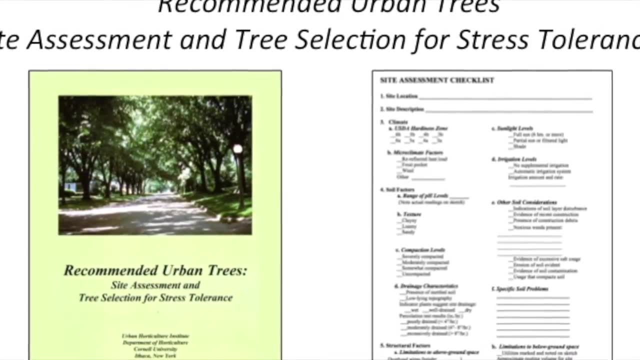 and available on our website online, But you can go through and they also have a checklist where you can actually go through each of your specific limitations and kind of check them off for a given site and then you can use that information to then select plants after that. 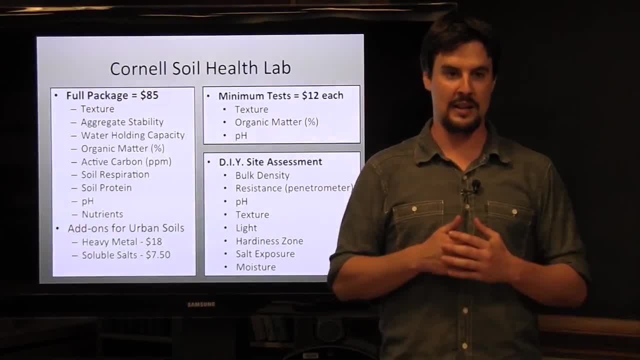 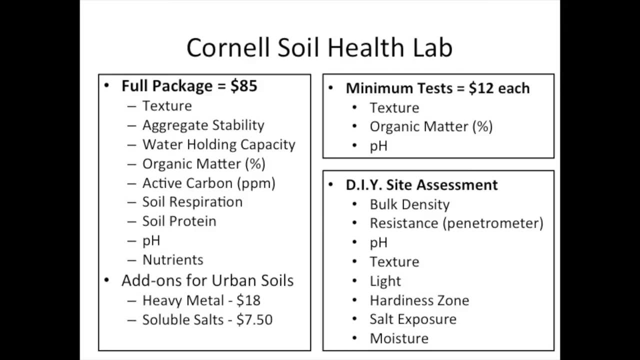 So, as I mentioned before, I've talked a lot about the concept of soil health, what it is. Cornell has a soil health testing lab so you can actually take soils and collect them and send them into the lab. Okay, So the soil health testing lab is a great tool to use for soil health testing and it's 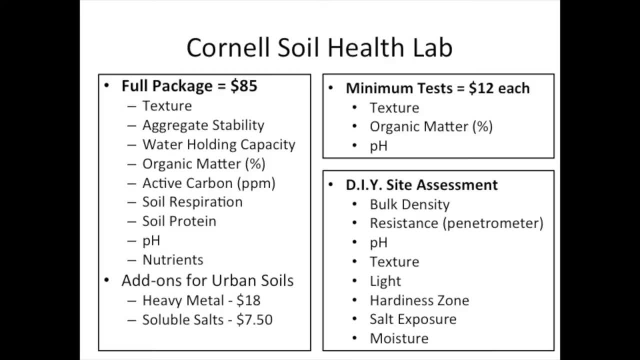 a great tool to use for soil health testing. It's a great tool to use for soil health testing. You can get a battery of tests, many of the ones I've talked about today, as well as some other ones that I haven't focused on as much. 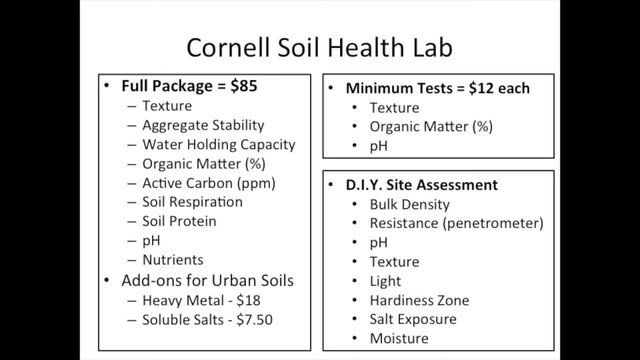 And for $85, you can get a full package where you get a really good picture of what's going on, And I would say that this is a great tool to use, specifically if you're doing a new management technique on a piece of land and you kind of want to see how your soils. 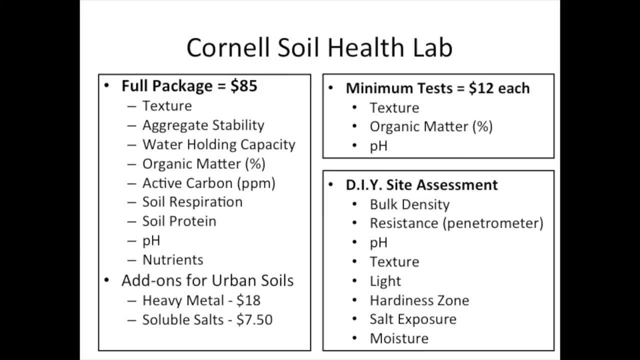 respond over time. Most soil testing it's always- you always want to do it when before you're about to establish a new site or if you're trying to understand what's going on with a site, specifically if you're having issues with some of your plant failure or you're just trying to get 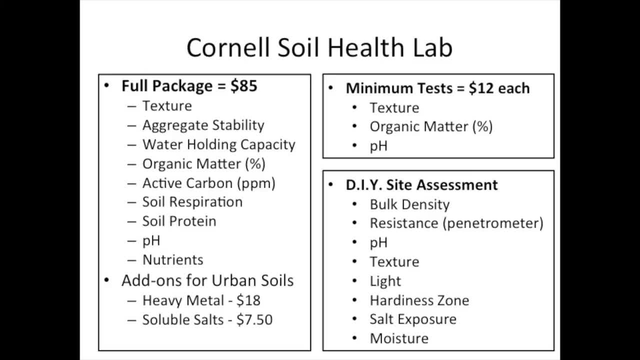 a better sense. But it's also something that's good to test over time, And that's what's really convenient about the soil health test is that it is responsive to management. So if you test one year, maybe two or three years down the line you can test again and 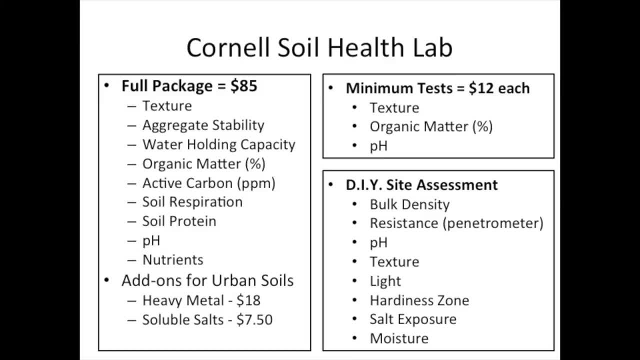 you can kind of see how your soils have changed in response to your management. There's a few add-ons. If you're concerned about heavy metals, You can add that onto the test, as well as soluble salts, if that is another concern for you as well. 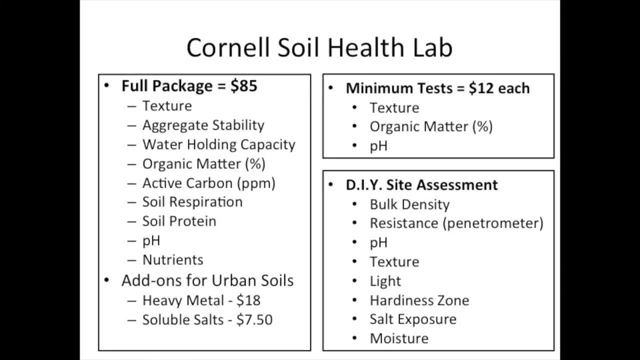 I would say, if you don't want to go and get the full package for $85, you can also send in and get what we call a cart or specific tests done. And I would say, if you're going to get a minimum set of tests, you should get your texture. 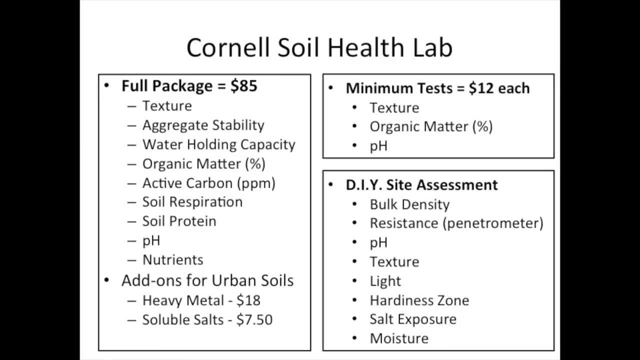 looked at. you should get your organic matter looked at and you should get your pH looked at, Since these are all, at least texture and pH is something that you're probably going to not be addressing in changing on your site, but will be very informative when you. 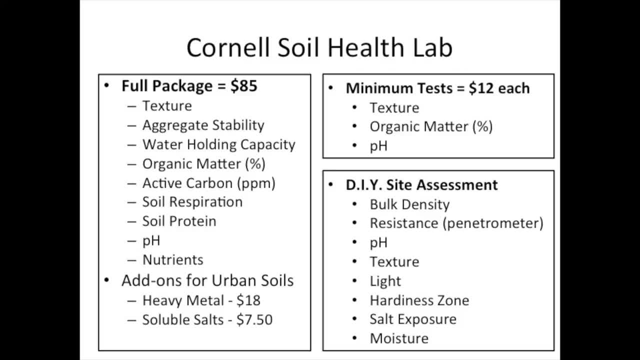 want to select plants for that landscape. And then there's actually a whole bunch of tests that you can do on your own, The do-it-yourself assessments, And these are bulk density, resistance with a penetrometer, pH, and then some of the site. 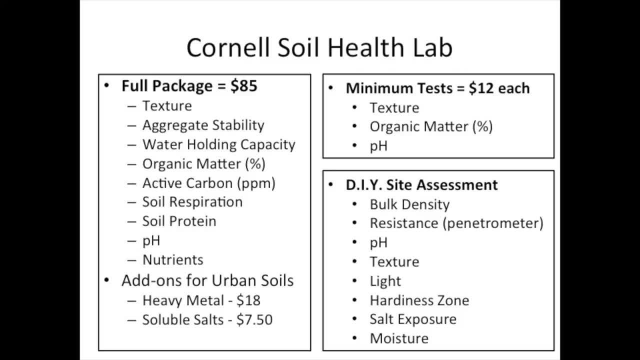 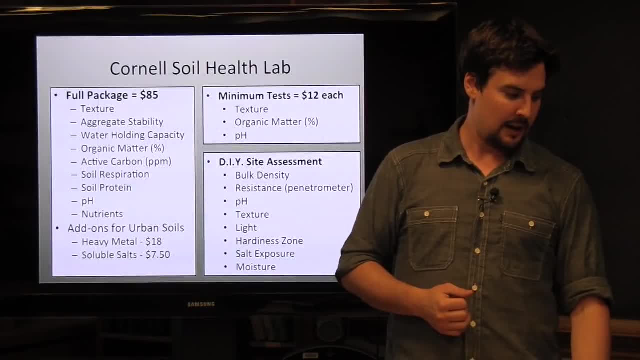 limitations, which I was discussing before. So texture, light, hardiness, soil, And then there's a whole bunch of tests that you can do on your own, the do-it-yourself assessments- Salt exposure and moisture. So I'm going to just talk about doing some of these assessments yourself. 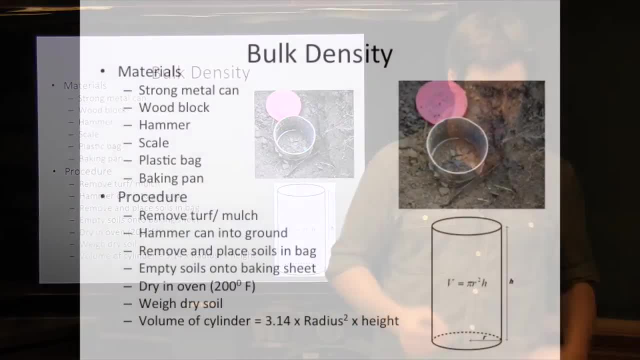 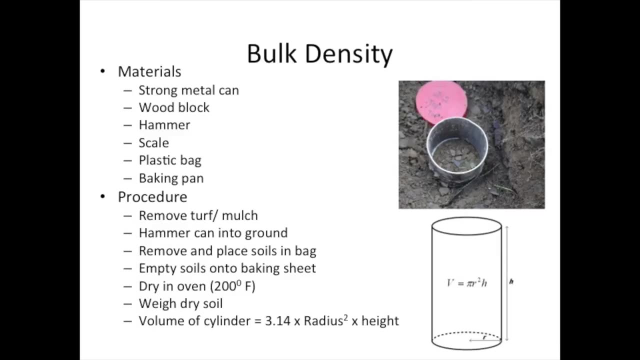 The first thing I'm going to talk about is specifically bulk density. Bulk density, as I've mentioned many times, is a measurement of weight by volume. If you're doing a lot of soil testing, it's wise to invest in a soil a can that you can. 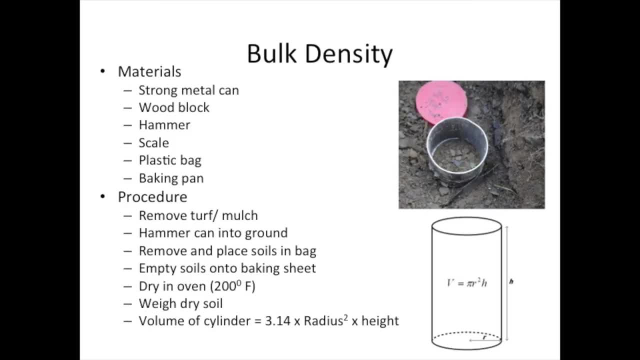 use specifically to test these, And it's a pretty straightforward process. If you don't want to buy one of these, you can also cut off two ends of a soup can anything that you know the specific size on, or you can measure and figure out the specific size. 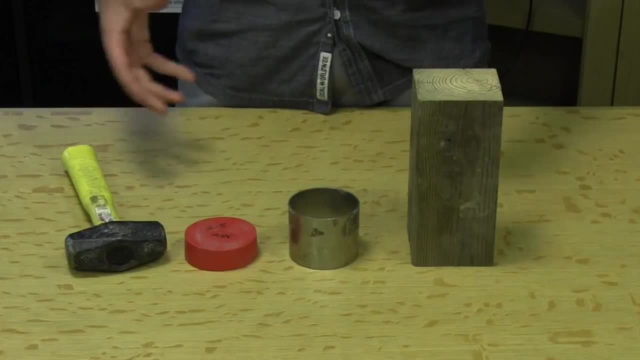 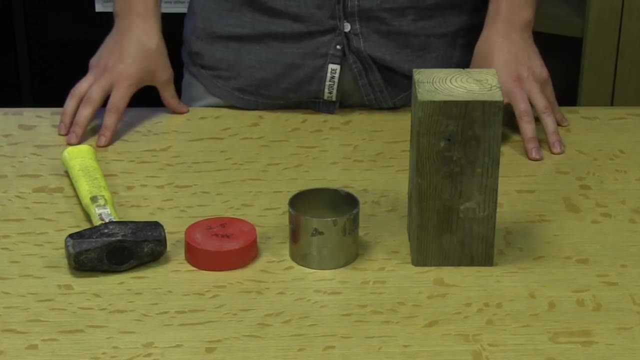 So what I want to show here, briefly touch on, is the actual technique of taking a bulk density measurement, And it's a pretty straightforward process. What you really need for it is just a few things: You need a wood block, You need a can. 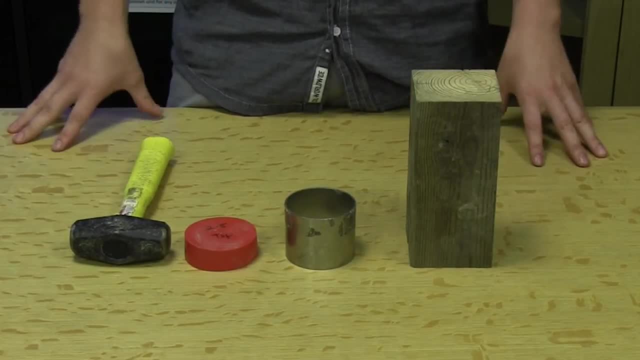 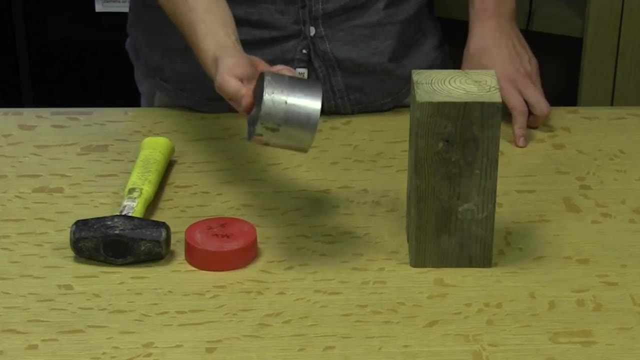 And you need a hammer. You need a hammer, as well as an oven at home and a cookie sheet, And this is a specific soil core that people who are doing a lot of soil sampling will use. If you don't want to purchase one of these, you're only doing maybe one or two sites. 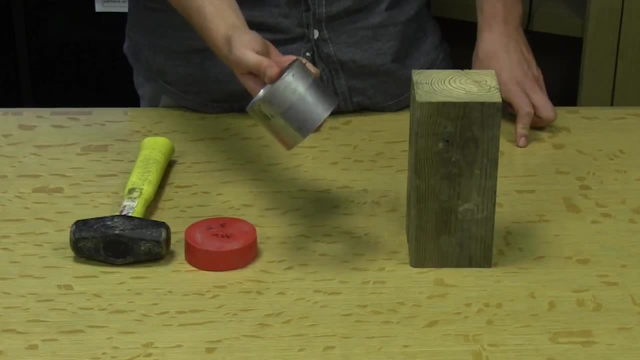 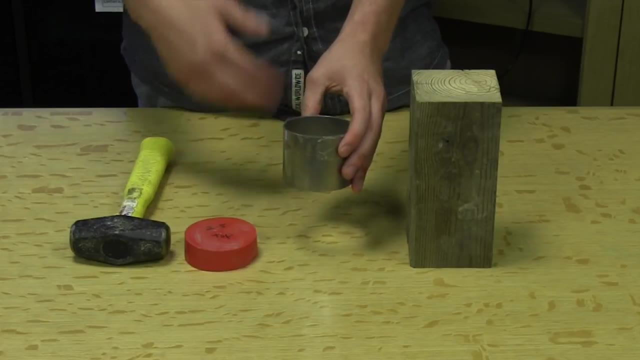 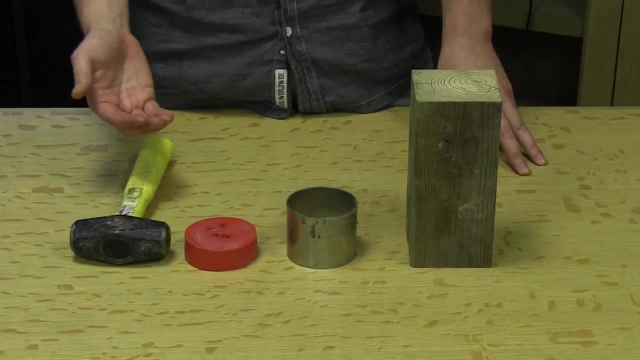 you can also use something like a soup can as well. You of course want to be careful not to cut yourself, But anything that you can measure the height as well as the diameter so you can calculate the volume afterwards. Bulk density is a specific measurement of weight by volume and therefore tells us our 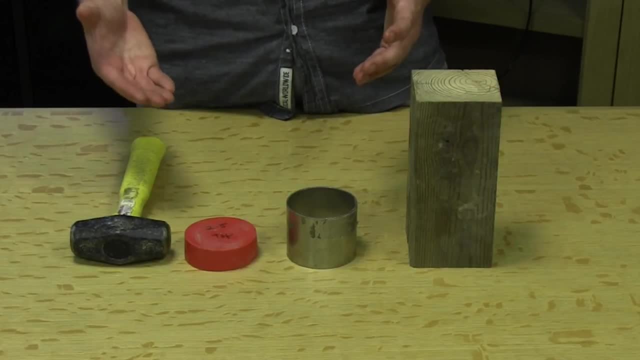 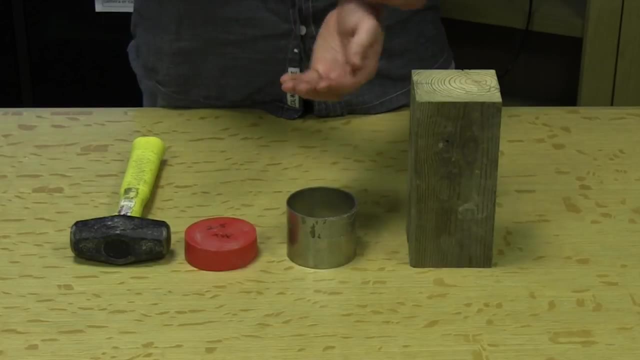 compaction in our soil. So the technique is pretty straightforward: We'll go out to a site and we'll, if it's turfed, what we'll do is we'll slice the turf layer off and then we'll come in and we'll take our core, put it on the soil, on the 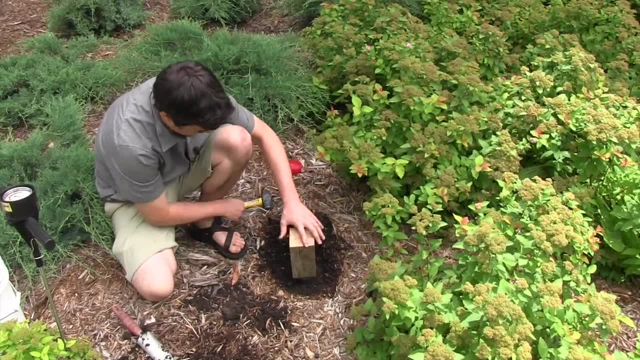 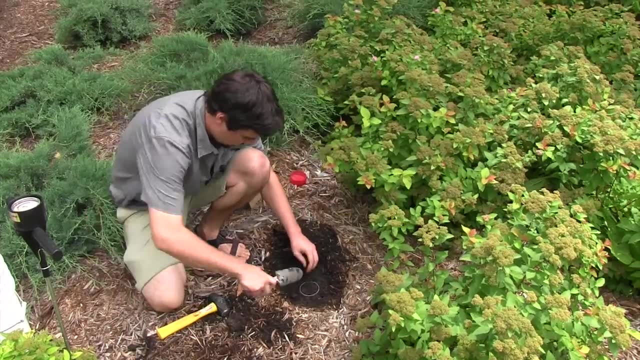 top of the soil, come in with our block and our hammer and hammer it down until you've got it Okay, And then your soil level just reaches the top of the can. At this point you can smooth it out, and then you're going to come in with a trowel, trowel. 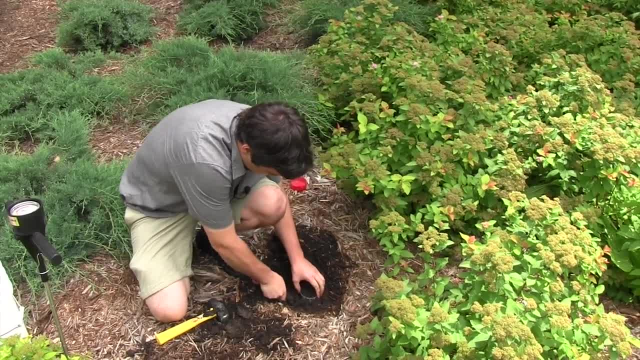 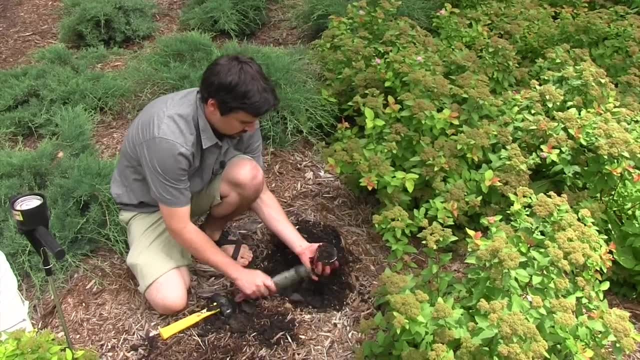 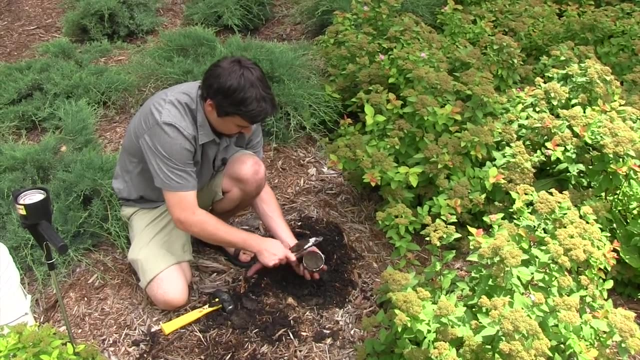 underneath it. It's good to get a cap, but if you don't want to get a cap, you can use anything that's flat. So cap one side of it, flip it over, smooth the soil out as well, And this way you know. now you have a known amount of volume of soil within this canister. 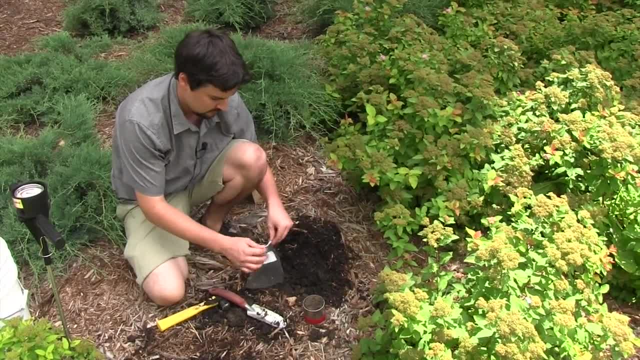 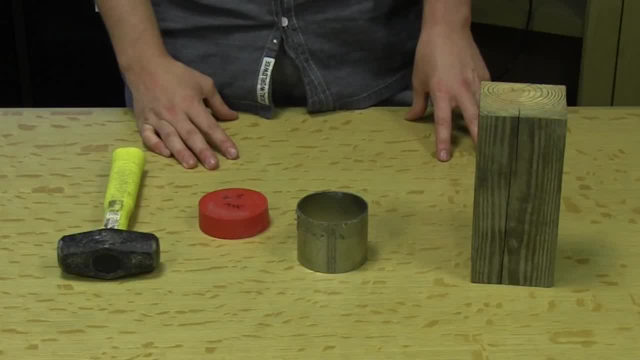 You can take this soil. Okay, Push it into a bag. You take that bag of soil, bring it home, put it on a cookie sheet, put it in your oven at 200 degrees for two or three hours until all the moisture has evaporated out. 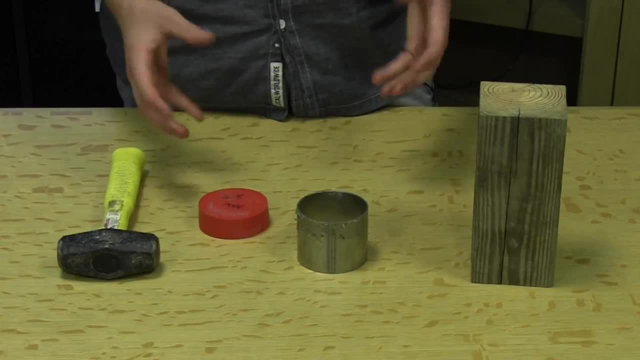 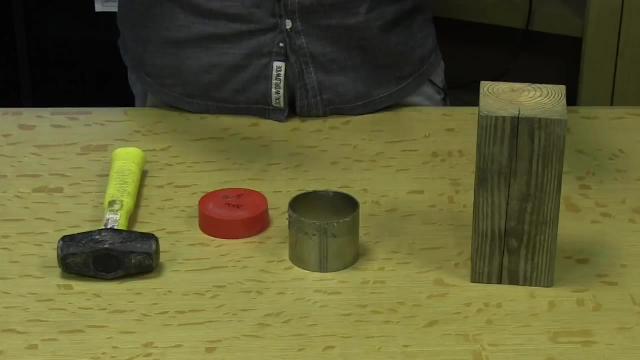 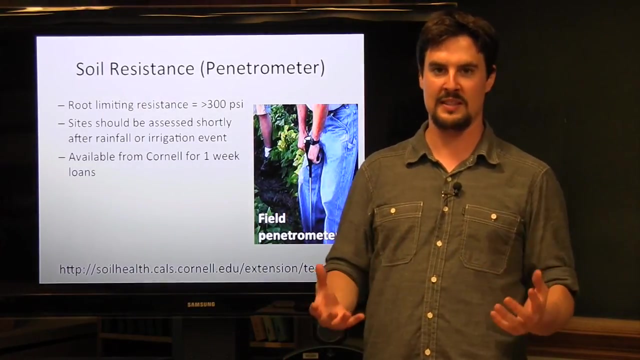 You can take that soil out, allow it to dry and then weigh it, And since you know the volume of your cylinder and the weight, you can then figure out your weight by volume and therefore you know your bulk density. Okay, So the next kind of do-it-yourself assessment is looking at soil resistance with a penetrometer. 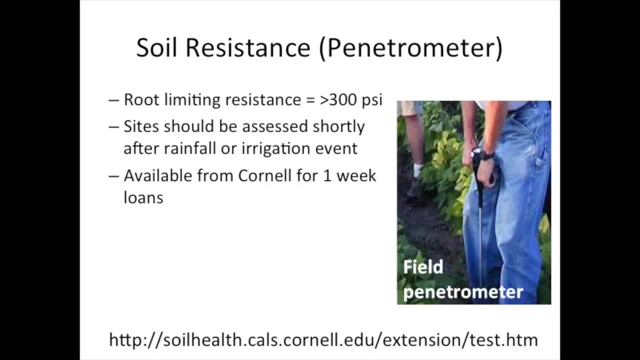 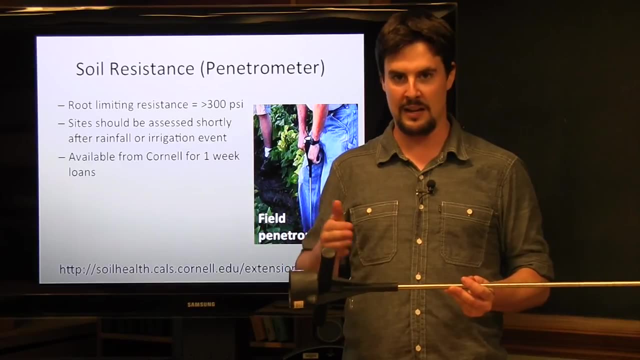 These are available from Cornell directly. You can borrow them for a week at a time where we'll ship them out to you, And you can get one of these penetrometers if you wanted to look at compaction across a lot of sites. And the main thing with these is that it's best to do it kind of after it's rained a. 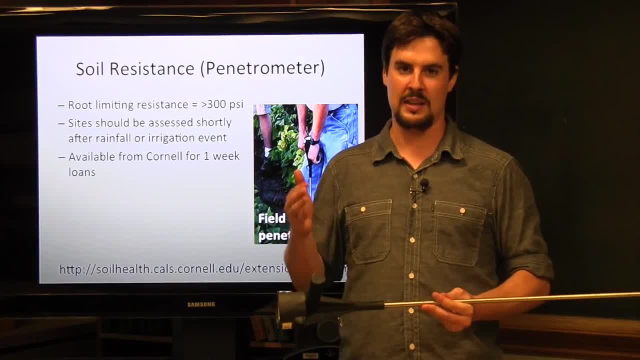 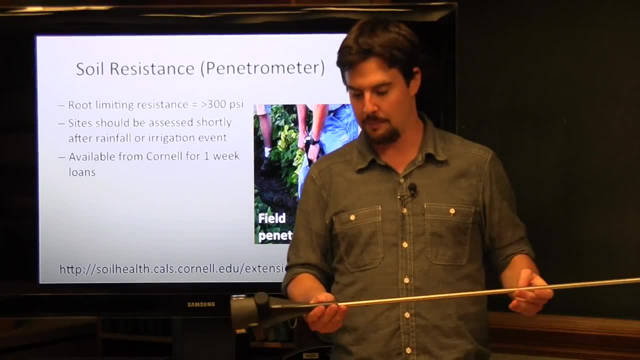 short period afterwards. But as long as you assess all your soils within a short timeframe so the soils don't dry out too much, you can get a pretty good relative indicator to each other. But, like I mentioned before, they're pretty straightforward in how they work. 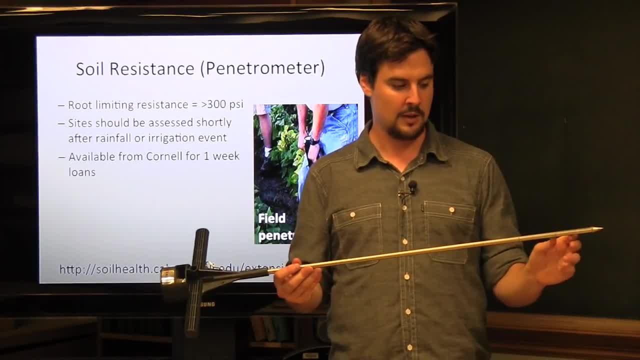 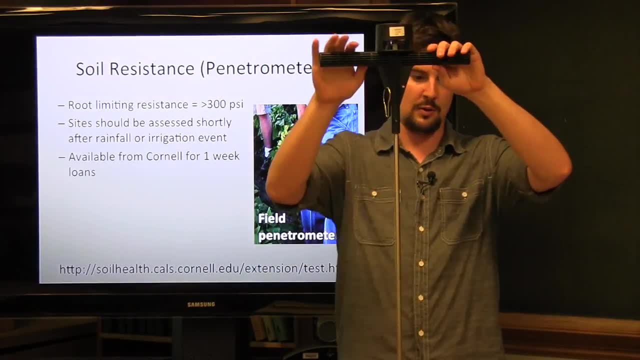 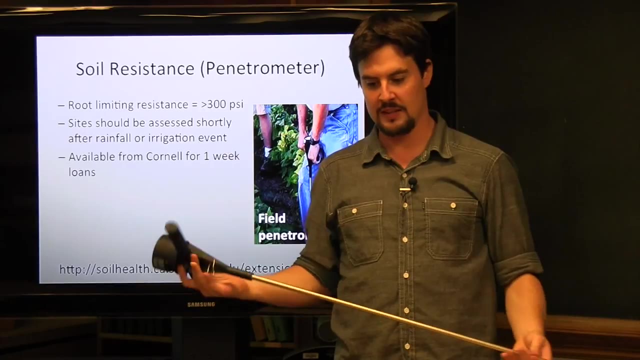 You've got a pressure gauge on one side and this is graduated, so there's actually measurements on this pole specifically, And as you push this down into the soil, what you're going to see on the top is increased pressure. The only caveat- other than moisture- on this is that there's two different tips you can. 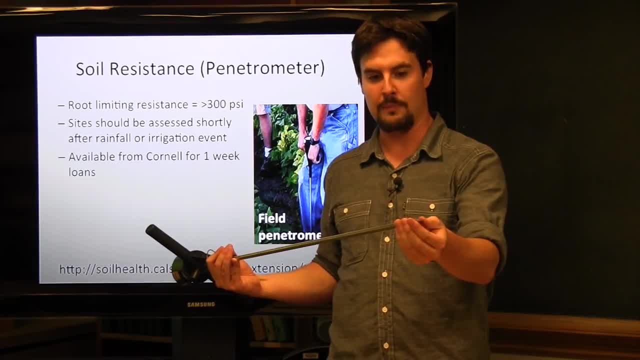 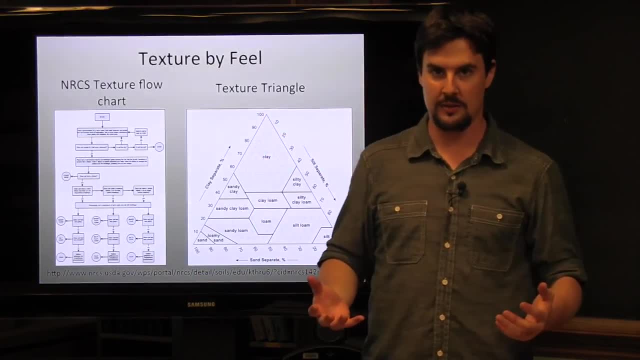 get. There's a 3⁄4-inch tip and a 1⁄2-inch tip And you only need to use the bigger one if you're working in very sandy soils. Next is texture: texture by feel. This is different than the way that if you sent soils into the lab, that they would look. 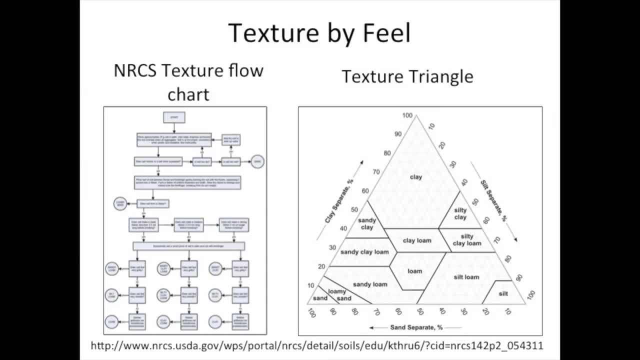 at texture. But there's a number of resources available that are just flowcharts, where you can collect a small amount of your soil with a little bit of water and you can go through the practice of assessing those soils And getting a texture simply by feel. 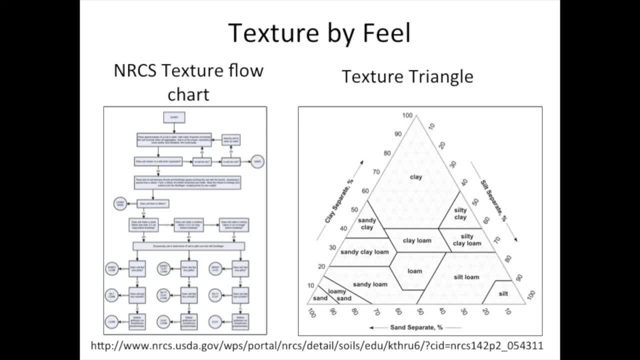 This is a common field assessment technique that a lot of farmers or land care practitioners or certainly soil scientists will develop so they can understand what the textures of their soil without going through the full test. So at the bottom of this slide there's also a link available where you can find a texture. 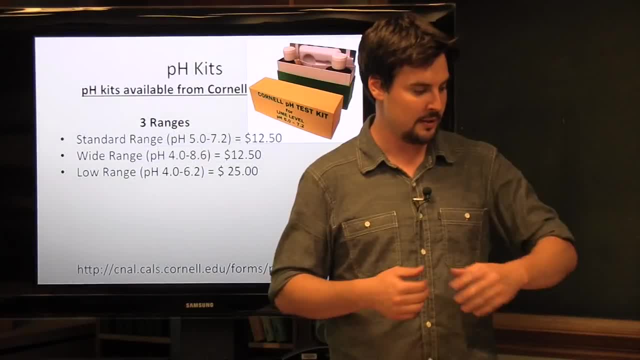 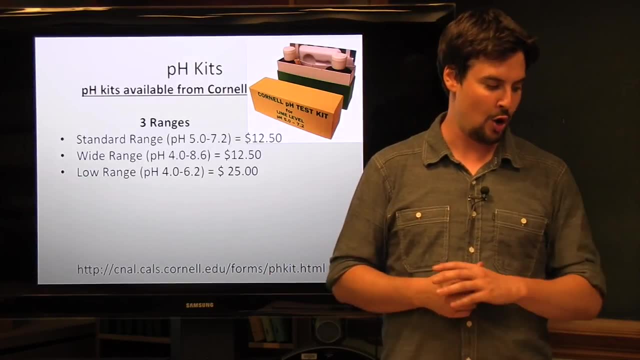 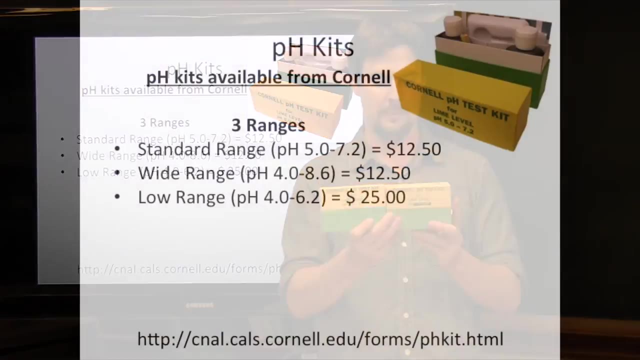 by feel, But there are a few out there. The next one that you can look at is pH. pH is another Indicator that is very easy to assess on your own. At Cornell we sell pH testing kits. They come in two different ranges. 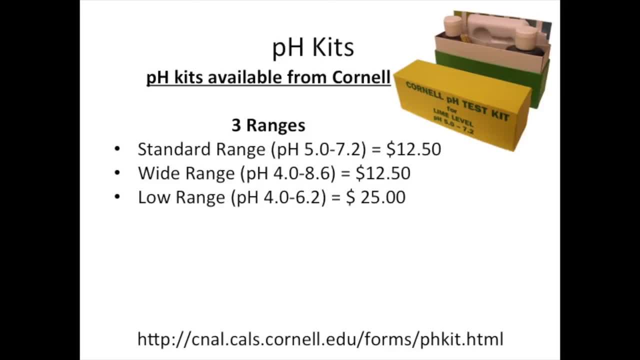 They come in a wide range as well as a standard range, Your standard range being from pH of 5 to 7.2. And your wider range being from 4 to 8.6.. And then we also offer one that's in the low range. 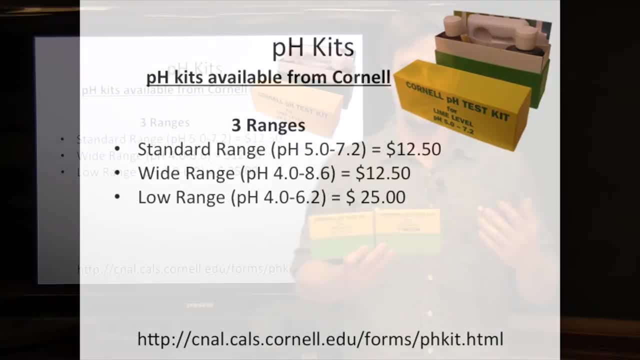 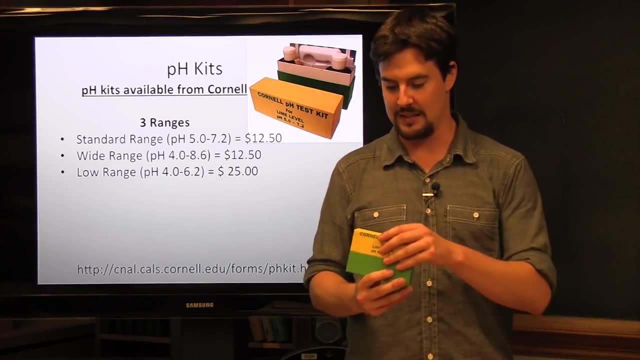 Which is from 4 to 6.2 pH. So you can buy a single one of these boxes for $12.50.. It will last you a very long time. It's a pretty straightforward process of taking a small amount of soil, placing it into these. 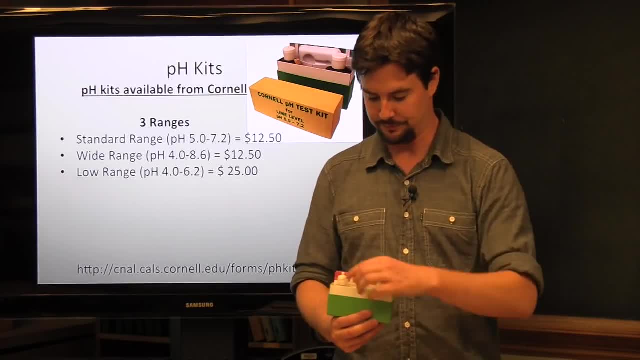 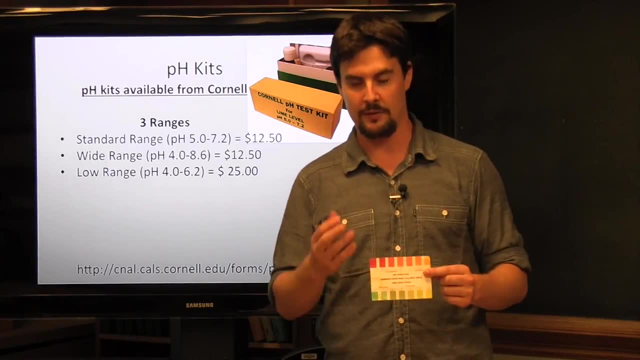 dishes and then using the different reagents and a color metric scheme to be able to tell what your range is in. So, particularly if you want to do a lot of sites across your campus, you could buy one of these kits for $12.50.. And you'll be able to do a lot of assessments. You compare this to the cost of doing the pH test on its own if you send it to the lab, Which is $12 for one test. So if you think you're going to be doing, even testing, more than one site, it's worth it. 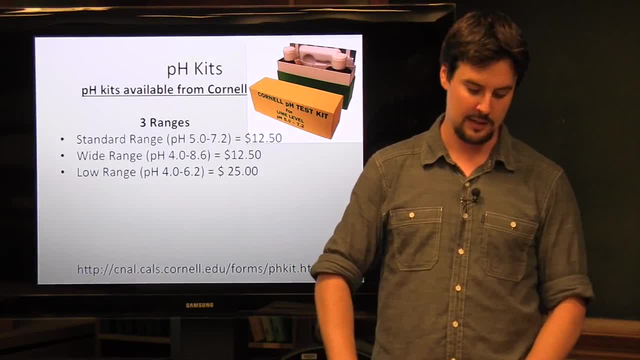 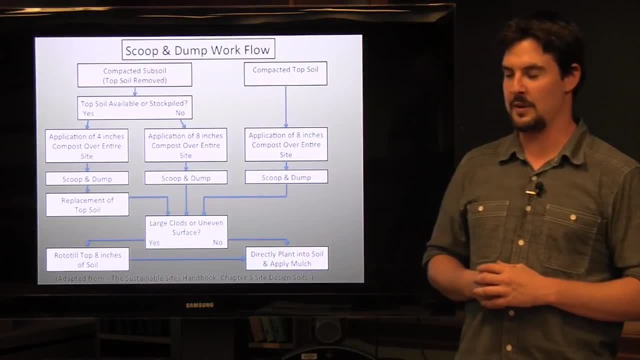 to invest within the pH kit, And you can also follow the links on this PowerPoint to get more information. There's a few extra slides here that are just at the end of the presentation. The first that I want to share with people is a general workflow. 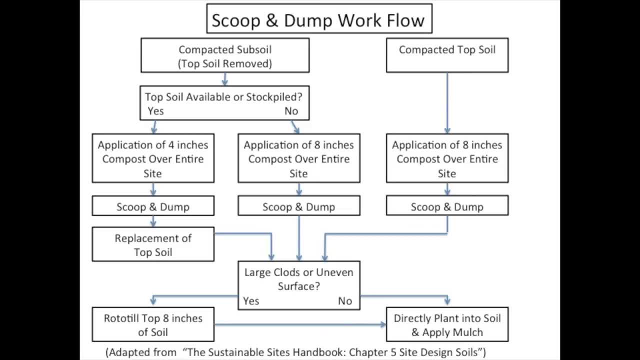 Of what you might want to be thinking about if you want to implement the scoop and dump technique And the first consideration you want to think about is whether you have a site that is just topsoil is present and it's just compacted or impacted. 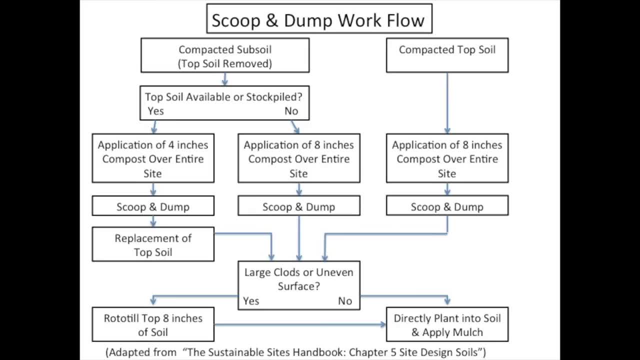 You can follow this workflow and determine the best, how much compost to apply and at what stage. You can also use this technique if you are on a construction site, where you strip the topsoil and have it stockpiled somewhere And you want to be able to do a lot of testing.